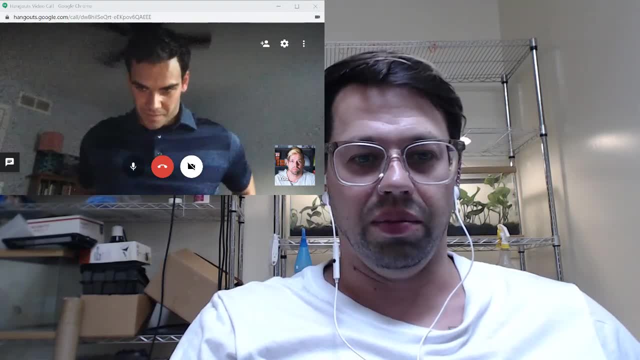 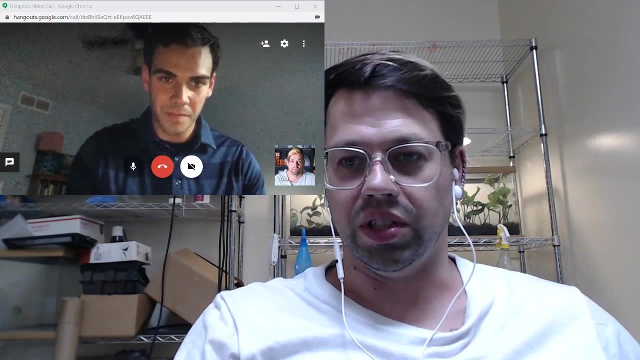 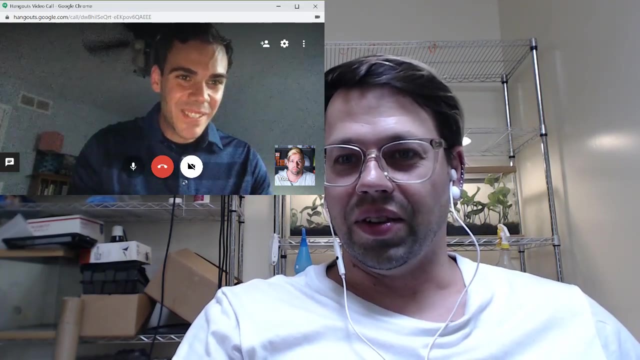 patched in so we're both live right now. um, i don't know if it's working very well. can you guys see justin moving at all or no justin? can you see justin moving at all? all right, well then, just uh chat. answer questions in the chat. we'll just get started. 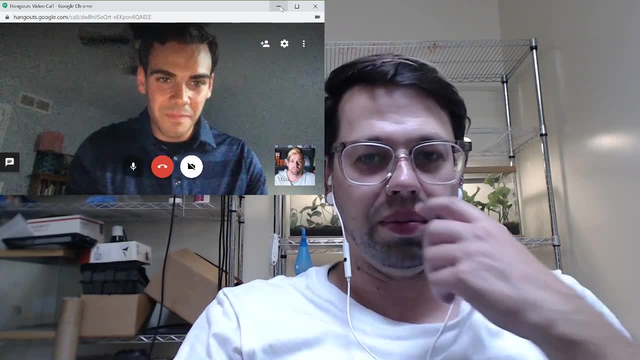 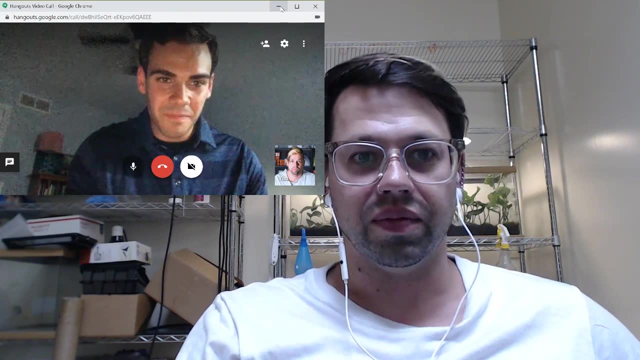 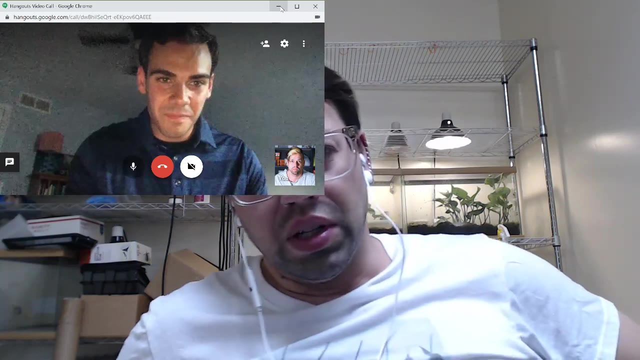 justin, you help answer questions. if that people have in the chat and stuff like that sound good, all right, okay, so bioengineering 101. if you go to the google classroom, um, we have the syllabus. we're going to go over the syllabus and then we're going to go over the syllabus and then 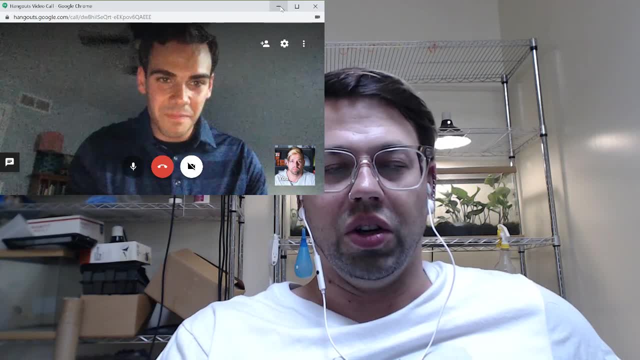 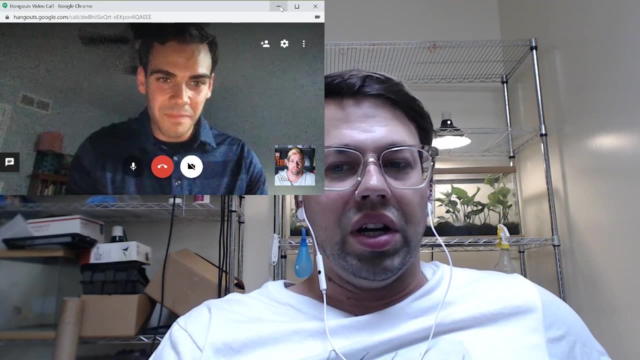 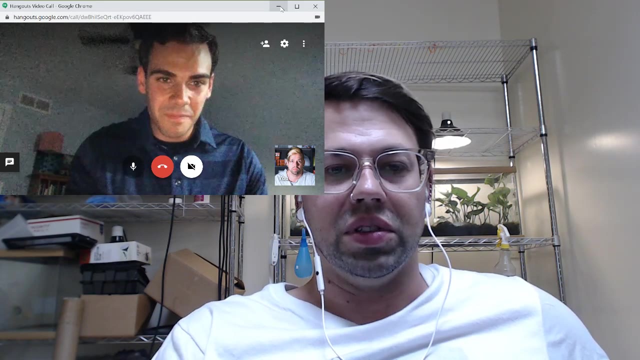 we're going to go over the syllabus really quick and just get everything going. so all the videos for this class are recorded and they can be found on the odin youtube channel. so please go to the odin youtube channel if you miss a class. um, it's just youtubecom. slash the odin inc and you should. 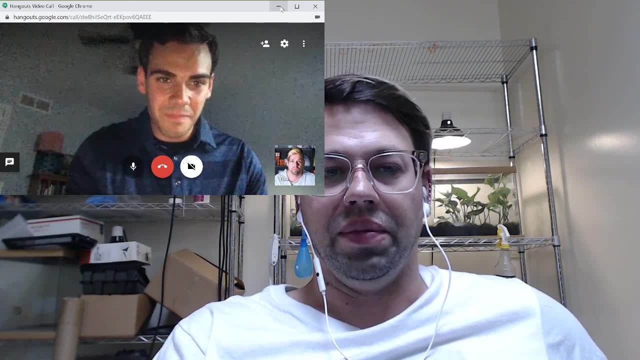 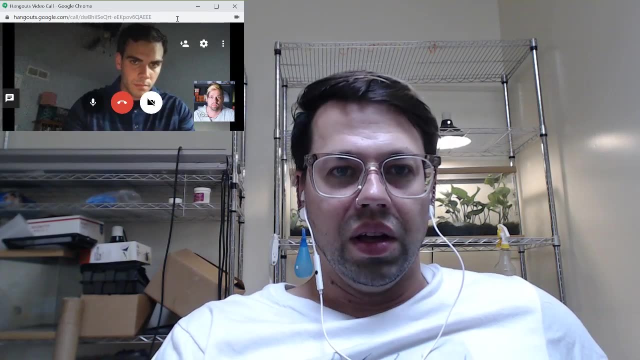 be able to watch any video that, uh, you missed out on, so don't worry about that too much. if you can't find it on the odin youtube channel, you can find it on the odin youtube channel. you can't make every class and you miss a video. um, this course is no experience required. we're going. 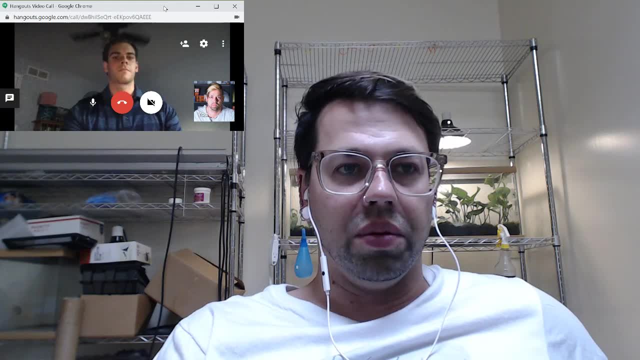 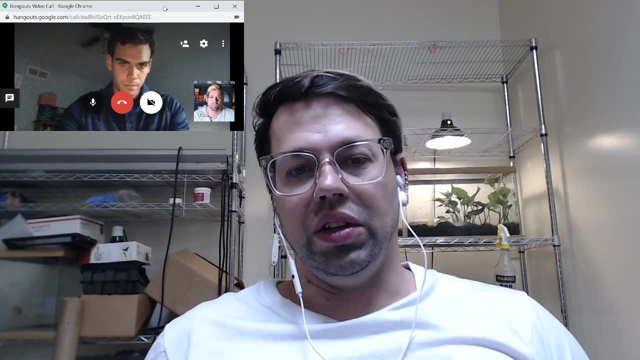 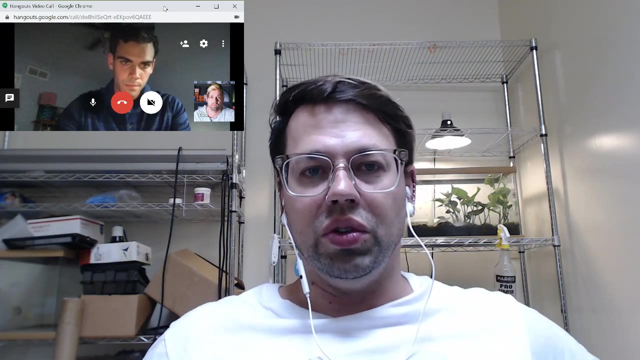 to teach you everything you need to know, so don't worry about that stuff too much. we're going to tell you about- uh, you know everything from what dna is, how to use all the equipment that you received in the kit and basically get you to the place where you can do genetic engineering. 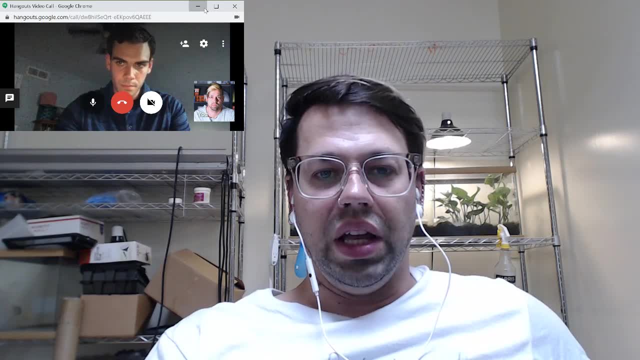 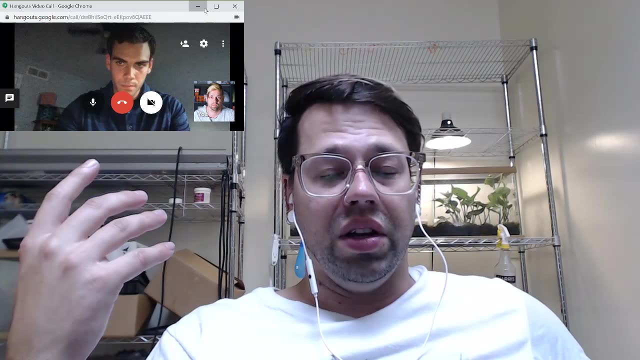 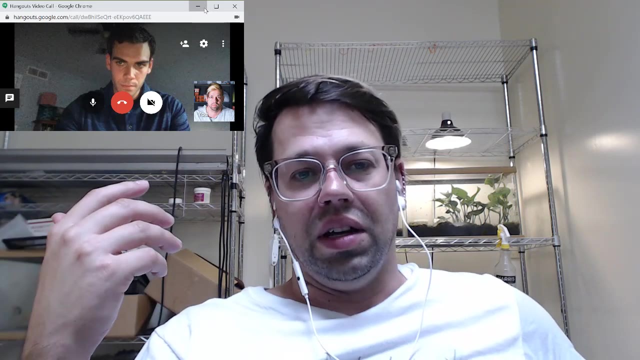 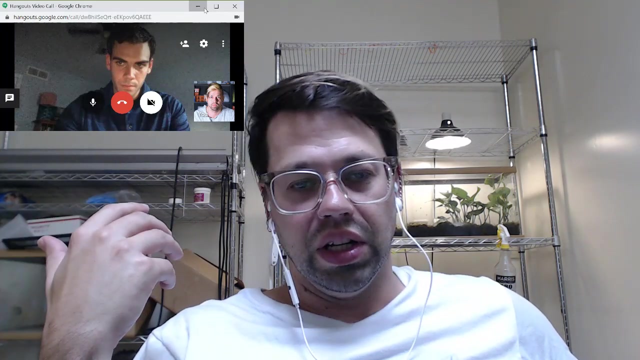 by yourself, without any uh outside help from anybody else. um, some of the uh goals and things we're going to do in this course is: um how to use pipettes, how to make agar plates, how to use sterile technique, culture bacteria, genetically modify bacteria and even go over crisper and things like that. 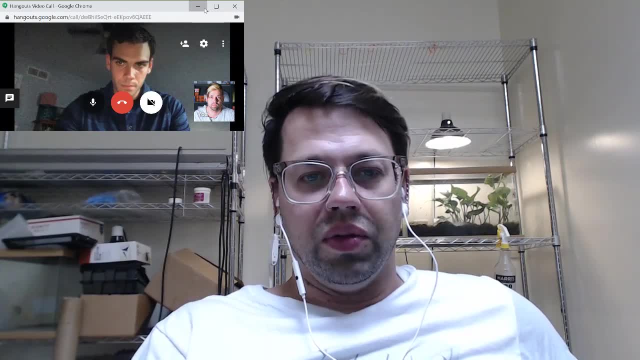 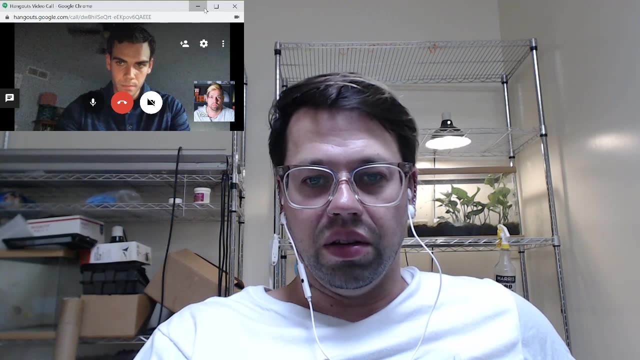 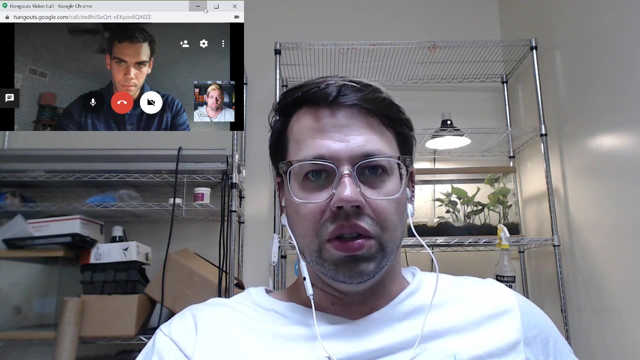 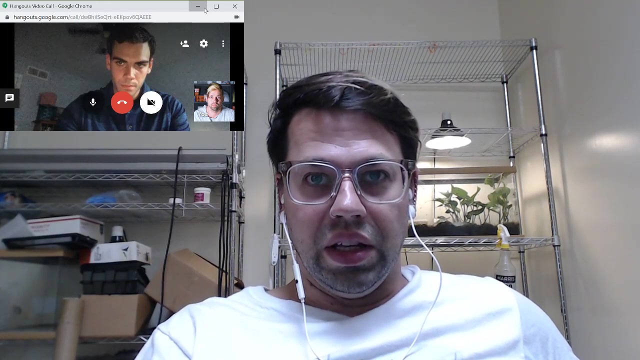 so the textbook for this is molecular biology of the cell. there should be a copy of molecular biology of the cell um in the google classroom under week one, so just go and download that from the link and, uh, follow along. so at the end of the syllabus. 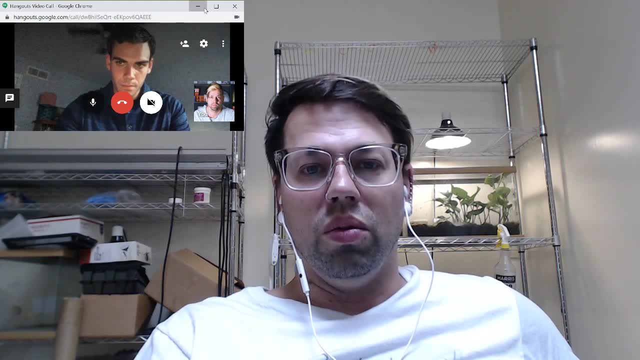 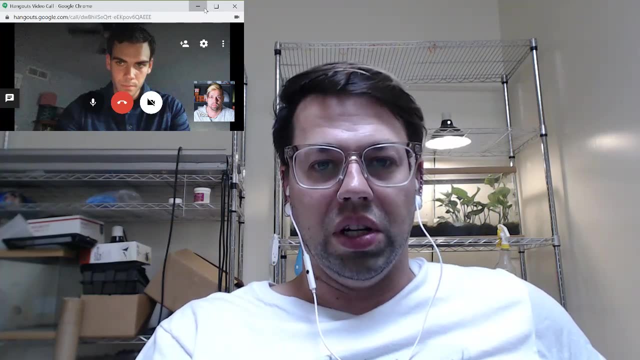 it tells you what weeks we're going to cover what chapters of molecular biology of the cell. so week one and two we're going to cover chapter one and chapter two, right? so check that out, try to keep up to date with that. there's going to be a lot of reading. 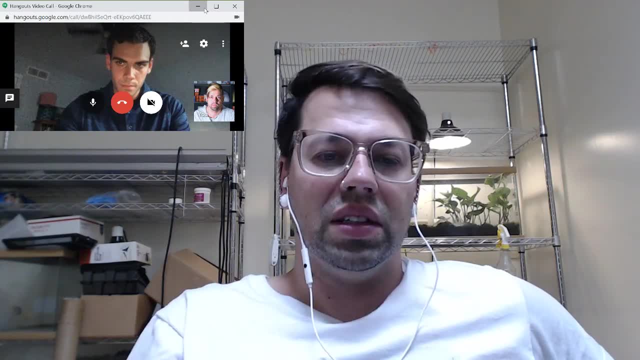 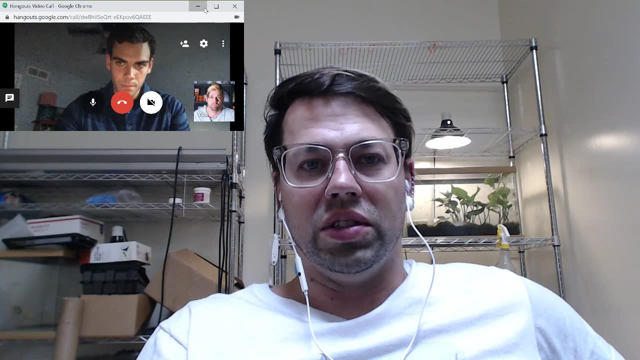 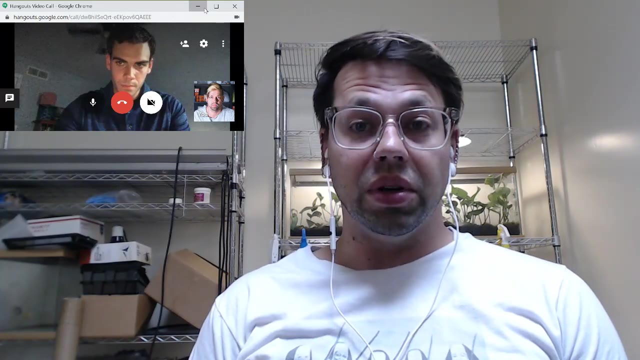 and a lot of work and stuff with this class, but you know, try to do the best you can. um, you know i i understand that you might not be able to, uh, get all the reading done. it's a, it's a lot of reading, but just do the best you can. right, because it's the class is just going to be. 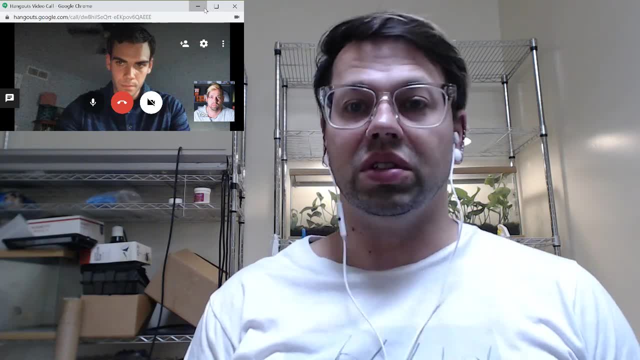 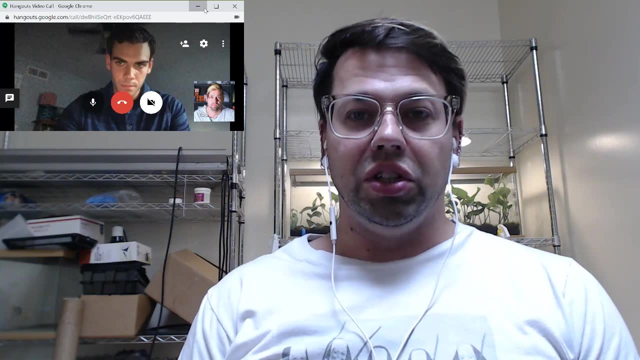 about subjecting yourself to this information and it's going to be a lot of reading and it's going to be a lot of information over and over and over again, right, like that's how you learn. somebody tells you about biology and certain things and you just keep hearing it and you 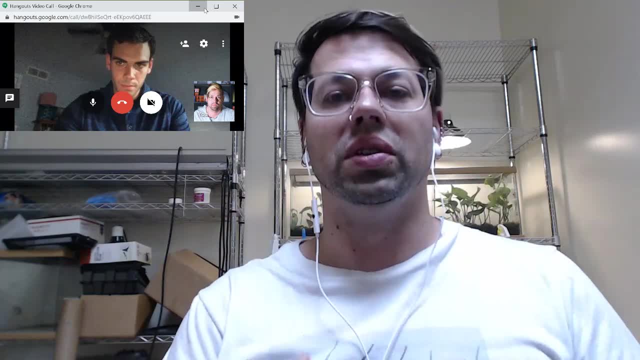 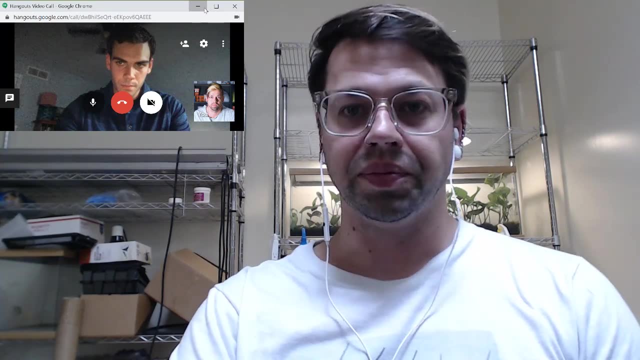 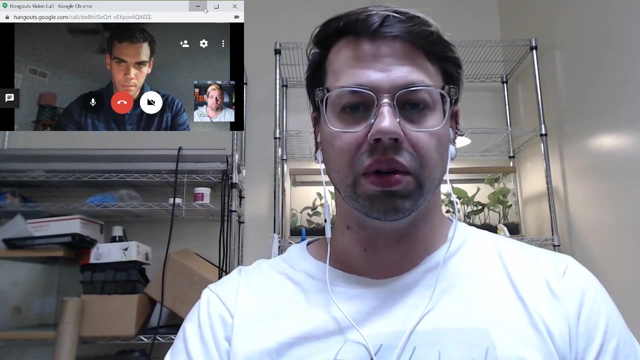 keep reading it and you keep learning it and the information just builds and builds and builds up. that's the way you're going to learn how to do all this stuff in the class. so, yeah, do your best, you the best you can, with the readings. so there's two programs that we're going to use and go over in this class. 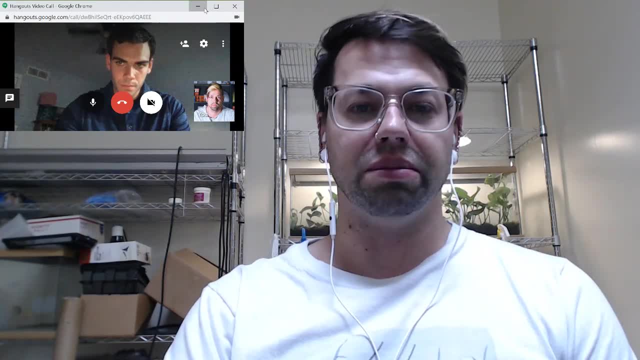 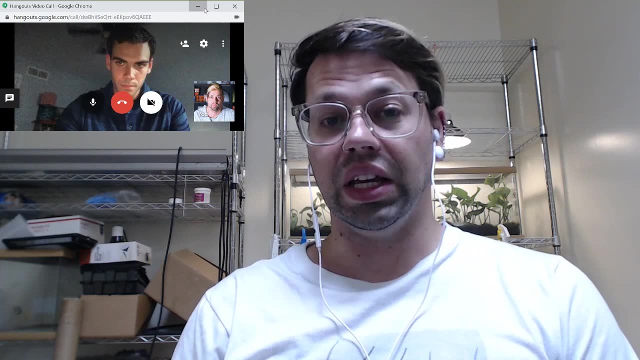 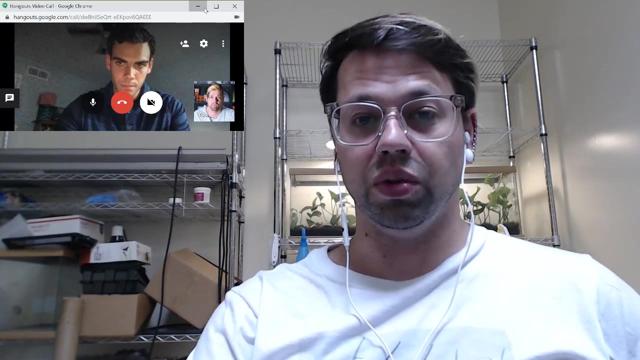 one is snap gene, so get the snap gene viewer, it's free. it helps you look at dna. we're going to go over that um: how to look at dna and analyze dna and stuff like that. the other is vmd. it's a visual molecular dynamics i think it stands for. it allows you to look at proteins. look at the. 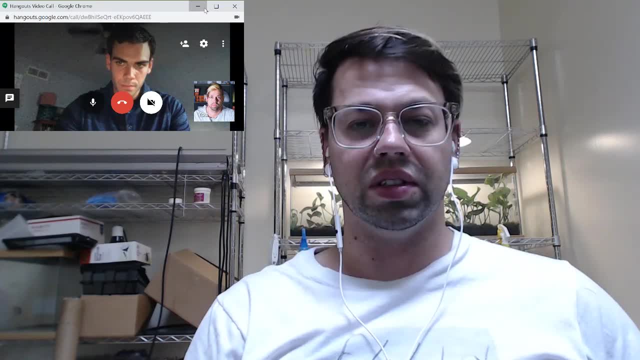 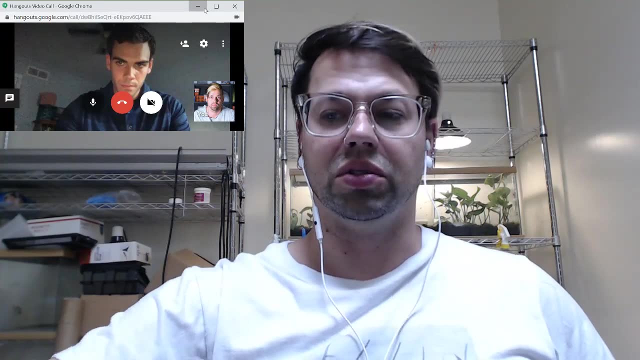 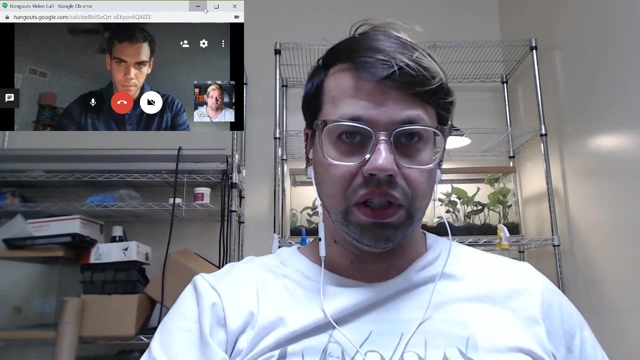 three-dimensional structure of proteins and all that good stuff, um, because, uh, it's an important part of molecular biology, biochemistry, genetic engineering type stuff, um. so each week the first thing you should do is go to the readme. the readme will have the information for the week, for the class. 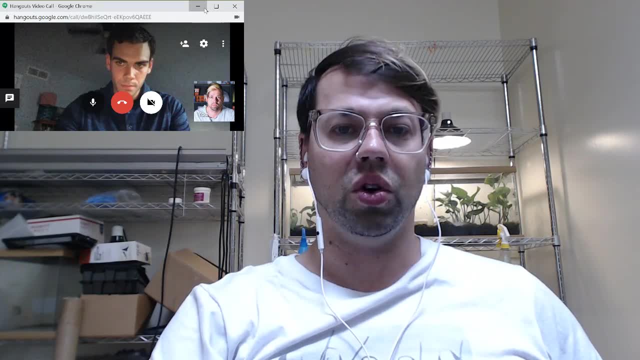 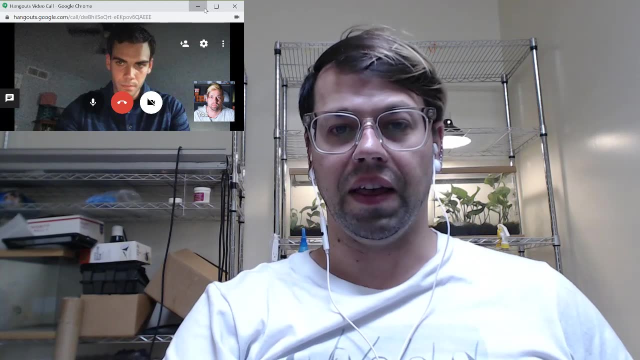 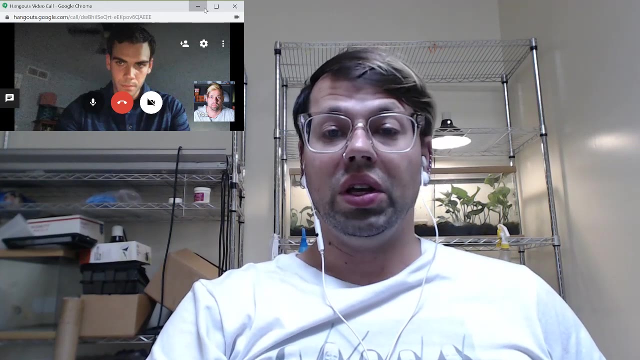 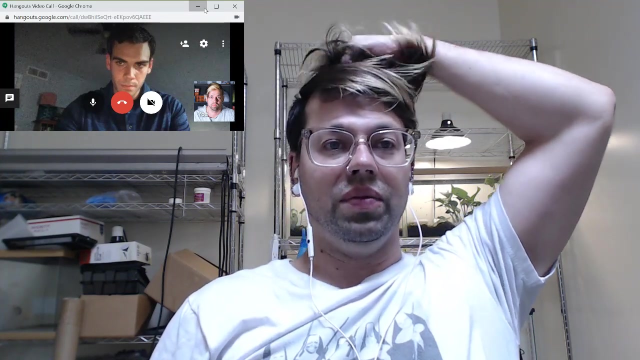 what things. you're going to kind of go over what papers you can try and read. you know the papers obviously reading are optional and some of the things you will learn this week. so this week being week one, we're going to start out um learning how to use a pipette and how to use a scale. 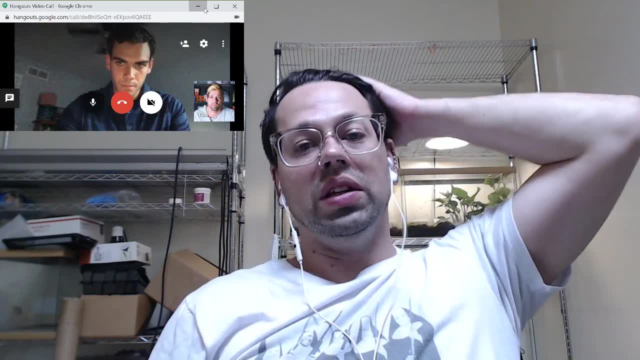 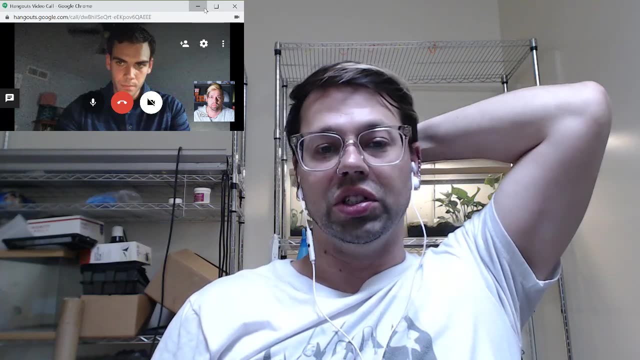 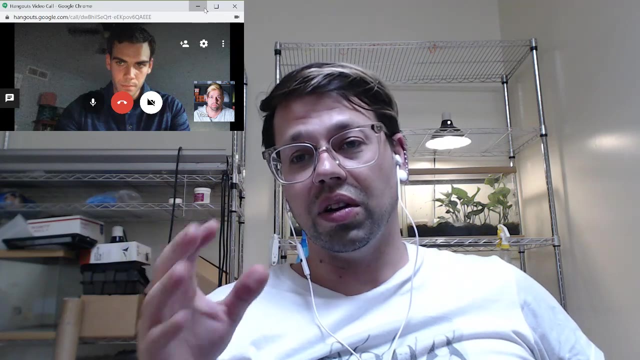 so that'll be the experiments for this week. these things are the building blocks of doing hands-on molecular biology and genetic engineering if you don't know how to do these things, even if you kind of think you know how to do these things but aren't completely. 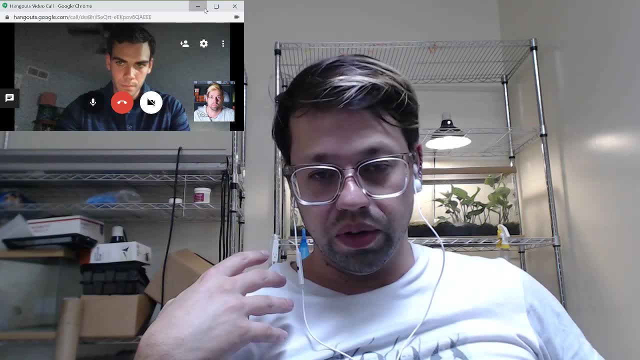 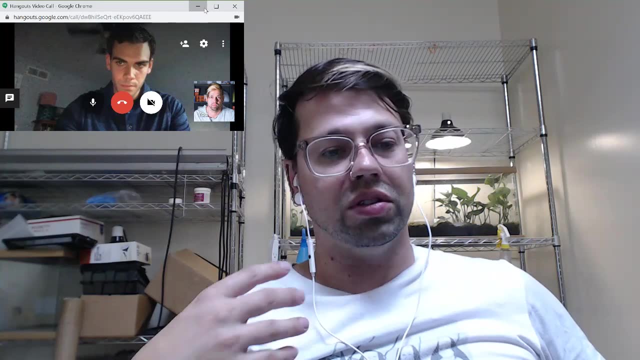 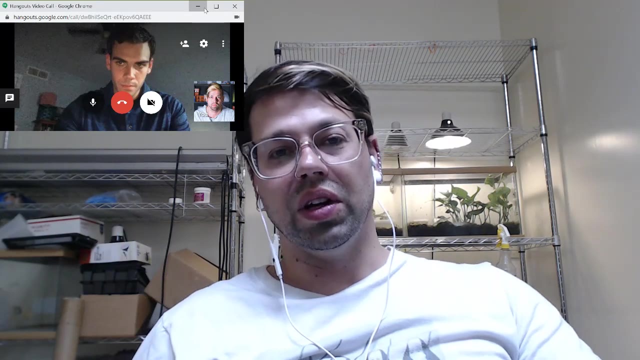 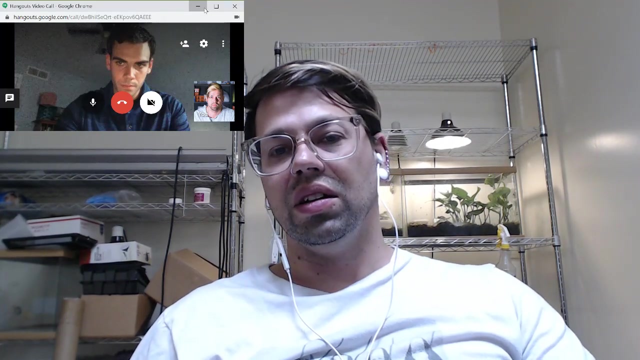 sure, make sure you, you know, reinforce those skills by performing the experiments. it never hurts to perform the experiments. if you've been working in a lab for ten years or something like that, then maybe you can get away with not performing these things, but you know, it's always a good idea. 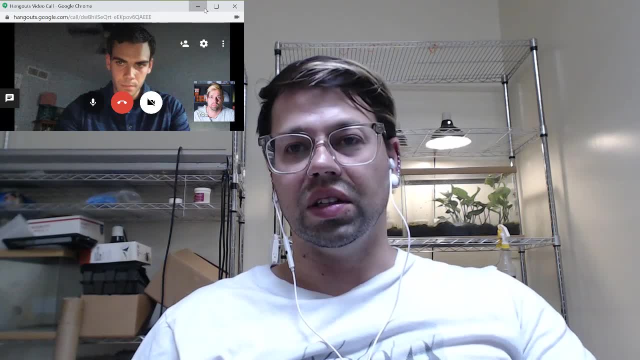 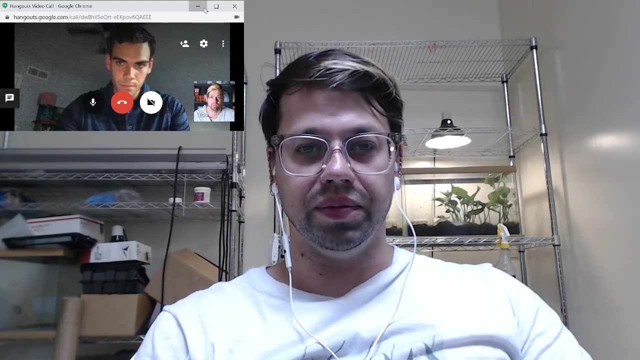 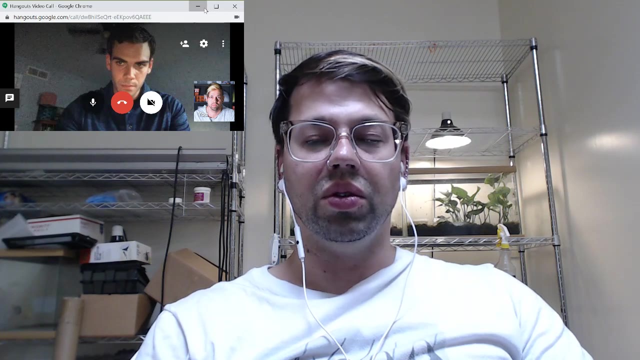 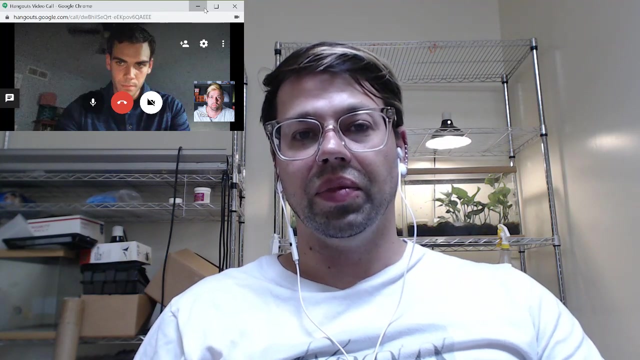 to go over these, these skills and experiments, to brush up on it, so you know what's going on. if you have any questions, please try and post them in the google classroom. that's the easiest way for the instructors to answer the questions and other people can also gain and learn from your questions. 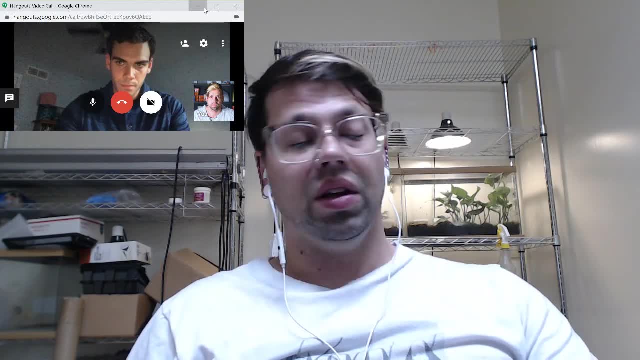 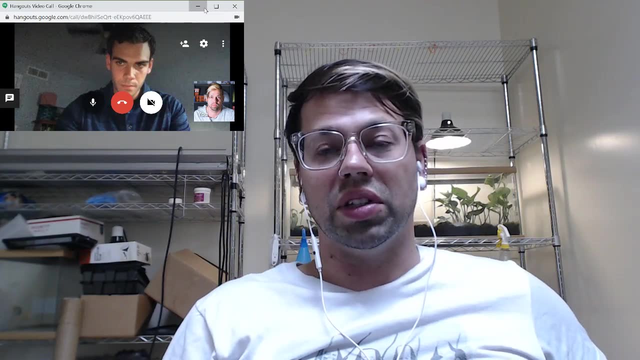 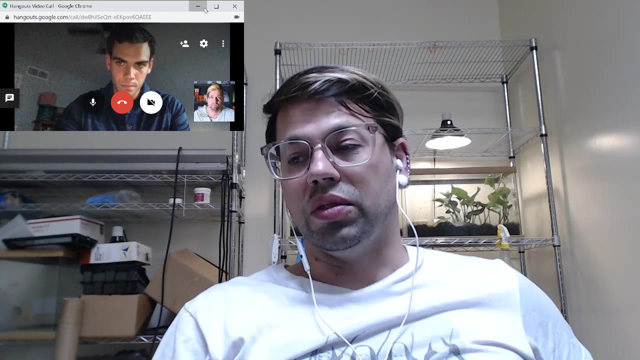 so try and post them in the google classroom. the live streams of this class are going to be every week at um 4pm pacific time, california time- um, so try and make it out for these live streams. we're here to answer any questions you have. 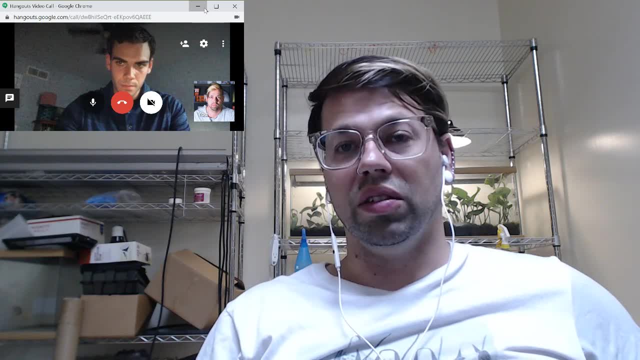 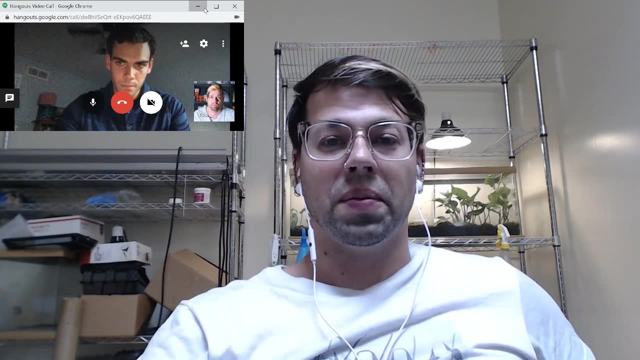 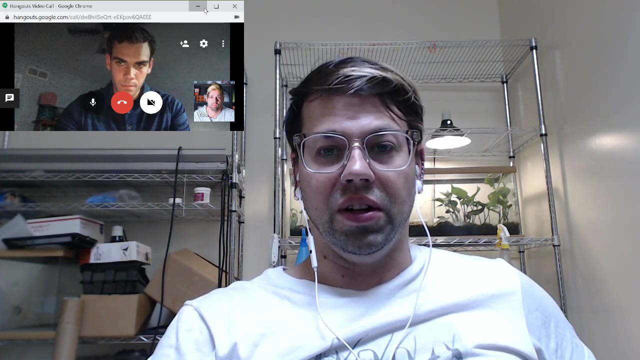 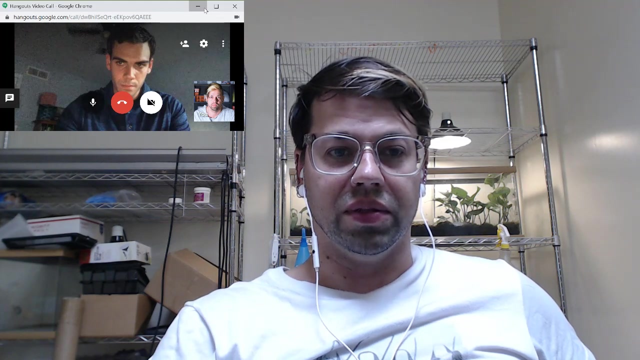 um, help you with experiments, give you advice on your love life, whatever you need you just come to us. we're here to help you all, right? um? so does anybody have any questions right now? um, about, about anything that's going on. anybody any questions? how are things going? is everything? 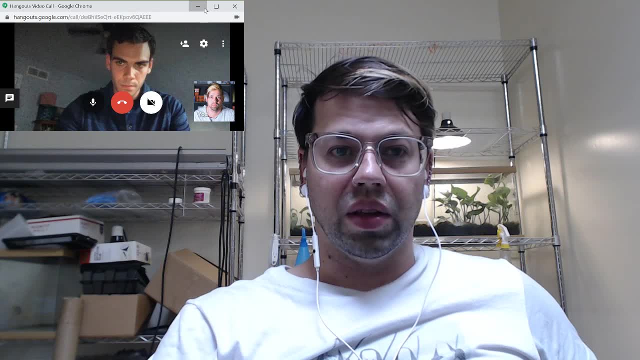 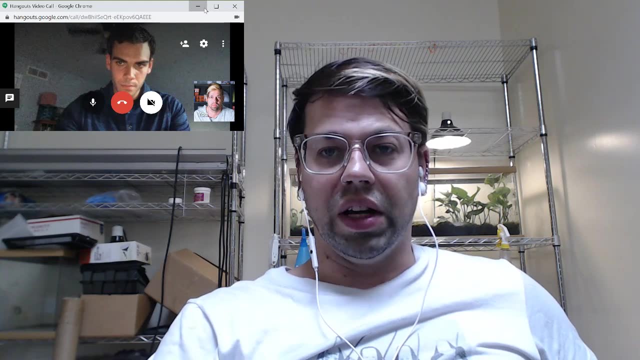 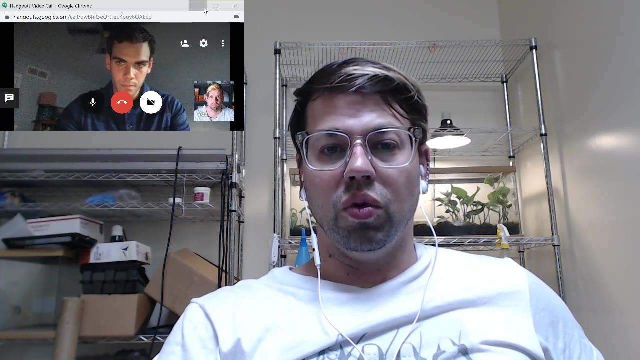 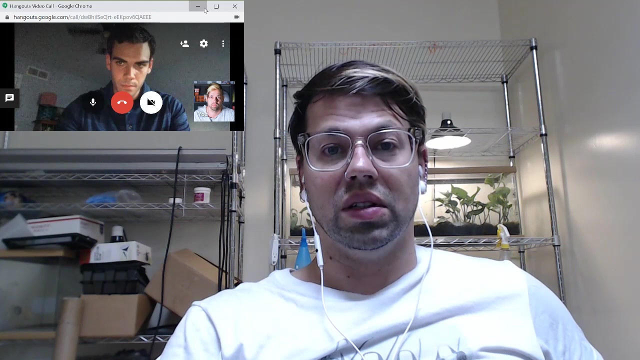 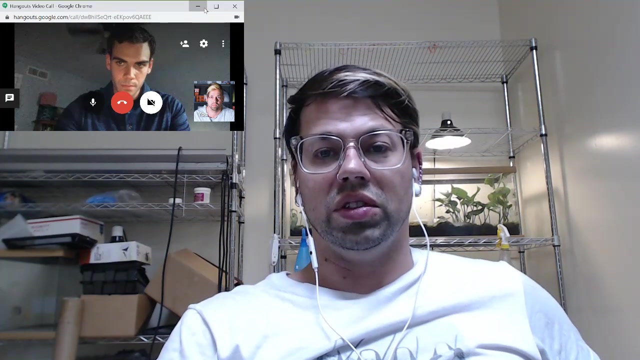 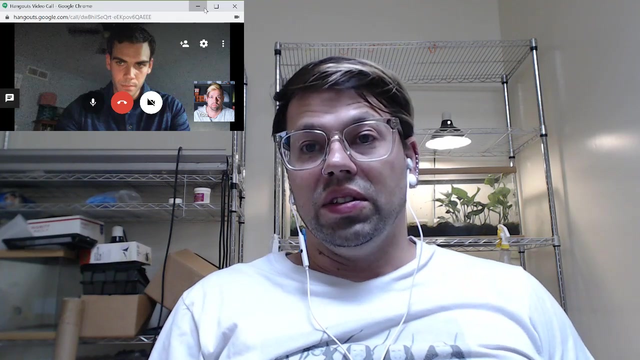 going good, yes, no, alright, great, sounds good, alright. so the first week what we're going to learn about is: we're going to learn the first and second week about cells. cells are a really interesting phenomenon, right? because cells, all the cells that we know. 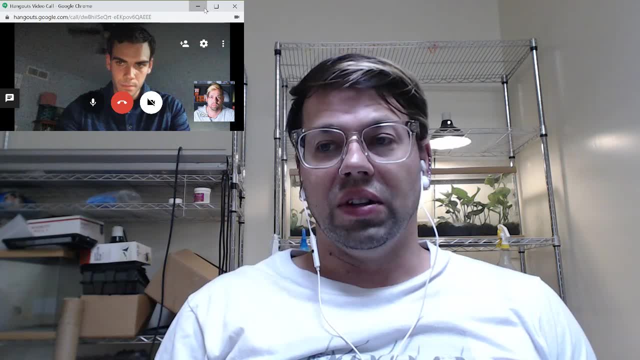 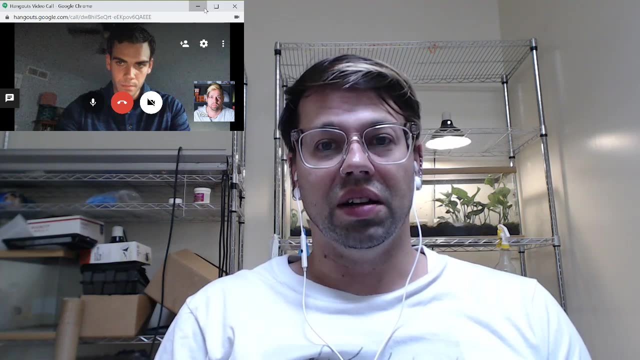 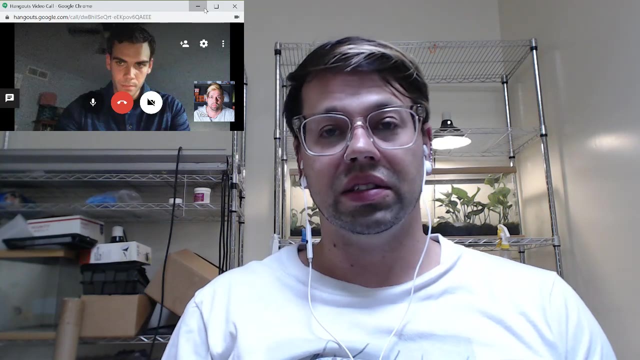 of only come from other cells, right? so there are no cells that we know in existence that haven't come from other cells And that kind of you know blows the mind. we can't recreate cells from scratch, not yet at least. the only thing we can do is replicate cells and modify those cells that. 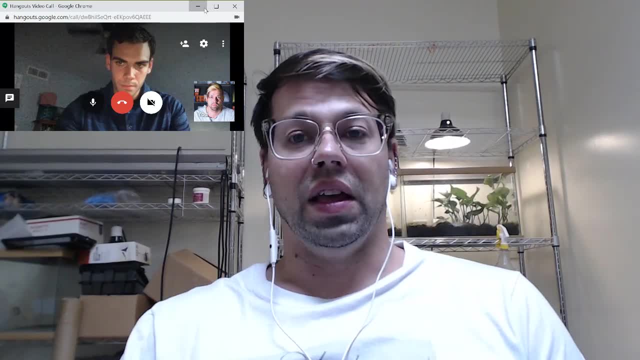 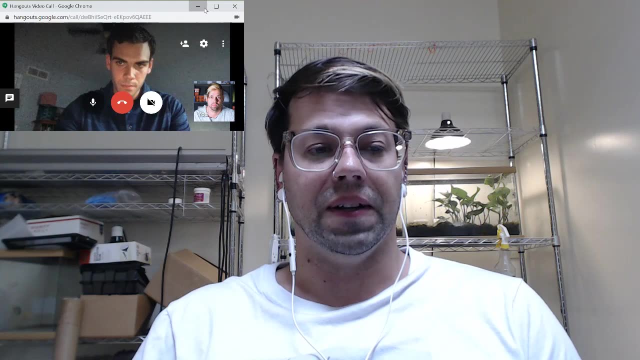 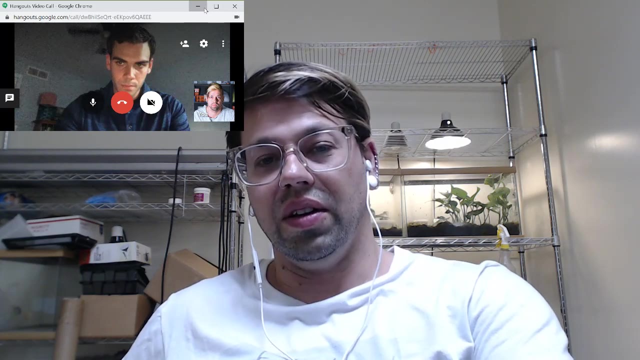 we replicate and it makes you think a lot about where the first cell came from. where the first cell came from, how is it able to do what it does? Some people are, you know, under the impression that maybe the first cell came from an asteroid or outer. 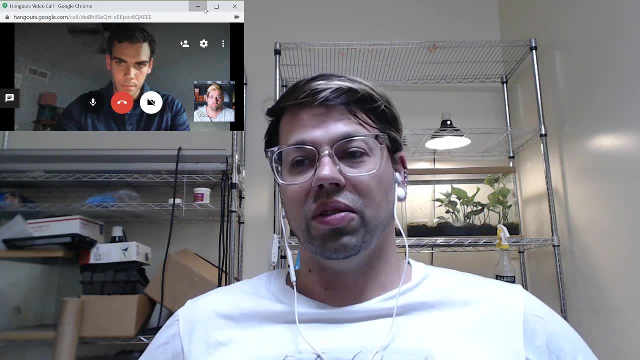 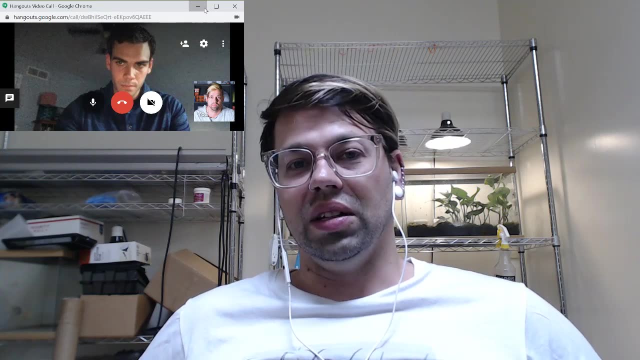 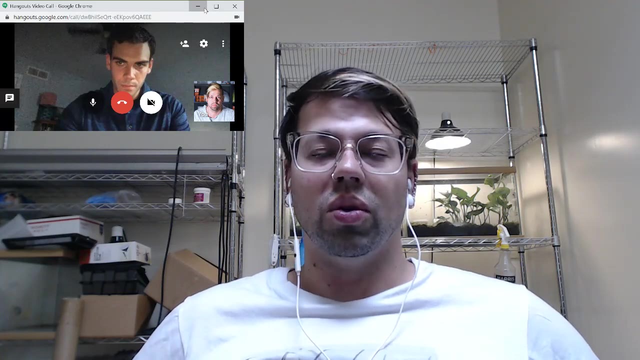 space, another planet somewhere, and landed on Earth and seeded the planet through pan-sperma. Other people think that, you know, cells just develop through evolution. lipids that form the cell wall just naturally formed into this. you know, lipid micelle shape. 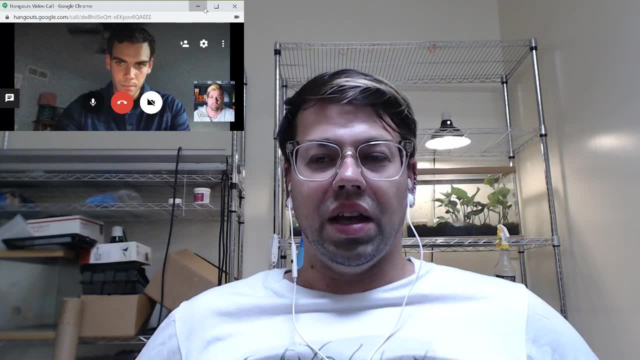 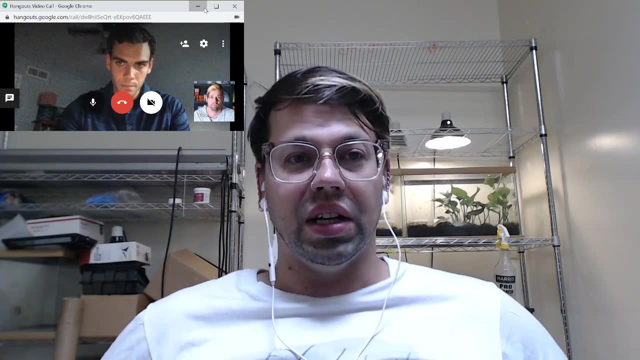 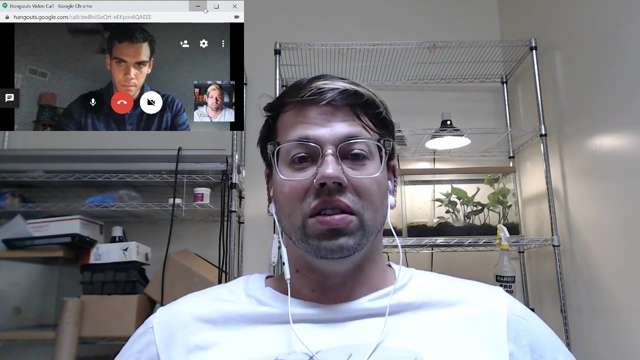 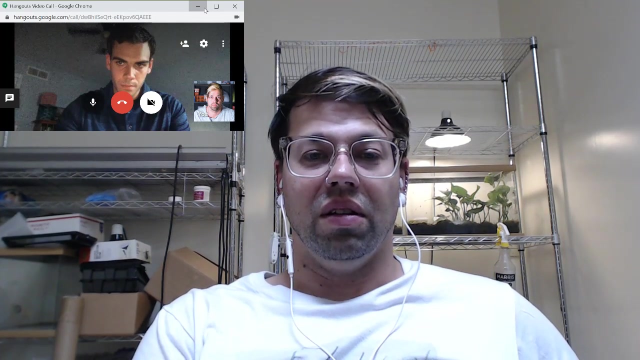 And encapsulated DNA and proteins, and you know organisms were born but honestly, you know, we really don't know. we have no idea where cells came from at all no idea. So you know that's something that people need to figure out. 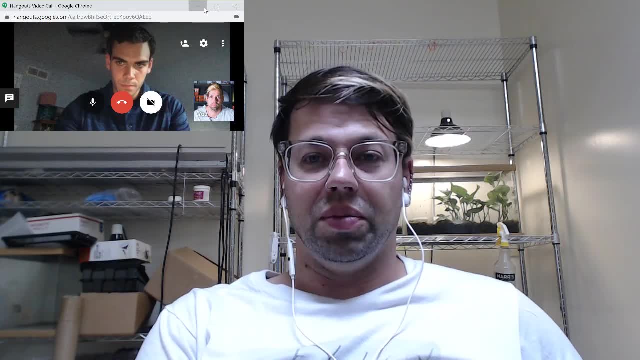 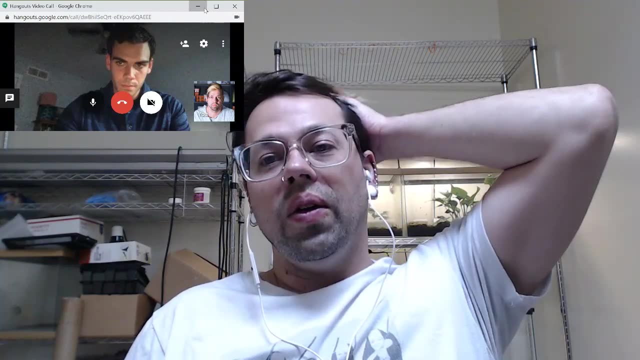 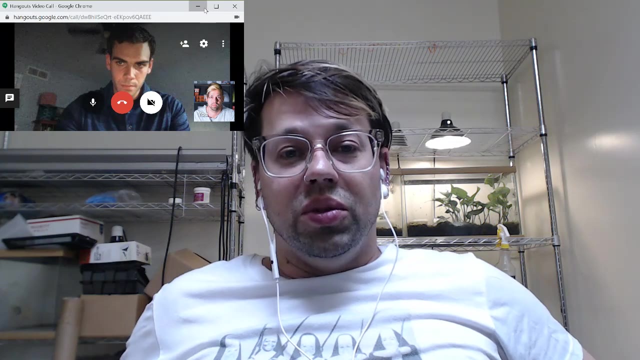 I know there's a a bunch of people right now it's starting to become really popular- in trying to create synthetic cells like try to create a cell from scratch. That's going to be really interesting when that first happens. They've tried lots of different ways to figure out how to do this. it's just cells are complicated. 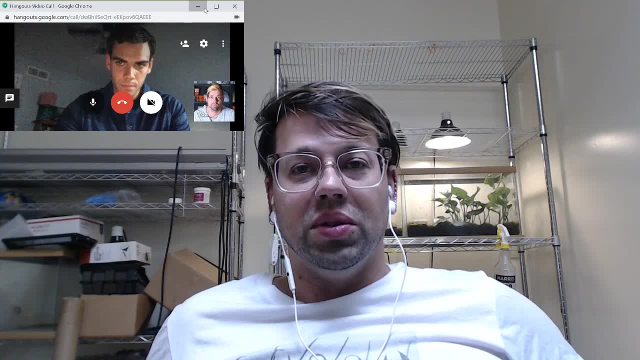 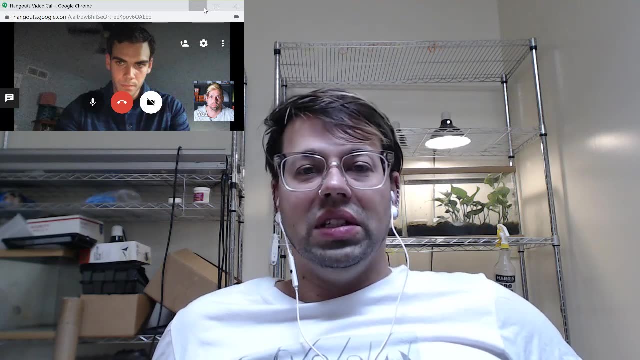 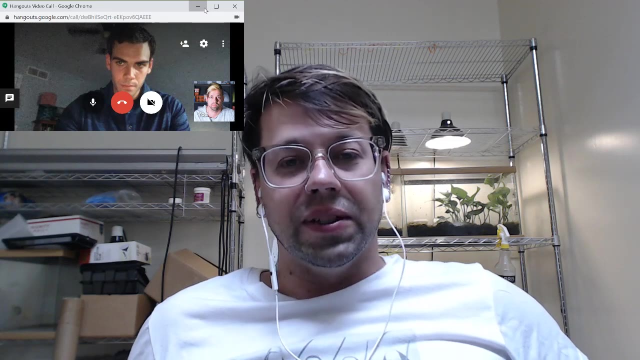 they really are right. The cell is composed of the cell wall, different organelles inside the cell, DNA, proteins, cells, Different molecules, small molecules, electrolytes, salts, all these different things. Having them in the cell is 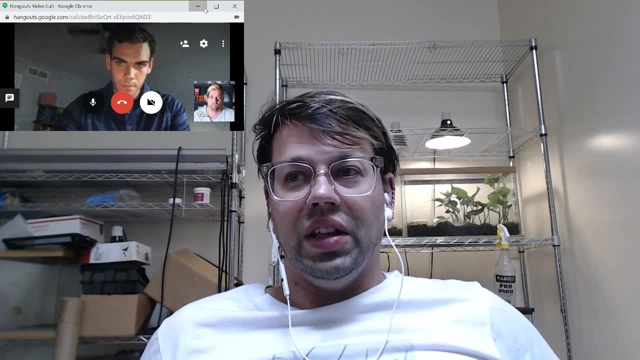 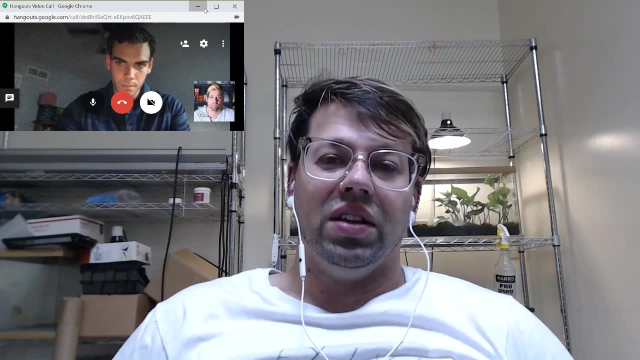 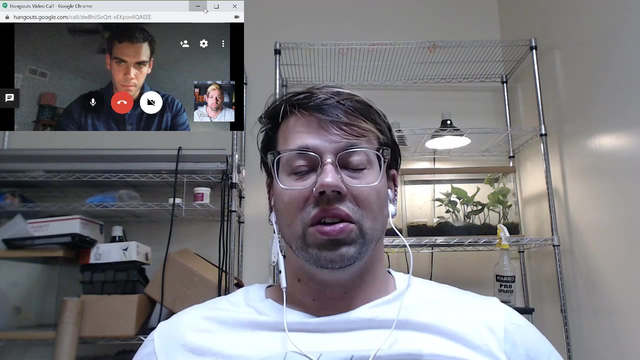 It's difficult. And not only that. like cells are all different, right, So like a human cell is much different in shape and size than a bacterial cell, Even bacterial cells are different between each other, Right, They're different in shape and size. 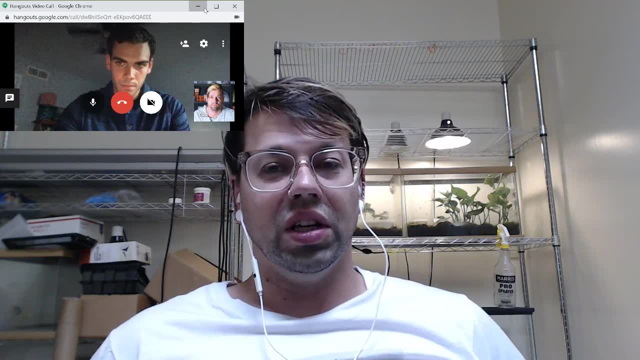 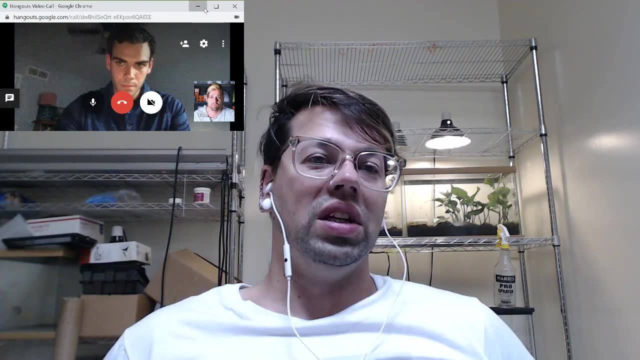 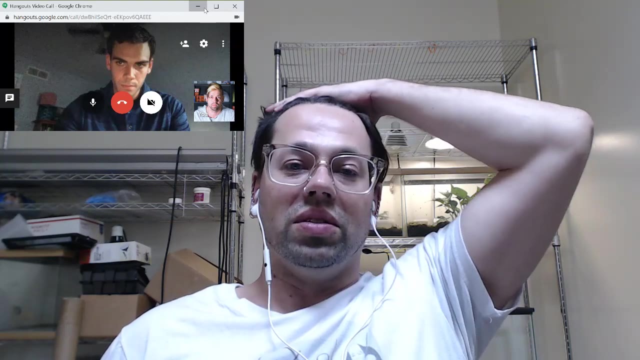 Now, bacterial cells are generally much, much more difficult to see under a microscope than human cells or plant cells or yeast cells. These cells are, you know, maybe almost ten times bigger than bacterial cells, And bacterial cells are really nice. 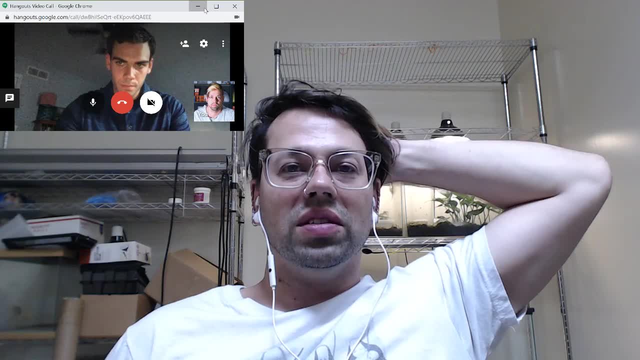 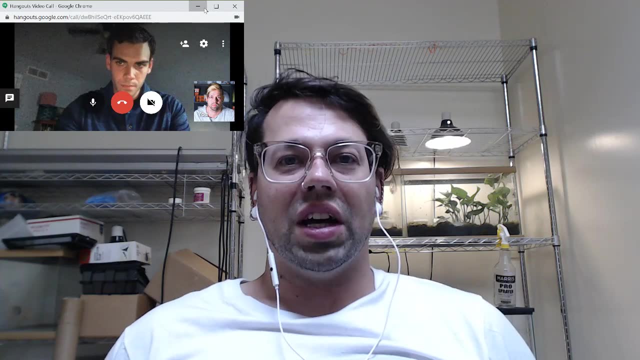 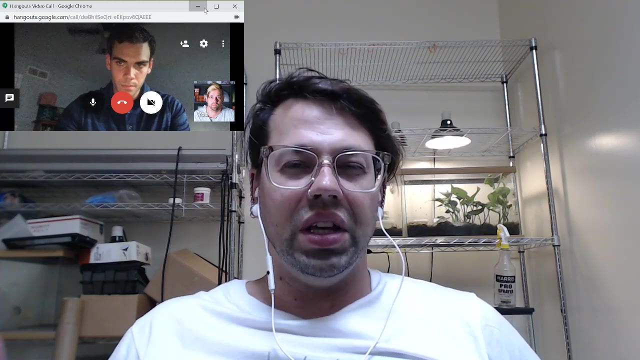 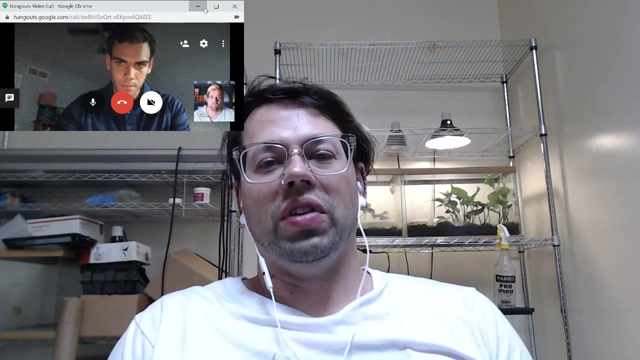 Through this course, We're going to work mostly with bacterial cells, and that's because bacterial cells are quick to replicate, right? So the amount of time it takes for a bacterial cell to replicate is like 20 to 45-ish minutes. So what you can do is you can grow bacteria and grow it fast. 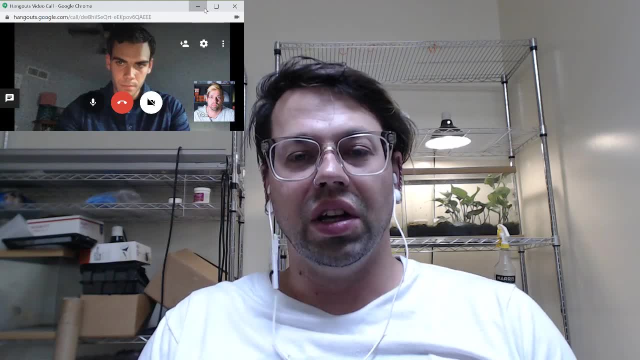 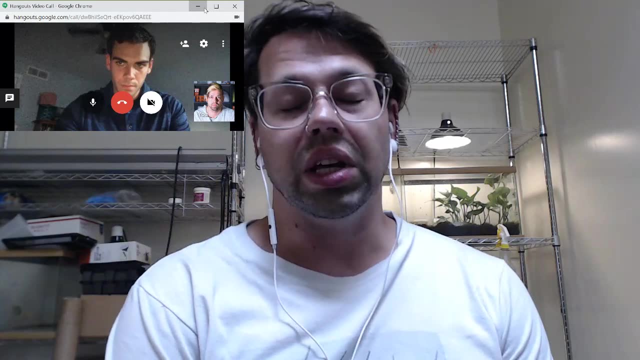 So when you're working in molecular biology and genetic engineering, you can get the results from your experiments pretty fast. Whereas yeast takes much, It takes, you know, a few days, and plants take, you know, tens or months, tens of days. or months. Human cells are kind of intermediate between bacteria- I mean yeast- and plants in which, if you're trying to genetically modify some human or mammalian cells, it can take, you know, five to ten days-ish or something like that. 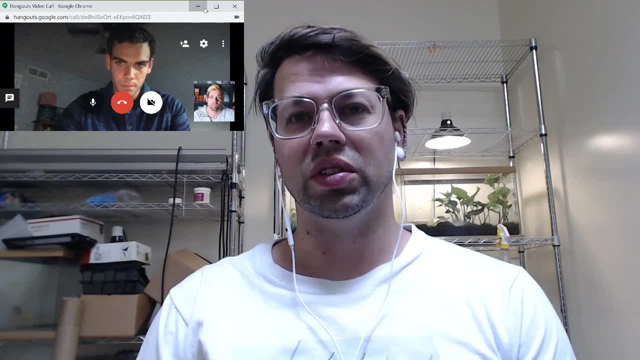 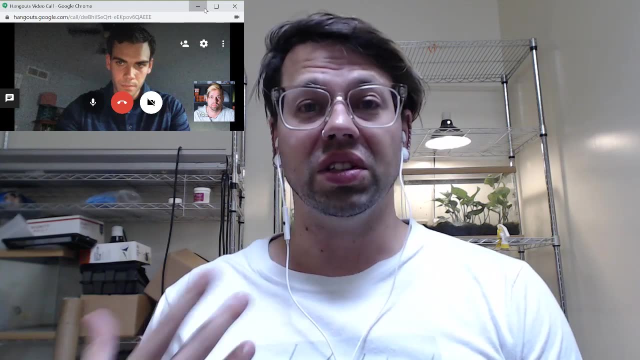 All right. So yeah, this course focuses on bacteria because it's small, it's easy to grow And understand. all the bacteria used in this course is not hazardous. It's not harmful, So you don't have to worry about that at all. 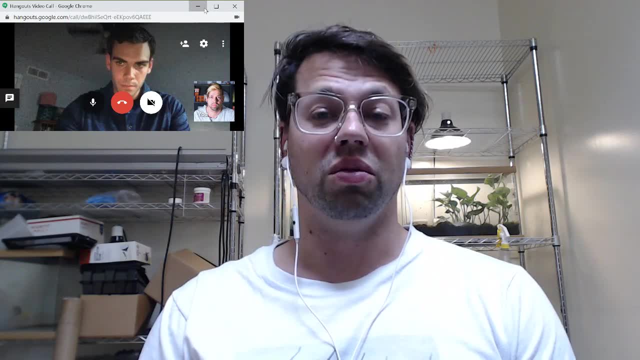 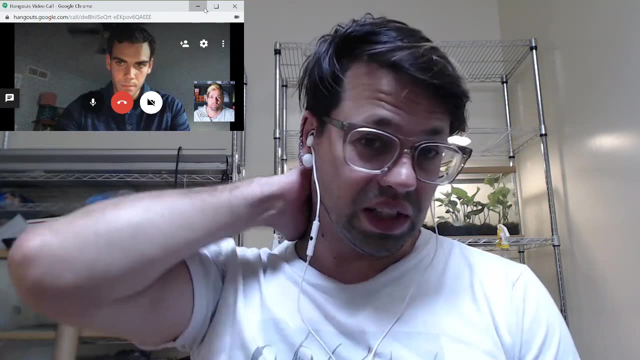 The bacteria won't kill you, no matter what you do. You can eat the glass vial that the bacteria is in and you're probably not going to kill yourself. I'm not saying you should eat it. It's not a good idea. 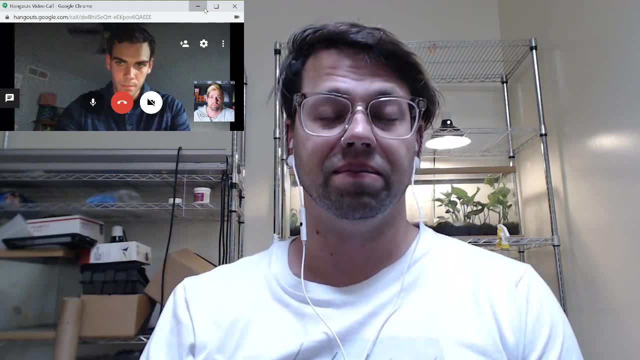 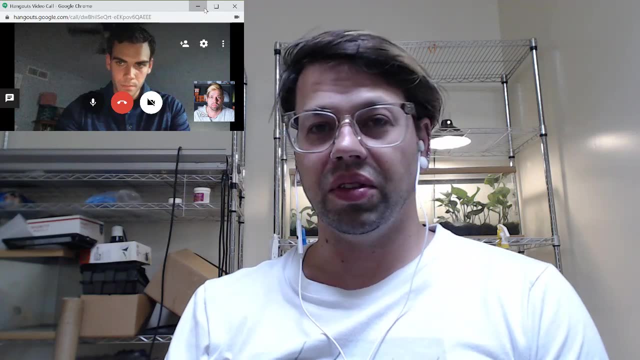 But you know, Yeah, All this stuff is pretty safe, so don't worry too much about it. Bacteria gets a really bad rap right When you think about it. it's like less than 1% of the species of bacteria that actually. 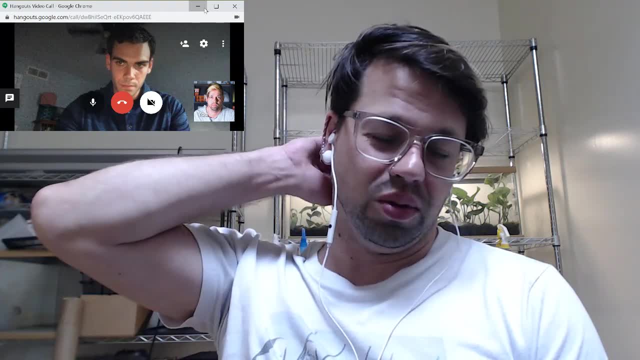 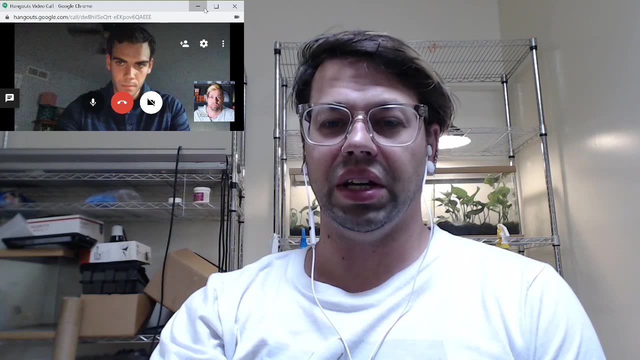 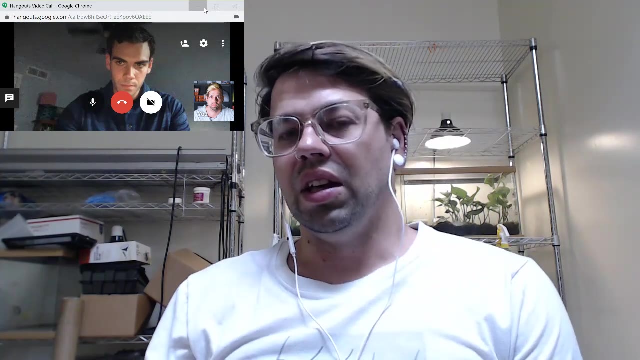 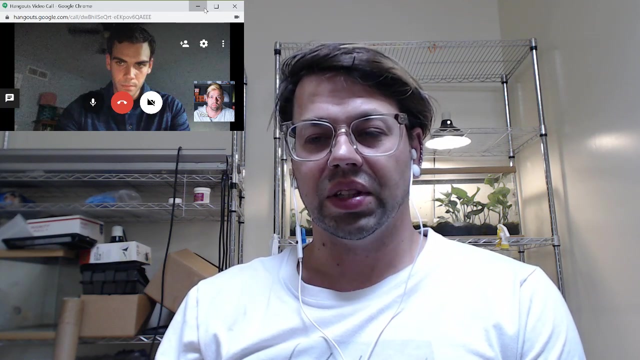 cause any sort of illness or disease. right, So you know, understand. bacteria are the workhorse of molecular biology. If you're going to do molecular biology and genetic engineering, you're going to have to learn to work with bacteria. It's just the way it is. 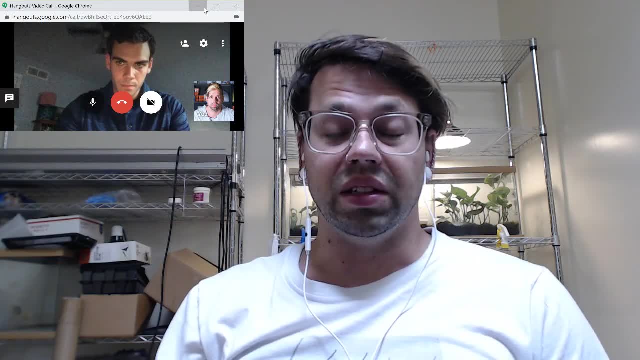 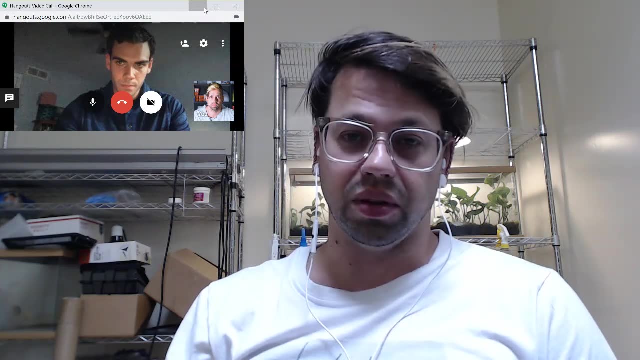 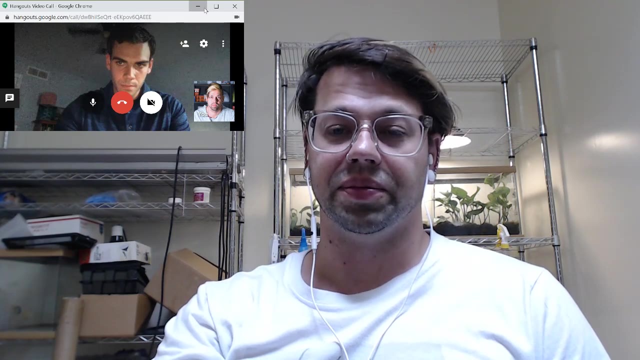 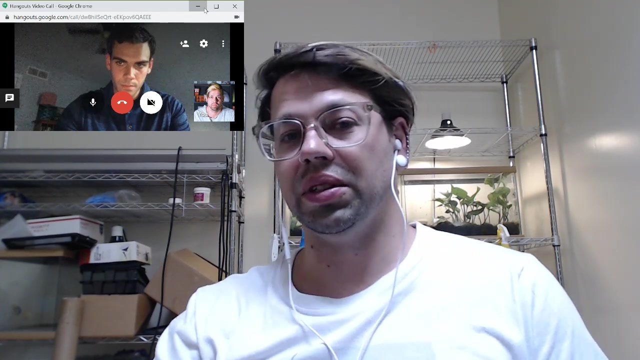 Because it doesn't matter how hard you try to avoid it, you're going to have to use it for purifying DNA or expressing a protein or doing some experiment. Bacteria is going to be there. So you know, get used to working with bacteria and that's the reason we do it. 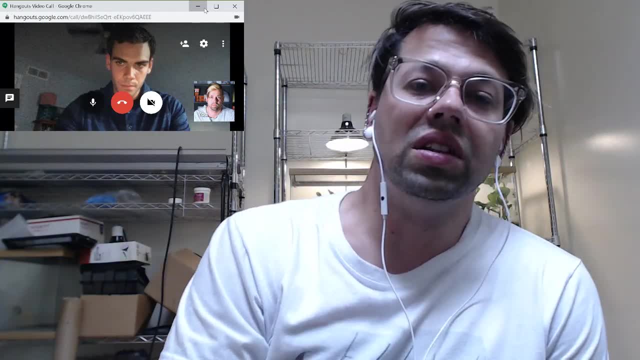 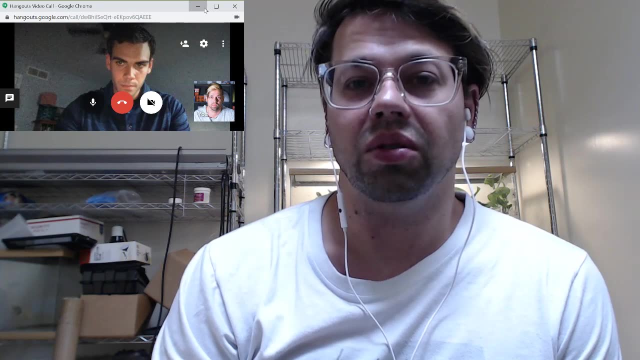 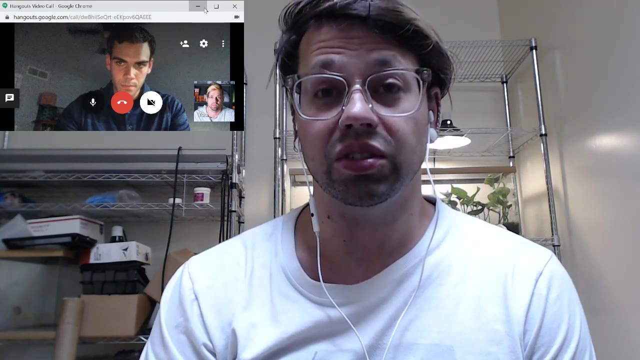 So basically, all living cells have DNA. Now I know some people might be like: well, what if you say a virus is alive, or something like that? Not all viruses have DNA. And that's true, Not all viruses have DNA. 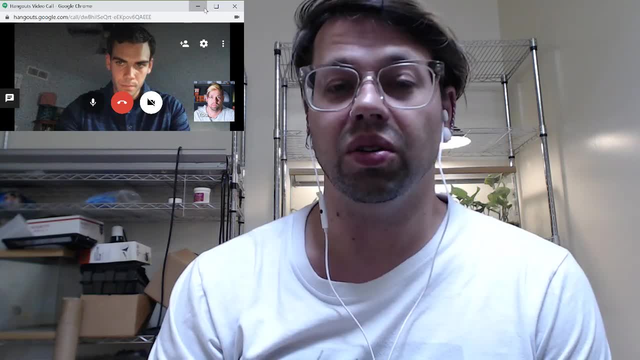 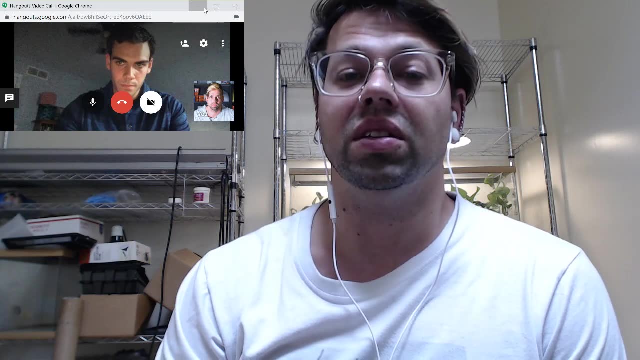 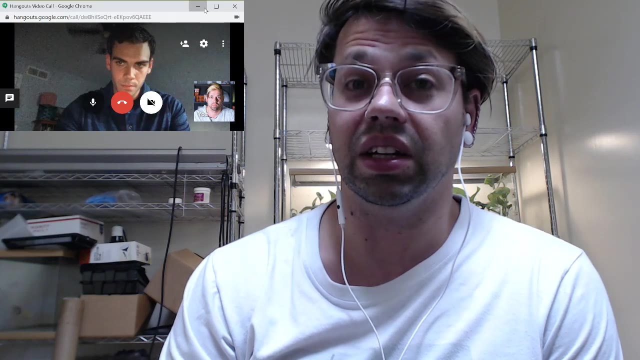 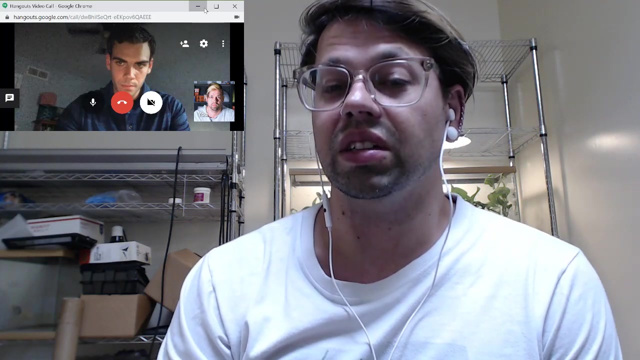 Some of them just have RNA. But you know, if we say, just like all viruses aren't living because they need a host, then all living organisms that we know of have DNA And they usually go about the process of replicating their DNA and making proteins. all in the same. 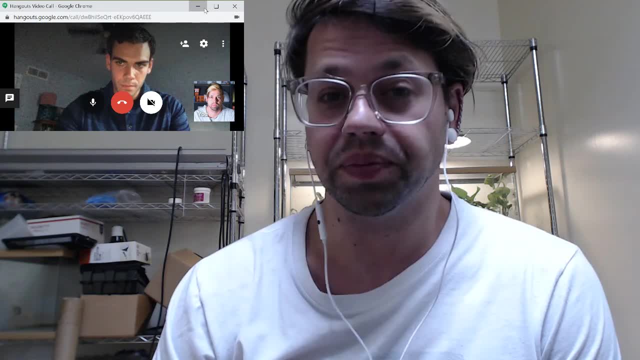 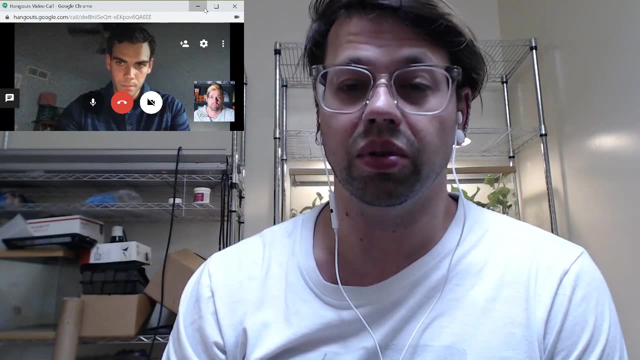 or very similar ways, right? So if you're going to do molecular biology and genetic engineering, you're going to have to work with bacteria. So inside the cell, when organisms are replicating DNA, the proteins involved are similar. A lot of things about the process are similar. 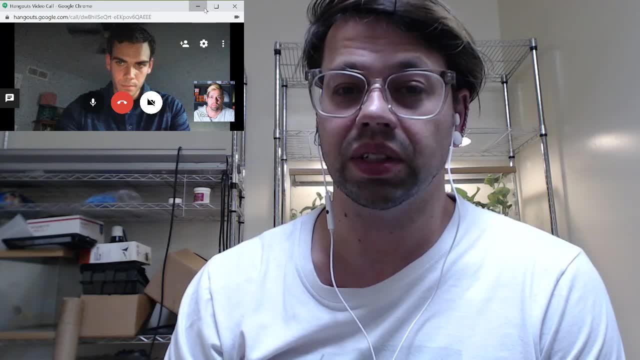 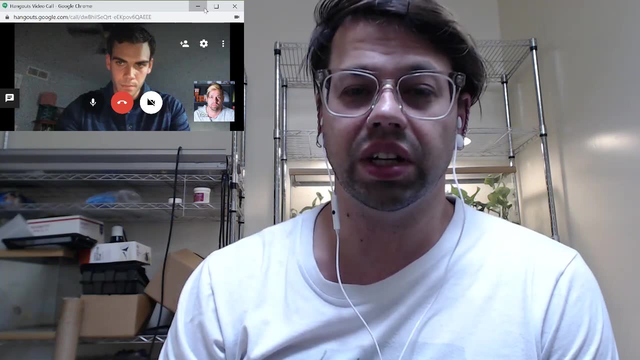 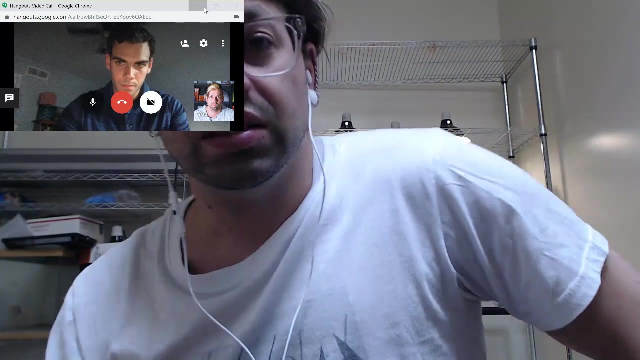 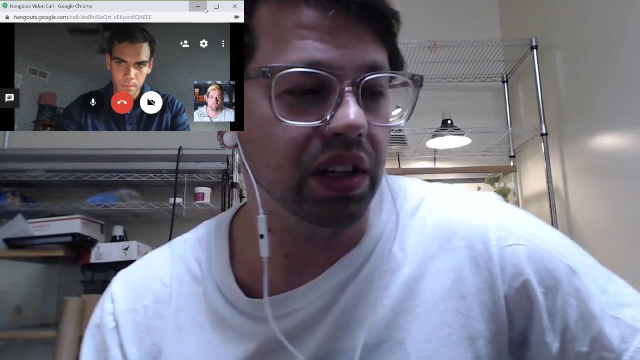 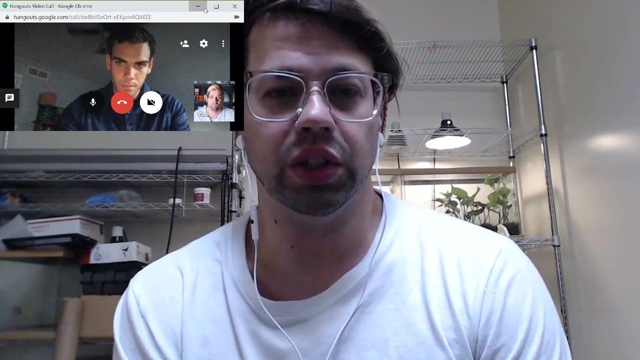 It's very similar in many different areas. So, despite cells having, you know, different shapes and sizes and different size of genomes and different amounts of DNA, Okay, Generally they all abide by very similar principles of function, using, you know, channels and using DNA replication and protein translation and all these different things. 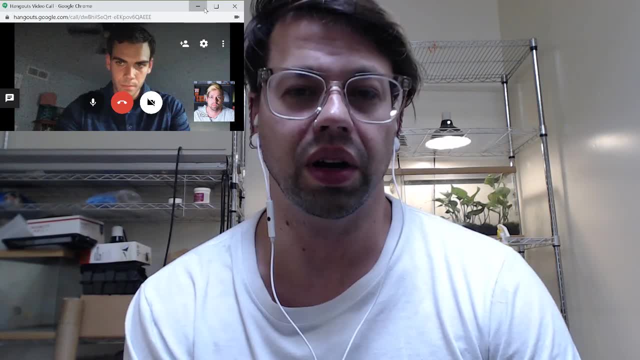 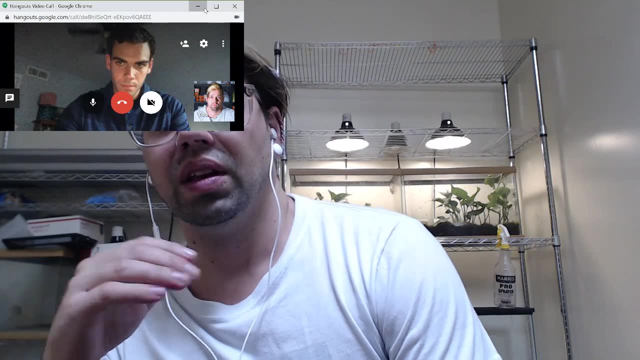 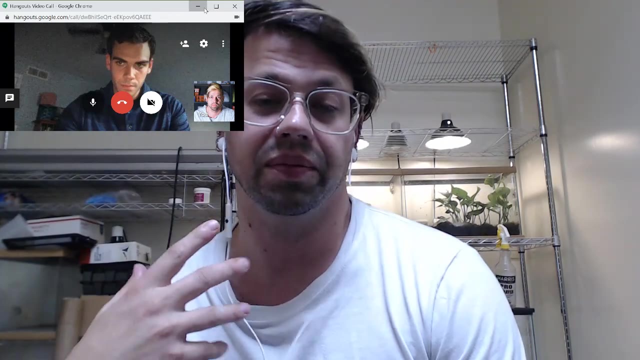 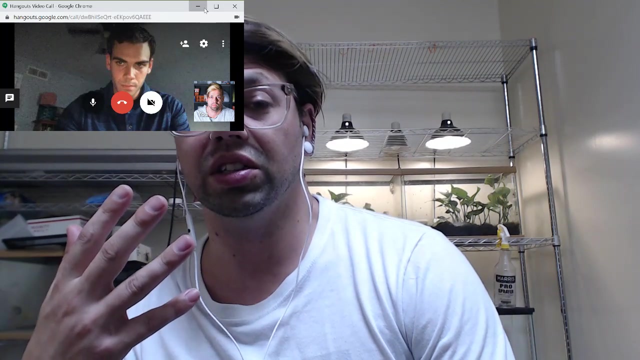 We'll learn more about these things in the class, And if you read the Molecular Biology 101, it'll have- or Molecular Biology of the Cell. it'll have a lot of information on these things, right? So don't worry too much if you don't know a lot about it, but go to Molecular Biology of the Cell. 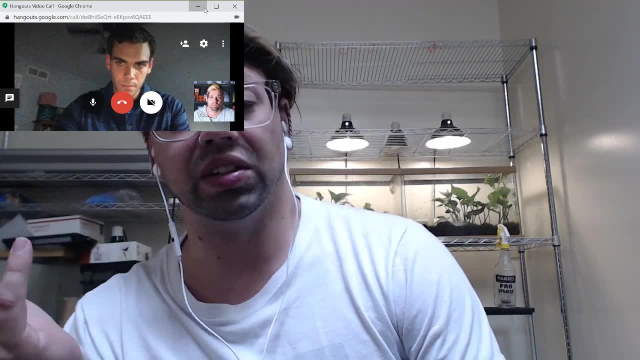 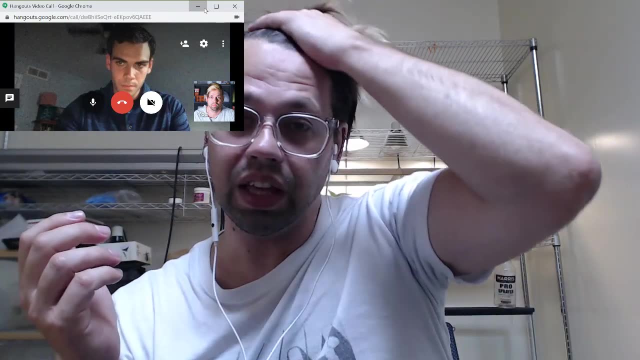 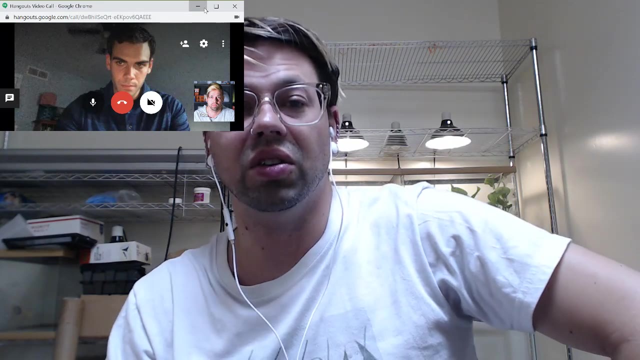 It's free. You can search it on the internet and find it. Molecular Biology of the Cell. It's a book that you're not going to need. You don't need to know everything in, but generally, at one point of time or another, the information in that book is good to have. 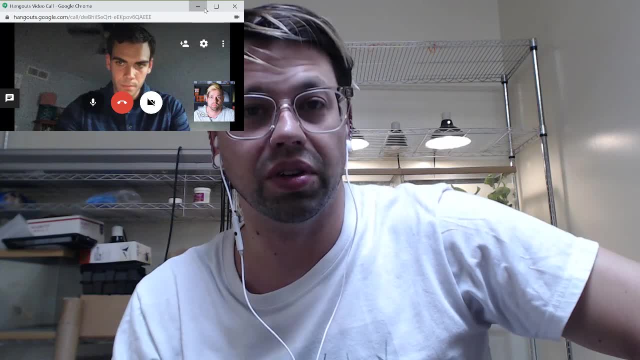 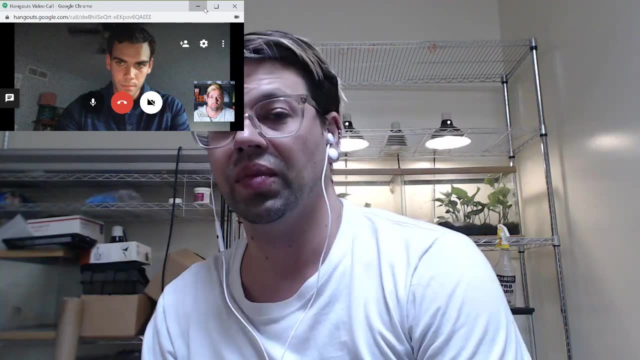 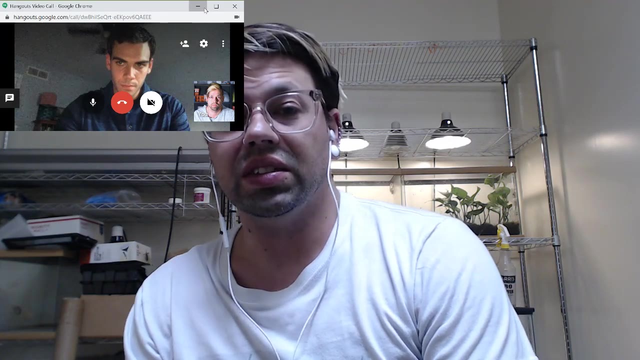 The knowledge in that book is good to have and it'll be very beneficial to you as you pursue a career in molecular biology and genetic engineering, right? So the things that go on in these cells happen because of proteins. So DNA Turns into RNA. 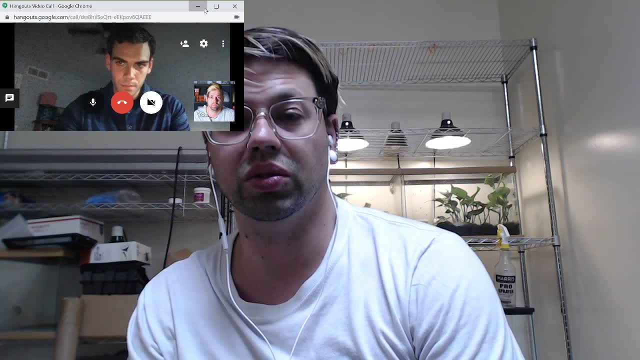 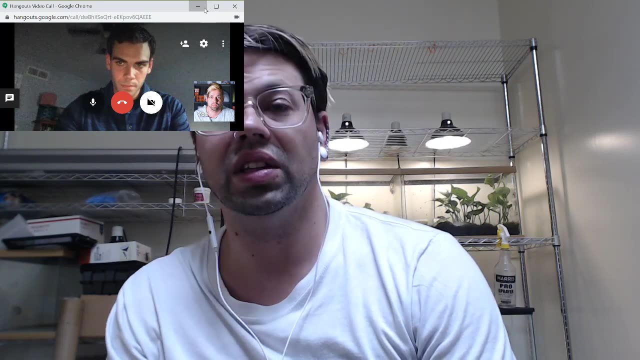 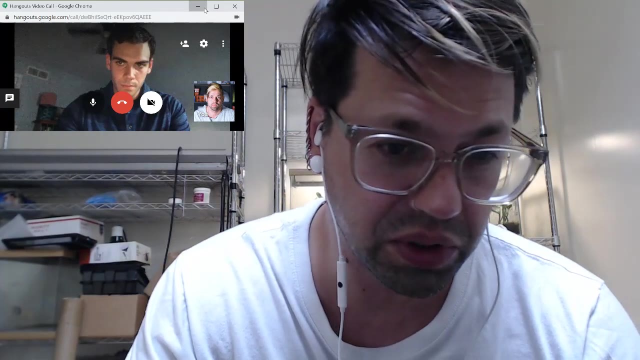 Turns into proteins. They call this the central dogma of molecular biology, And proteins are these little machines that keep cells alive. If you go on like YouTube or something, let's see if I could find a YouTube video about proteins moving around, and then you could see what's going on. 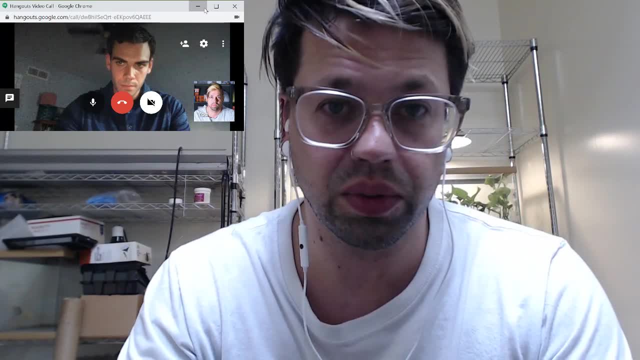 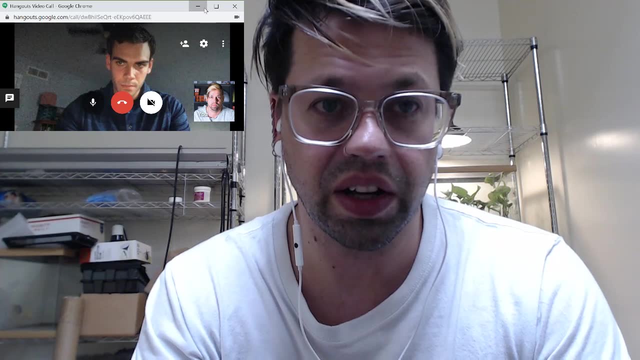 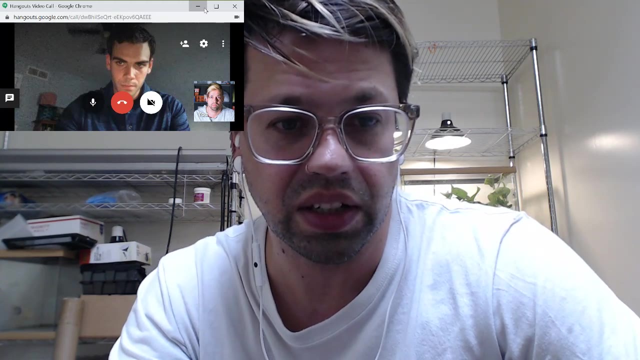 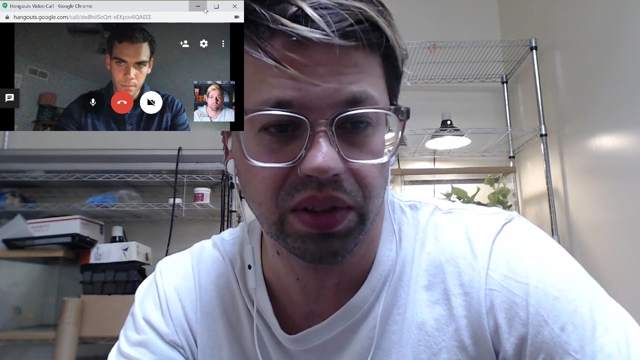 And like proteins are actually super cool. So you have to understand that, like DNA and proteins are, they're just these molecules, that kind of flop around inside cells and do things right, And them flopping around and doing things is basically what keeps you alive. 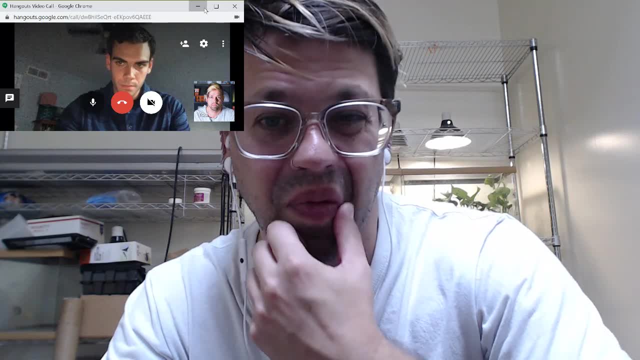 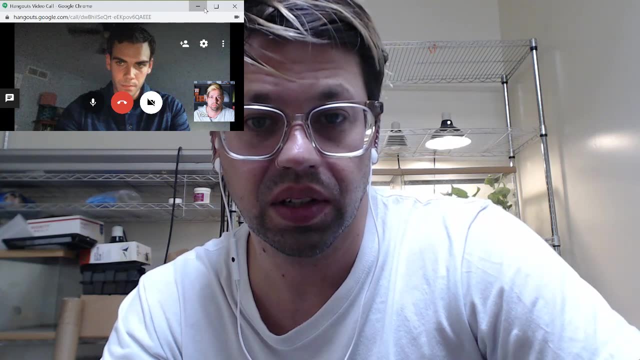 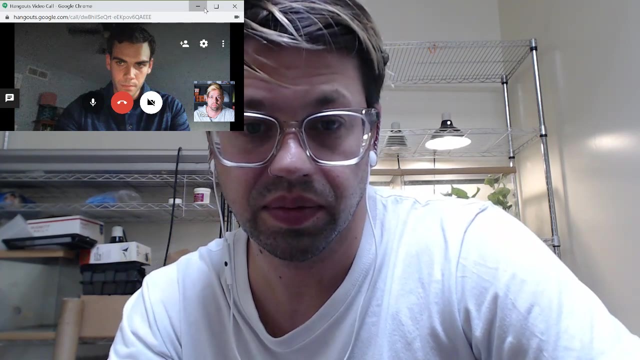 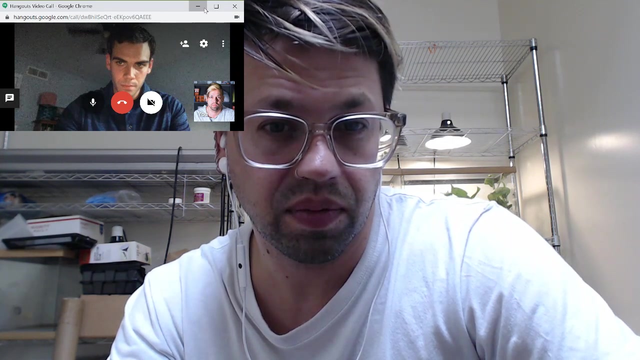 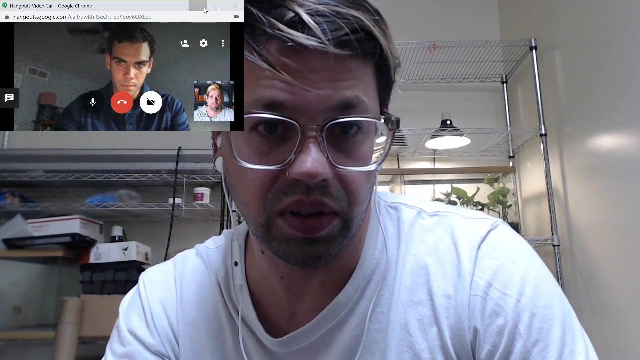 Let's see What do we got, Trying to find a protein simulation. Let's see. All right, I don't know if this is, I don't know if this is, I don't know if this is going to show up. well, 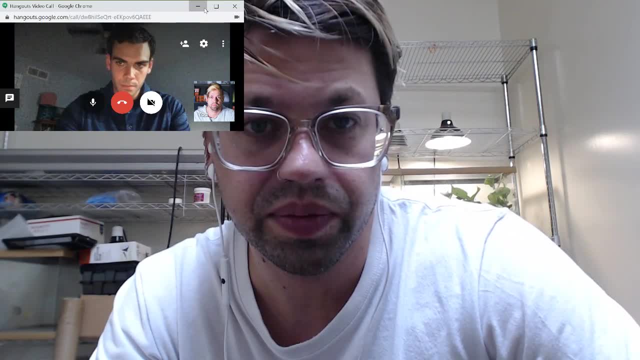 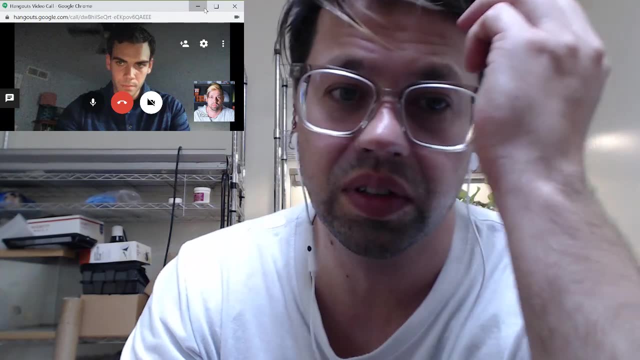 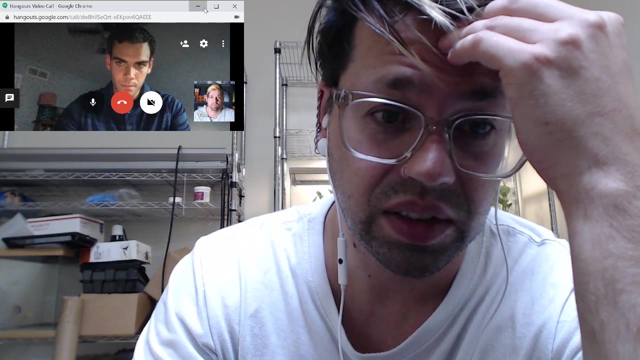 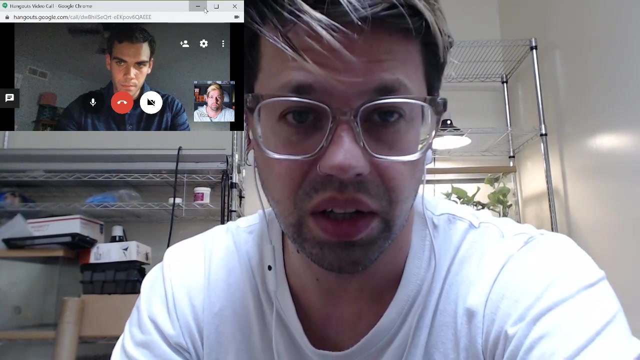 Hmm, Let's see. So, yeah, you have to imagine that proteins are these little small, you know tiny things, nanometers in size, that move around. right, They're in water and they're fluctuating in water and moving around. 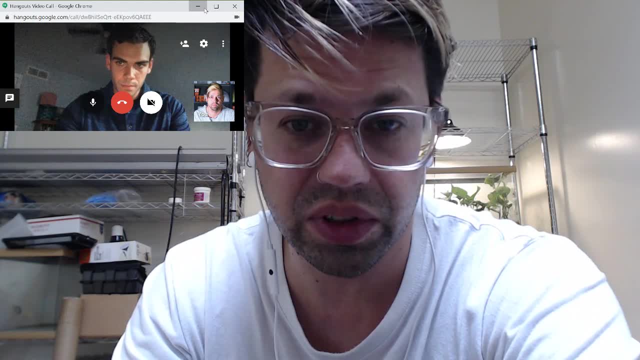 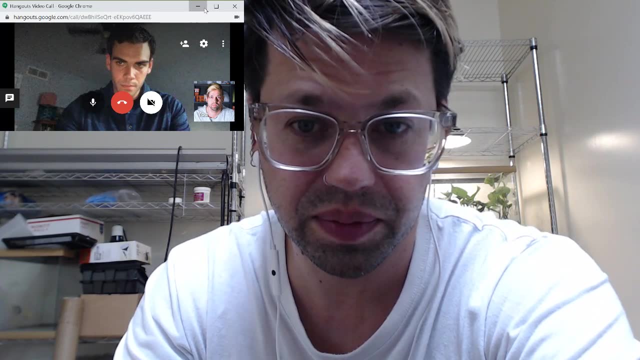 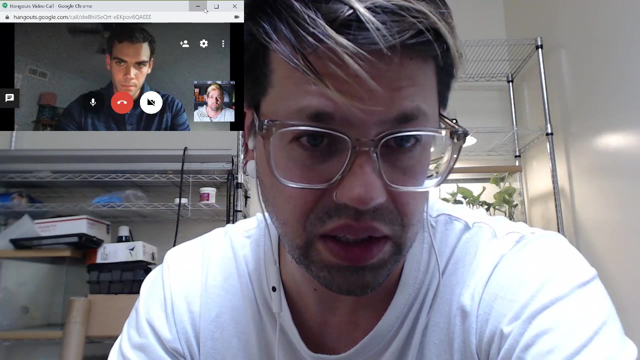 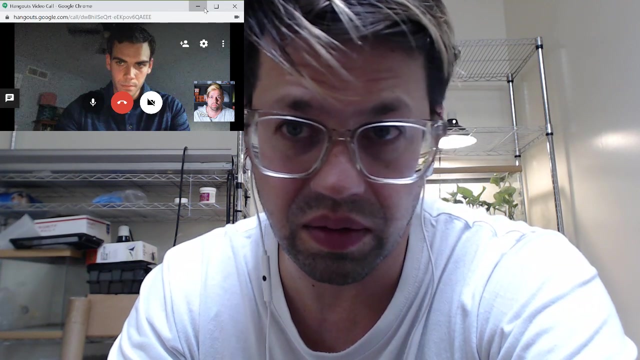 And, you know, waiting for stuff to happen, Trying to figure out what they should be doing. So I guess this is protein folding simulation, But it'll probably be interesting anyway. All right, Let me see if I can pop this window out. 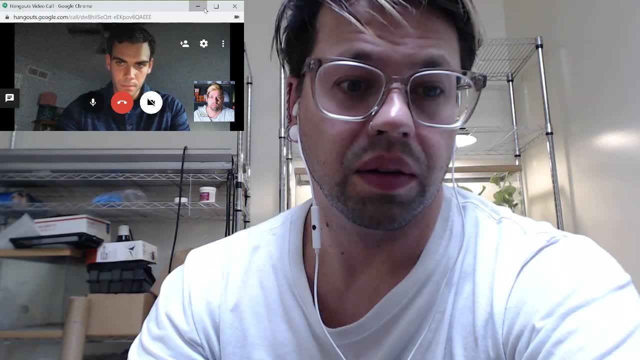 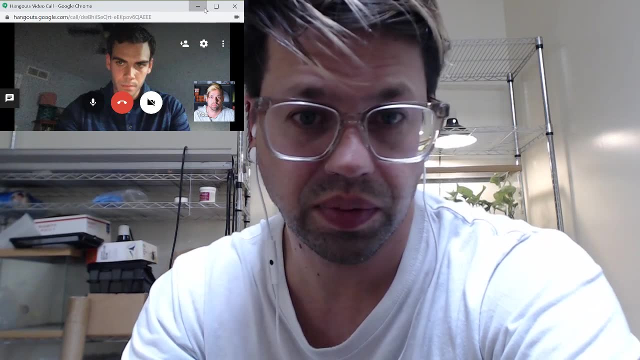 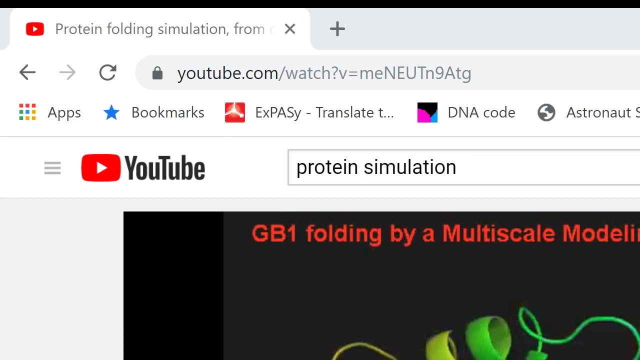 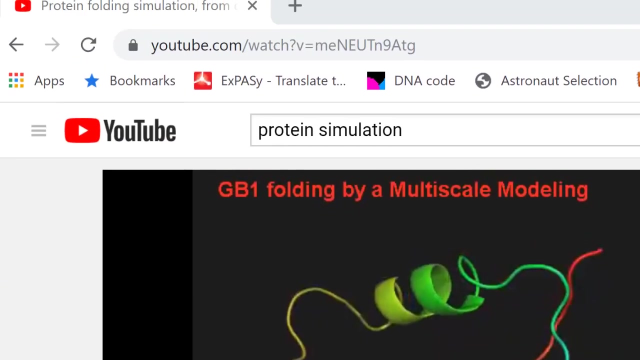 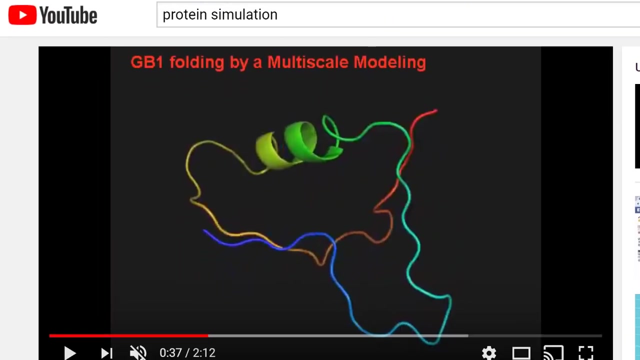 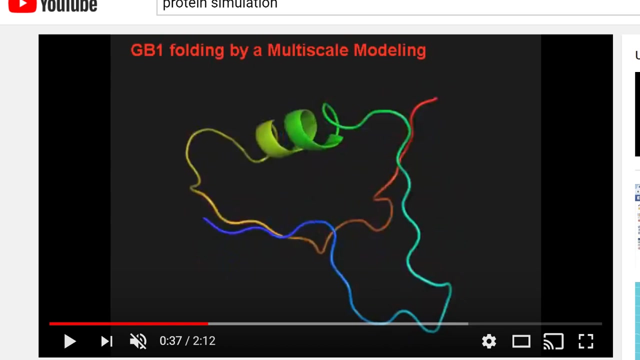 All right, Let me add in a window Window capture, All right. So what we're looking at here is we're looking at a simulation of a protein. So basically, what somebody did Was they just calculated Newton's laws of motion for the different atoms and molecules in a protein. 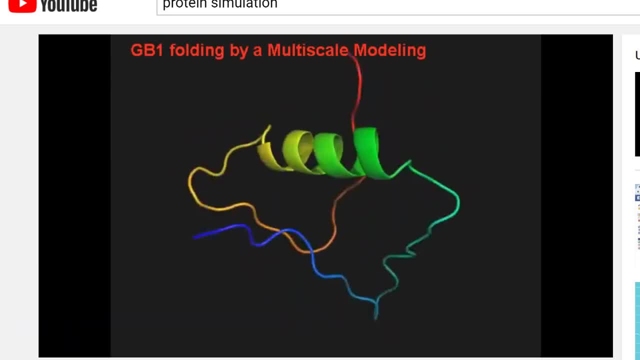 What a protein would be like if it was in water. And this is kind of what it looks like. It's just kind of flopping and moving around and doing stuff. But this moving around right, Its ability to move around in water. 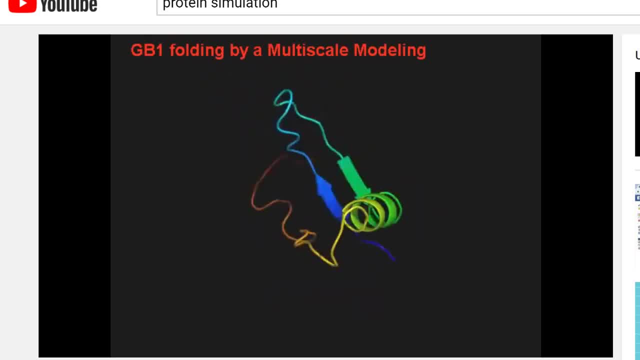 Gives it machine-like properties, so then it can actually do things right. It can bind to different things, It can, you know, release different things, It can cause chemical reactions on different things. But yeah, that's basically what a protein would look like if a human were looking at proteins. 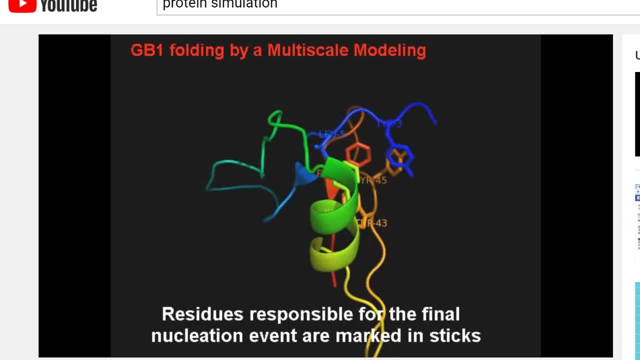 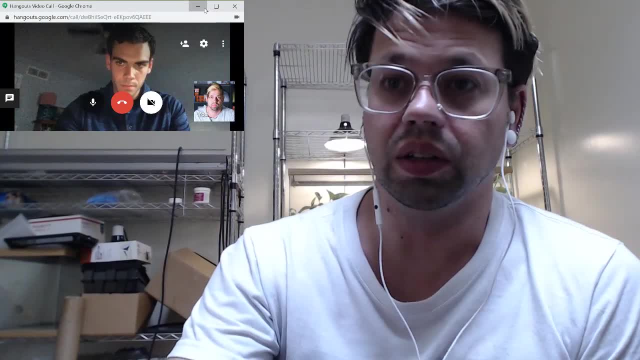 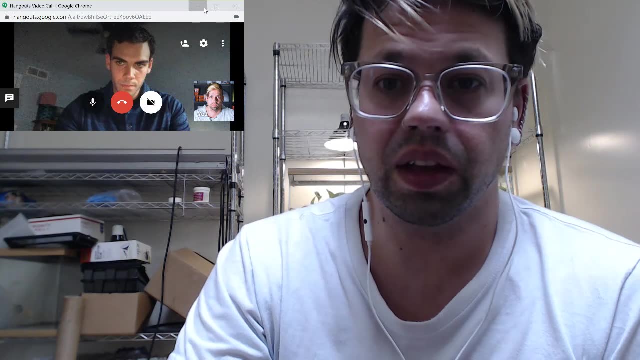 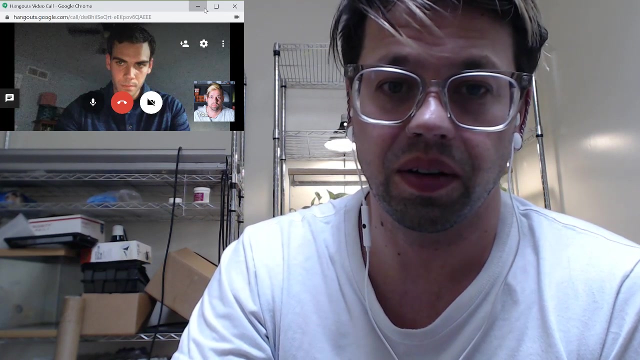 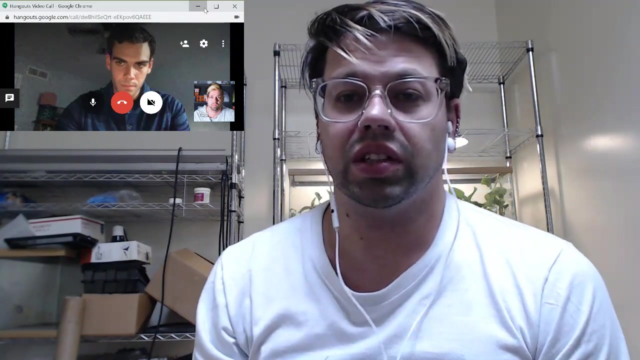 So Proteins are little machines made by DNA and help cells do their thing. They help cells, you know, stay alive, grow, function, whatever, All right. So, Even though you know, cell sizes of human cells are bigger than bacterial cells, 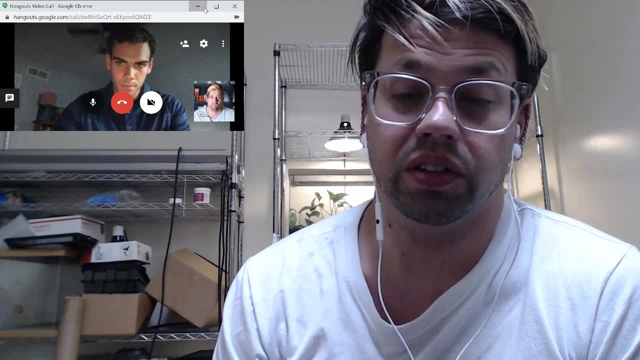 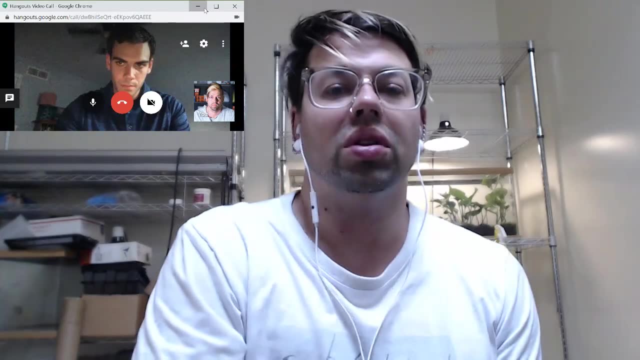 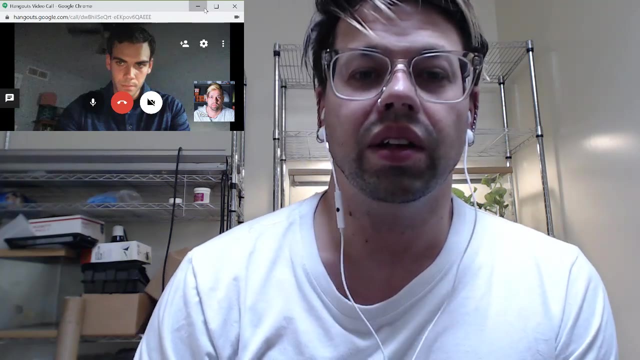 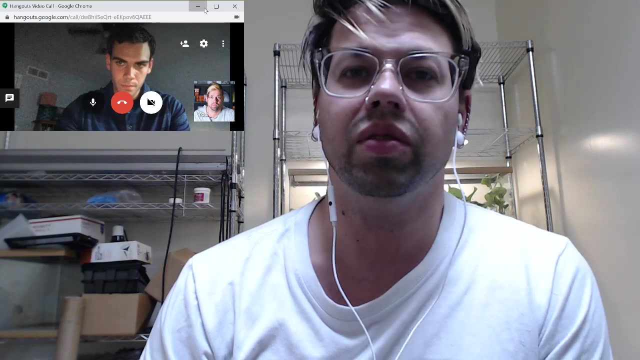 You know, And human genomes are bigger than bacterial genomes. Don't make the assumption that, like a cell size or a genome size, the number of bases in the DNA of an organism correlates with the complexity of the organism, right? So humans don't have the largest number of genes or the most complex DNA or genome. 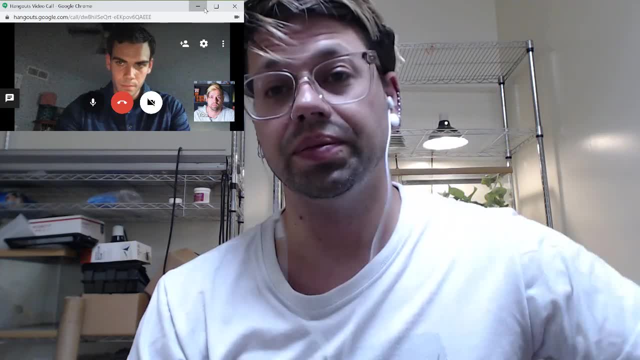 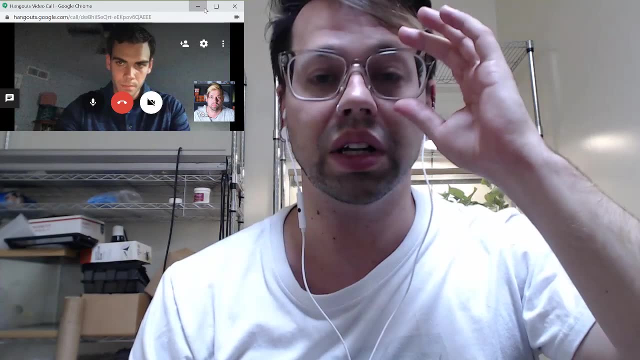 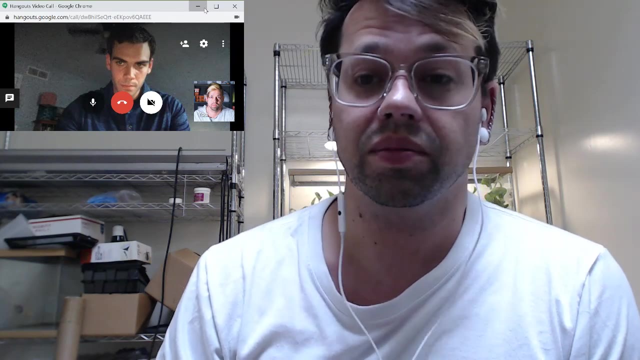 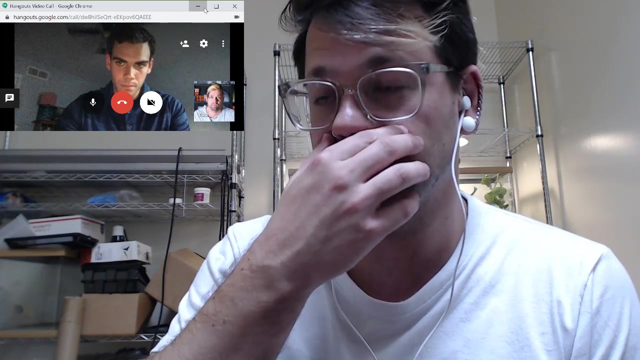 Of all organisms, Right, So they might have a larger number of genes and bacteria and stuff like that, But they don't have the most genes. Some organisms, like plants, have so many. They've gone through genome duplication events So they have so many different copies of their genes, right? 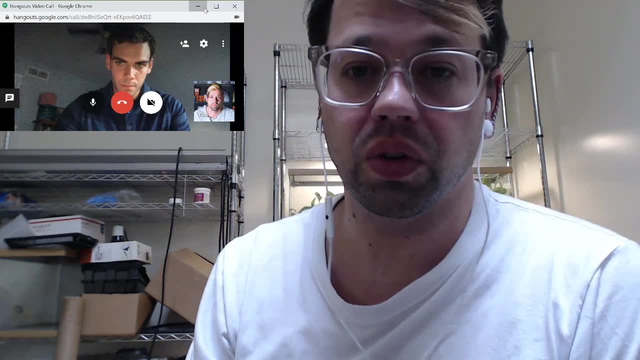 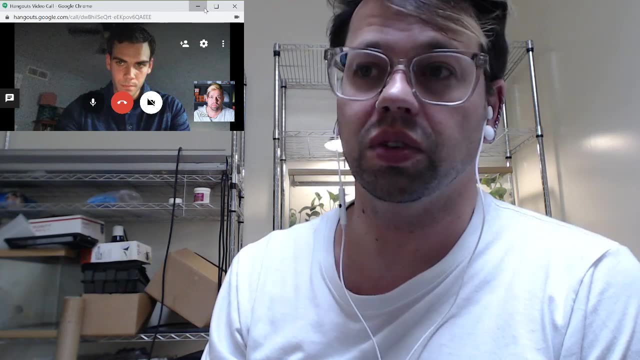 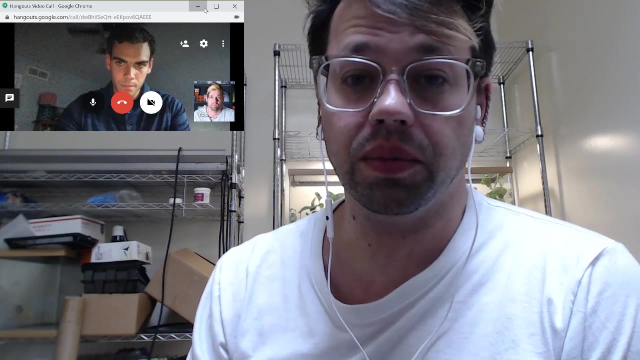 So humans have 23 different chromosomes And We have two pairs of each chromosome, So we have a total of 46 different chromosomes And then our sex chromosomes, Right? So Some organisms have like 10 pairs of chromosomes and stuff like that. 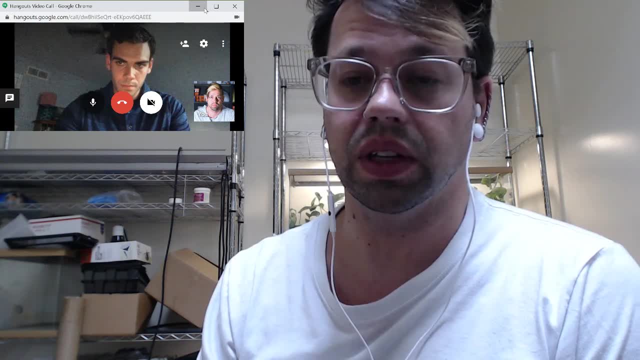 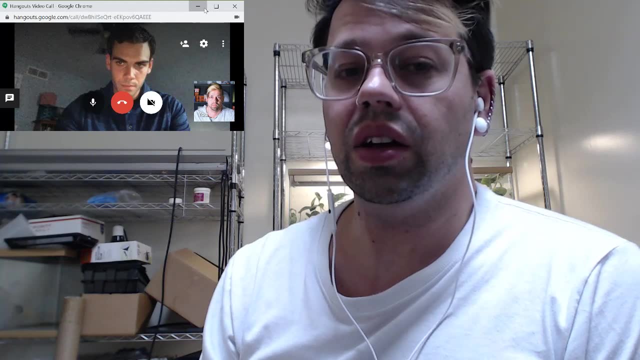 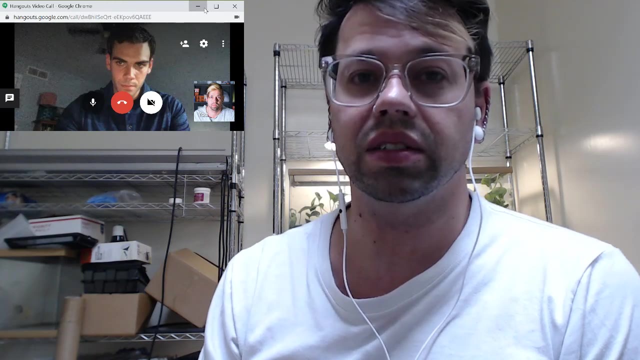 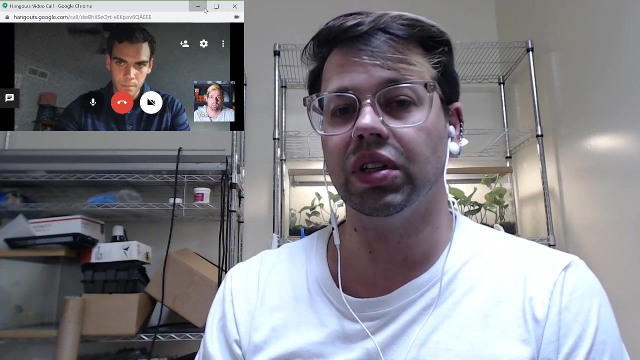 And they're way more primitive than humans- They have way more genes than humans Even So- And a lot Of Modern science, Especially medicine. You see a lot of stuff about how, like Mice and rats and fruit flies and all these organisms. 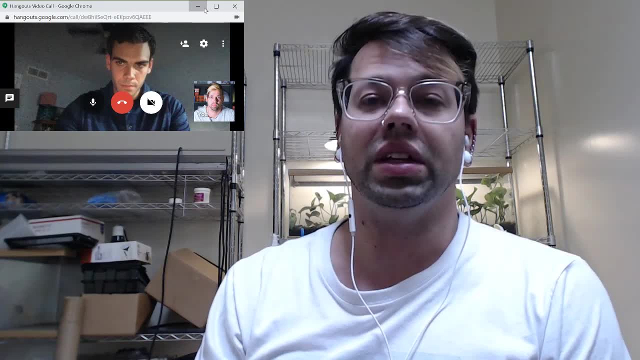 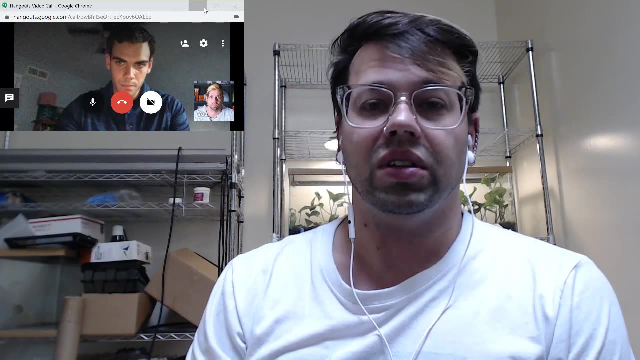 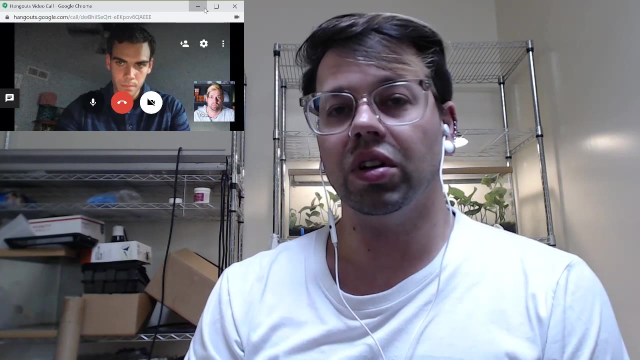 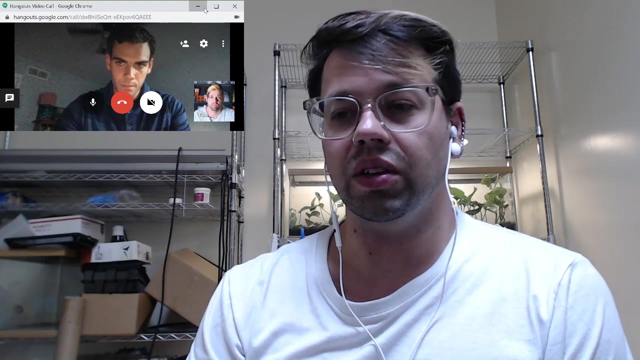 Are used to try To replicate humans. Now you have to understand that On a cellular level, The level of the immune system and metabolism And all these different things, These organisms are so much different than humans. So When people tell you that they've like 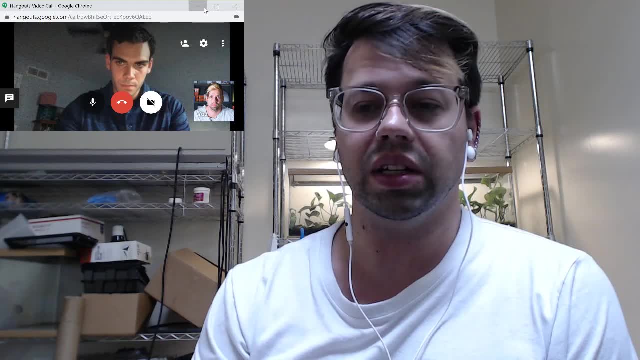 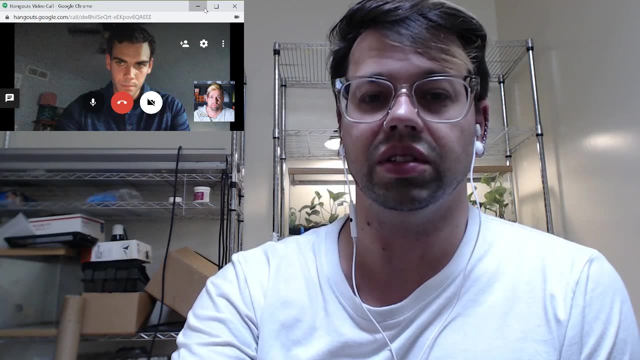 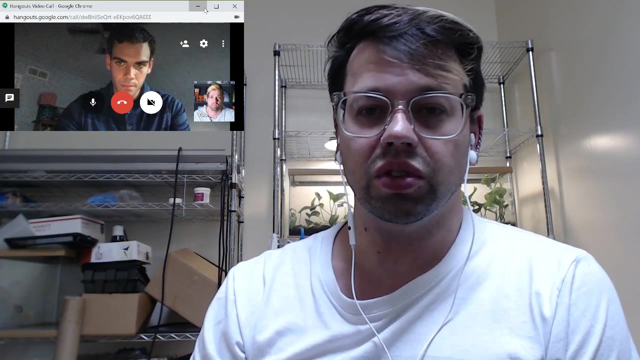 Cured autism or something in mice. Don't believe them at all. Right, Be very suspicious of this stuff, Because Cells are different, right. Like We have so many different cells And Different, We have a different immune system. 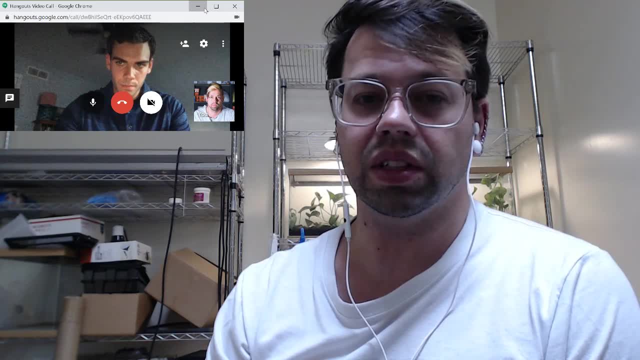 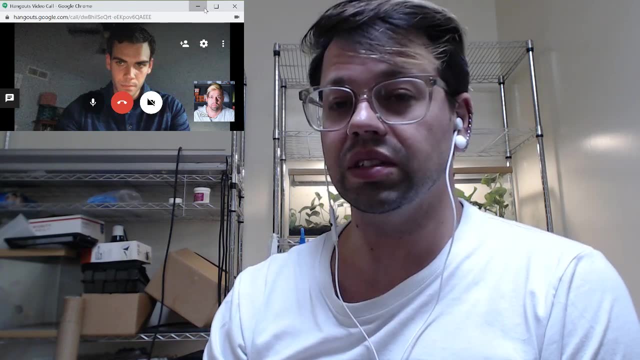 And we have Different metabolism And all these things Than all these other organisms. Is it a good starting point? Sure, But the chances that it translates Easily And directly To helping humans Is not good. It's generally not good. 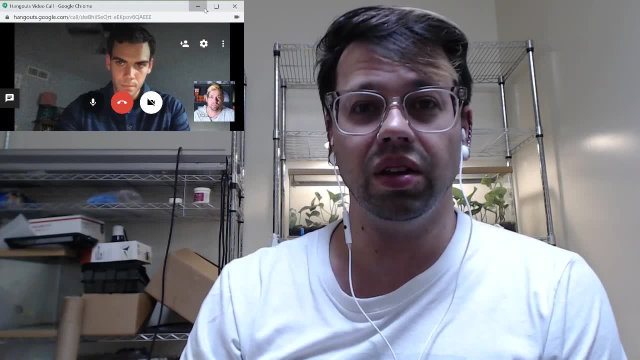 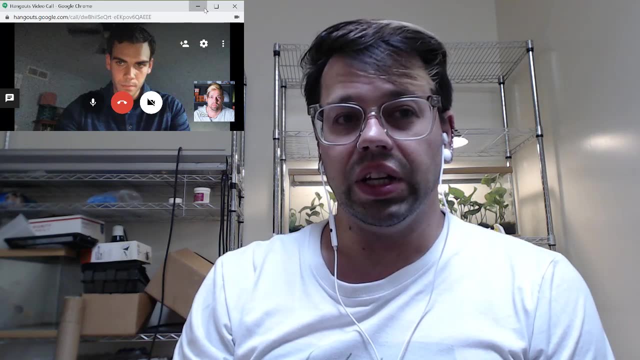 Right And we're not really allowed to experiment on humans. So We're left in a Very- Um, You know, Very- weird area Where we Scientists Kind of have to experiment on mice And Fruit flies and stuff. 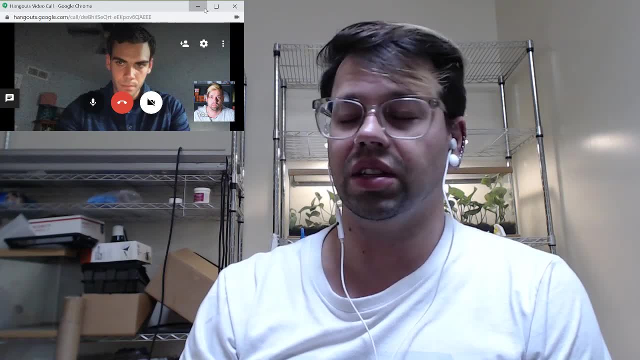 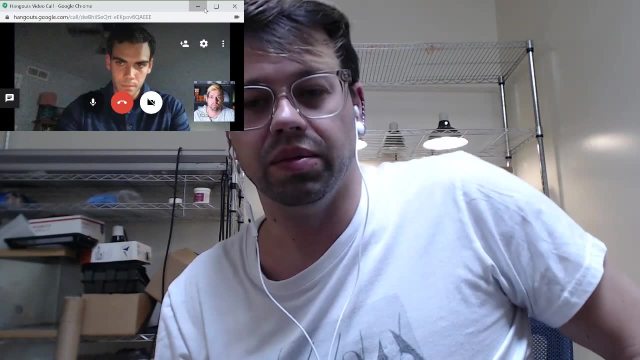 Um, I don't think we need to Experiment on fruit flies, But Don't Tell anybody. I said that Um Might piss off a few scientists out there, But I'm just saying, Like You see, some of these fruit fly research. 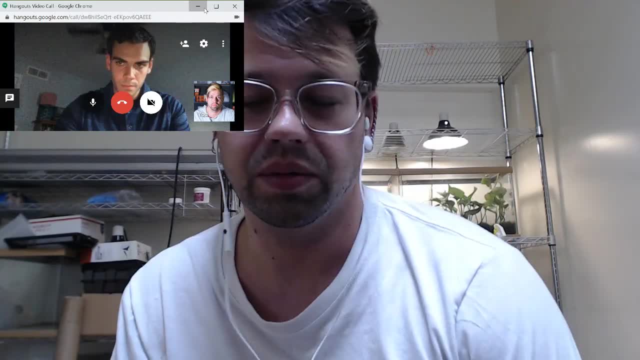 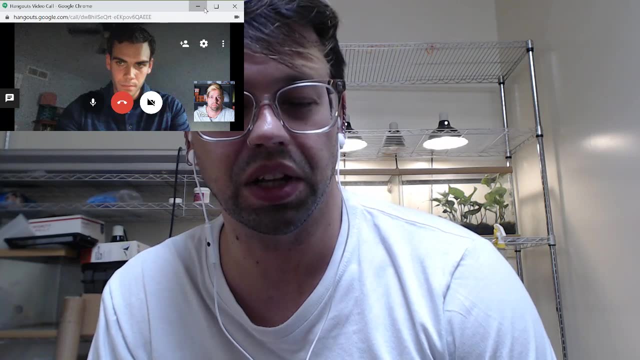 And they're like We got some Fruit- Fruit flies Drowning Out there. But I'm just saying Like We got some Fruit flies Drunk And then we tried to make them climb up a wall. 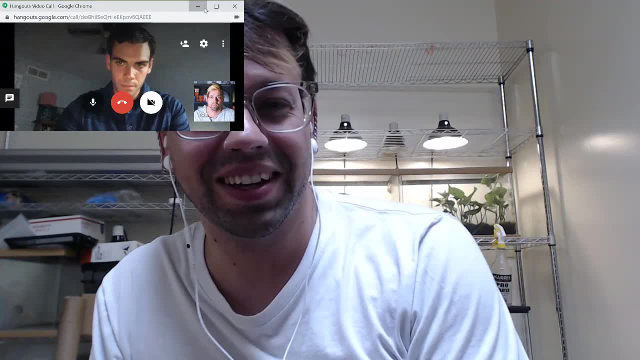 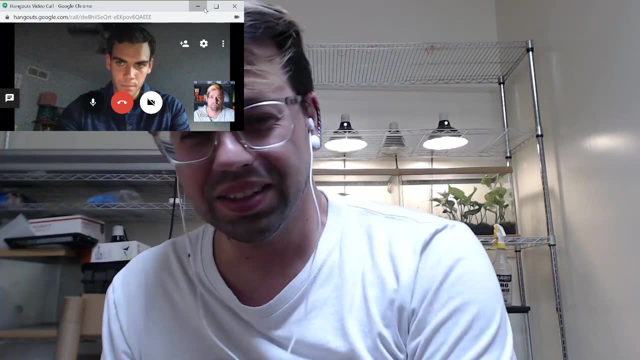 Or something, And you're like: Alright, You know, Like I kind of get it. You're trying to like Extrapolate that To humans And do science. But like You know How a fruit fly responds to alcohol. 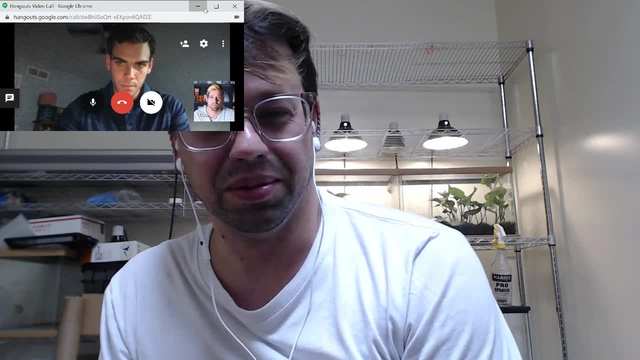 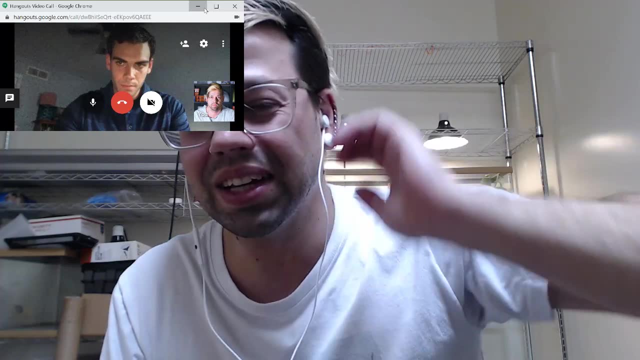 Is Probably Not Going to be Extremely Similar To how a human responds to alcohol. So, Uh, Maybe we could Figure out Something, Something else You can test Or work on, Or just Something in general. 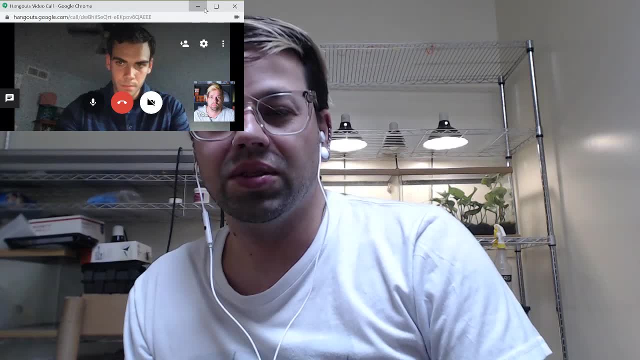 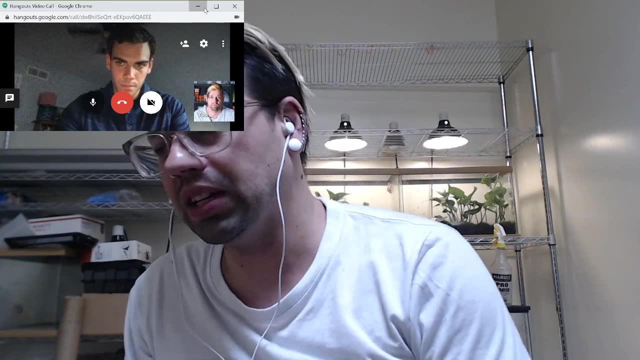 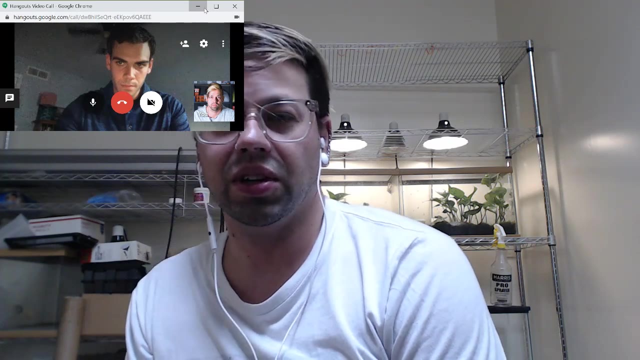 Um, So, You know, We all hear about DNA And all this different stuff And, uh, People say DNA Is made of A, T, C And G, Right, And We hear That, You know. 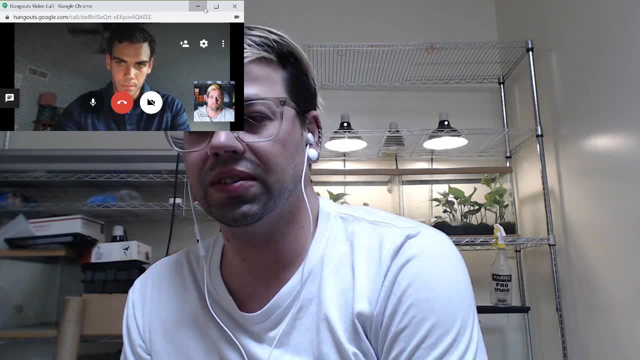 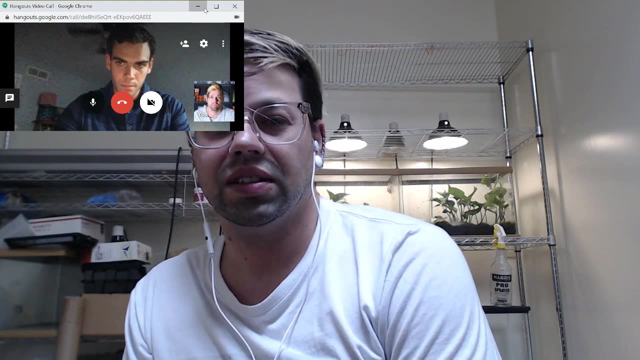 You got a cell And you got Cell wall And lipids Or proteins And I know These things Are like Hard to visualize And Understand, But What you have to Start to Understand Is that 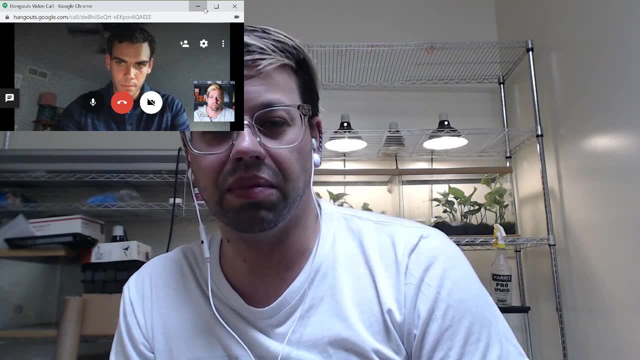 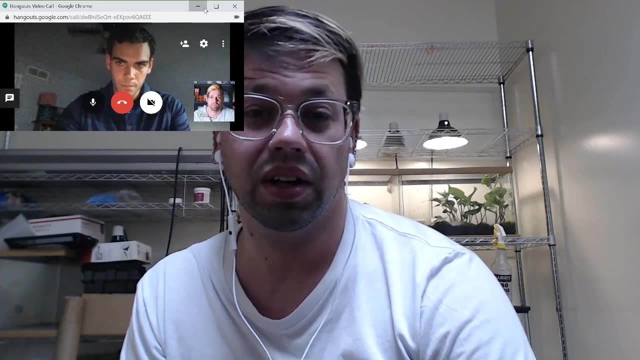 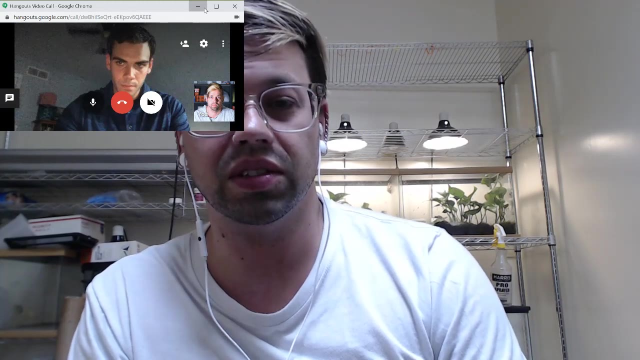 These, You know, Macromolecules, These Big molecules. They are Basically Composed Of Five Different Things, So Things In The Cells And Other Things Like Sulfur. 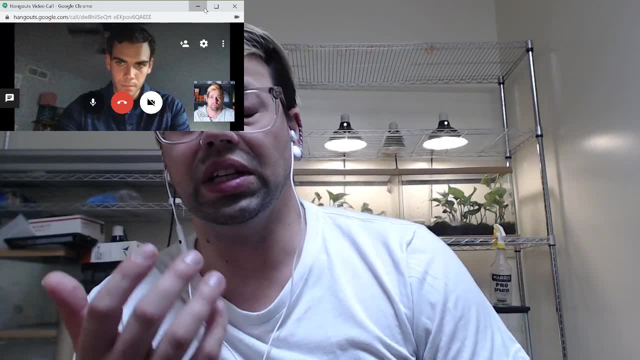 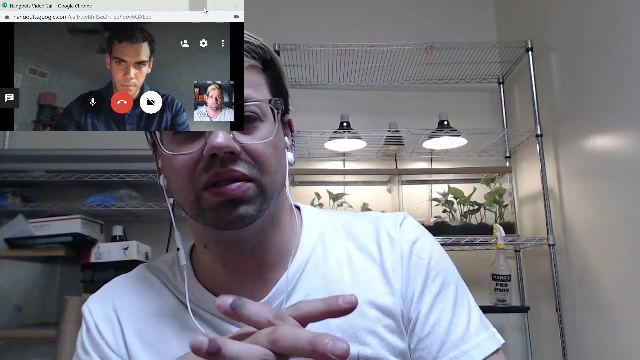 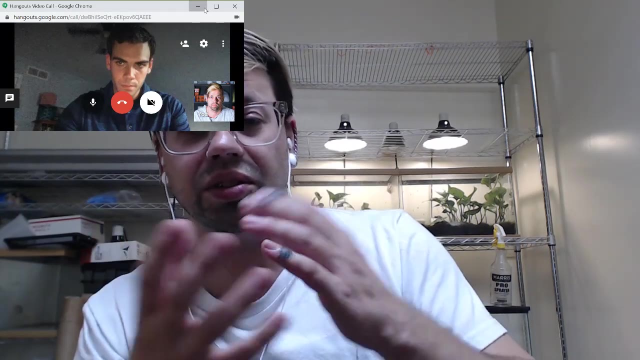 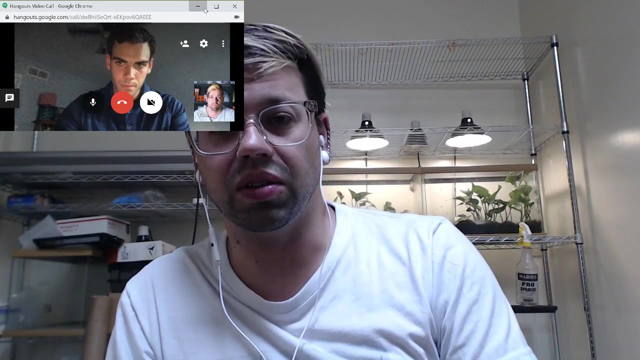 And Whatever You know That Are Also Involved. But These Are The Five Major Things. So, When You Think About DNA, When You Think About Things, 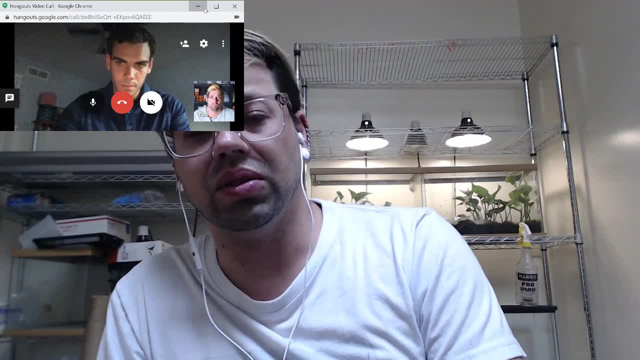 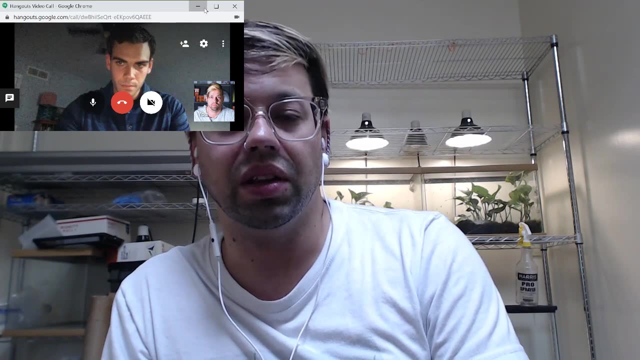 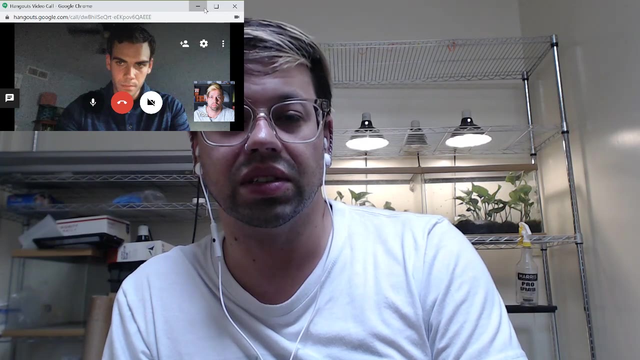 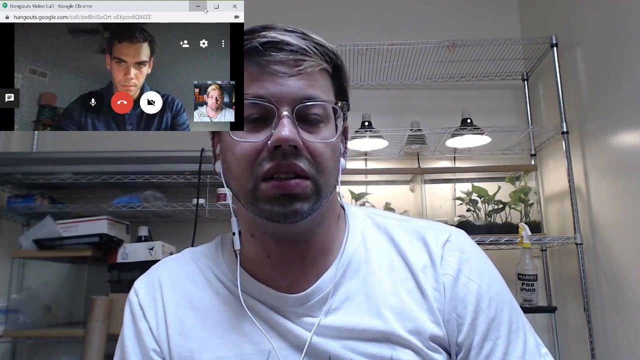 Work Right, Like Carbon, You Know, Carbon Is A Fairly Neutral Atom, And By Neutral You Mean That The Charge That It Has Based On 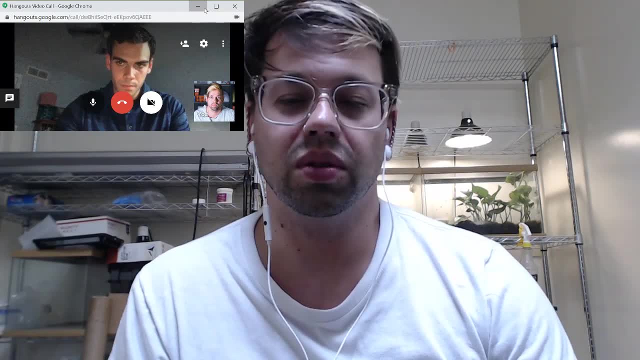 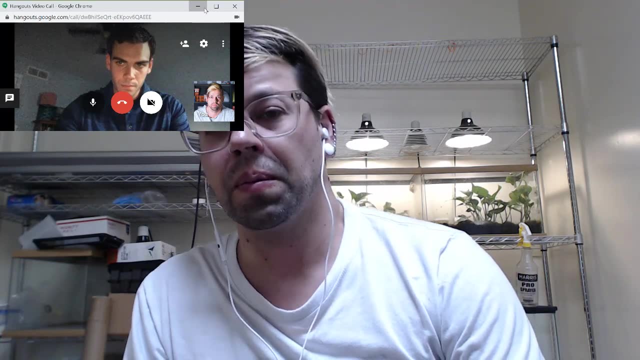 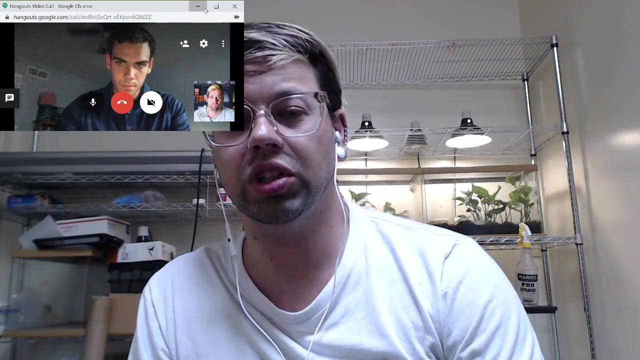 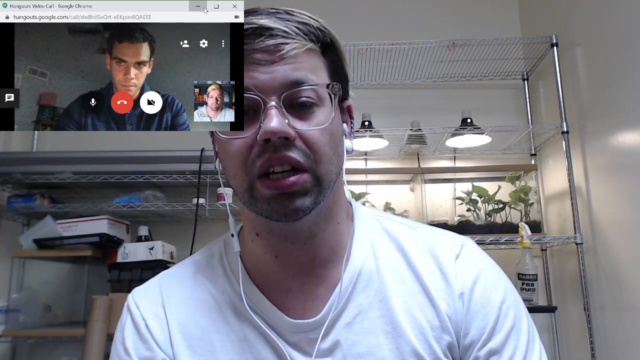 The Electrons And Its Positive, Or Have A Positive Or Negative Charge, Much At All. Certain Situations When You Have Like A Carbon Ring You. 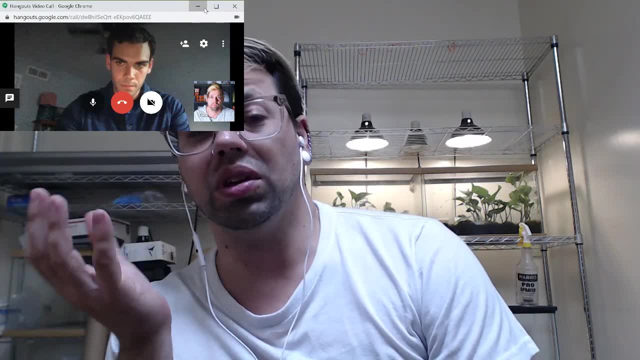 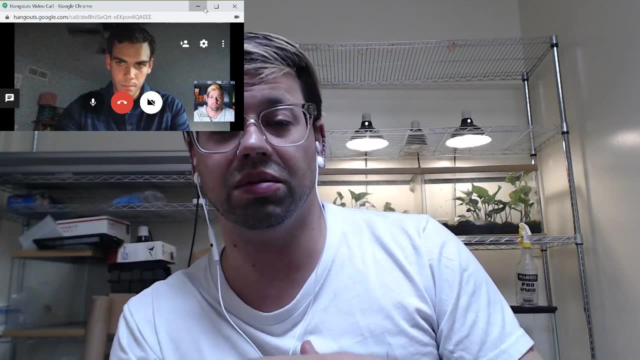 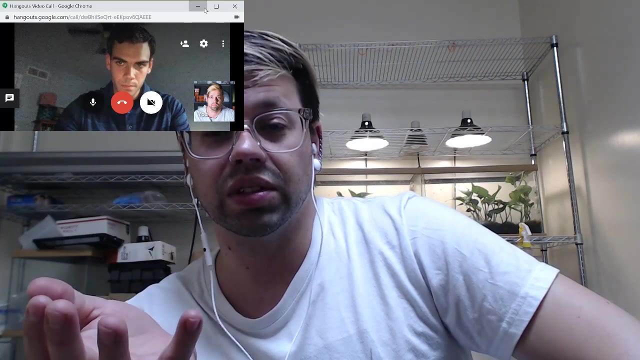 Can Start To See Weird, Strange Effects. But The Number Of These Atoms In The Arrangement Of These Atoms In The DNA And Protein? 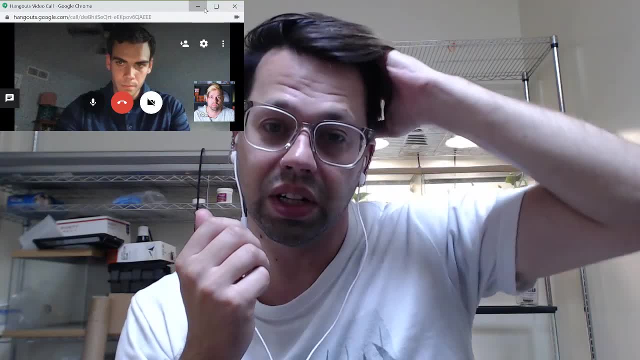 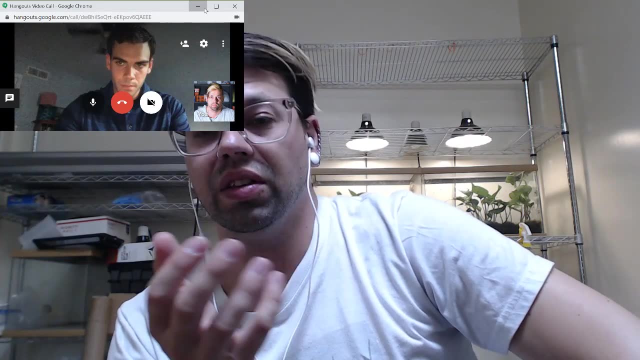 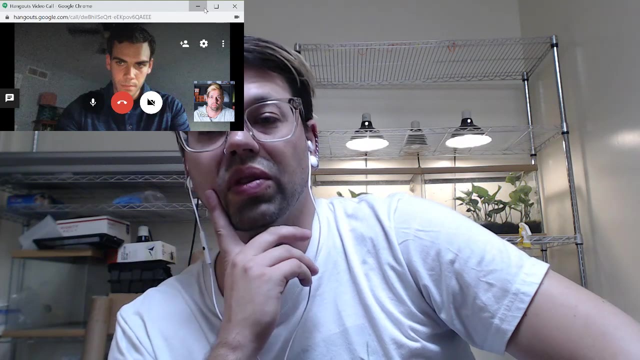 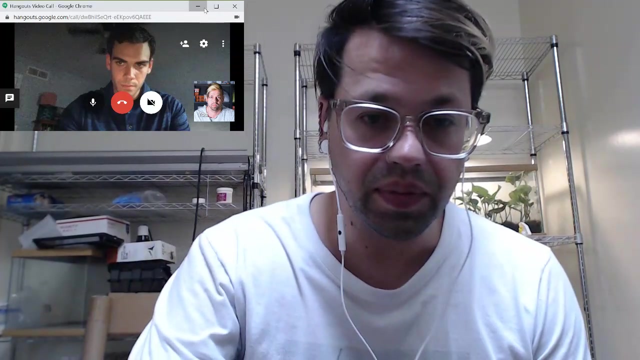 That Have Specific Characteristics, Like A Positive Or Negative Charge, And These Positive In. They Have Different Forces, Different Abilities To Do Different Things Right. So 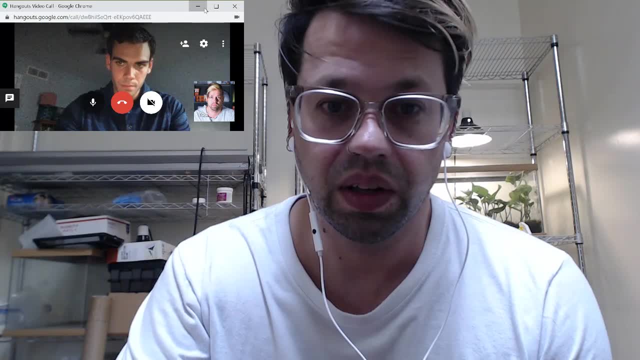 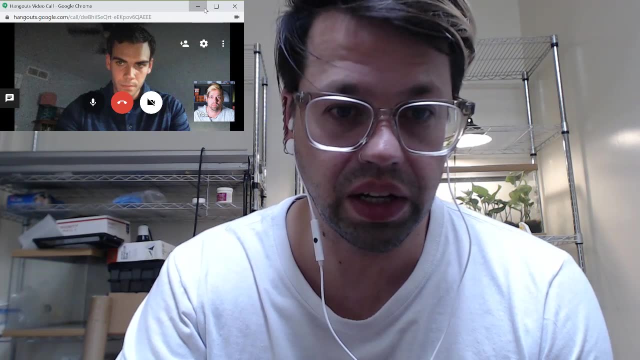 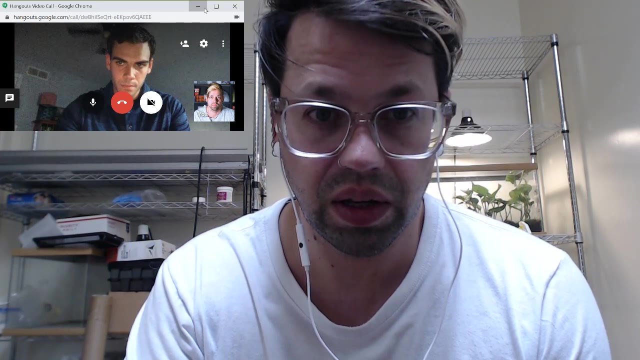 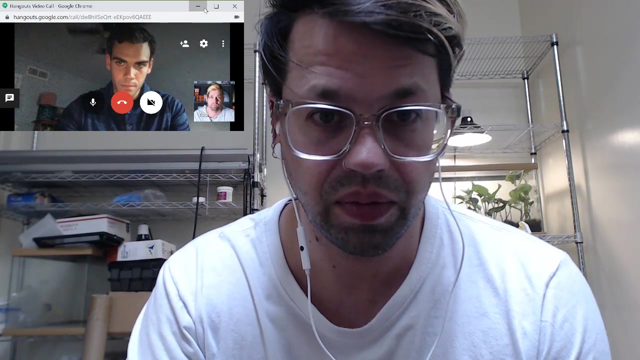 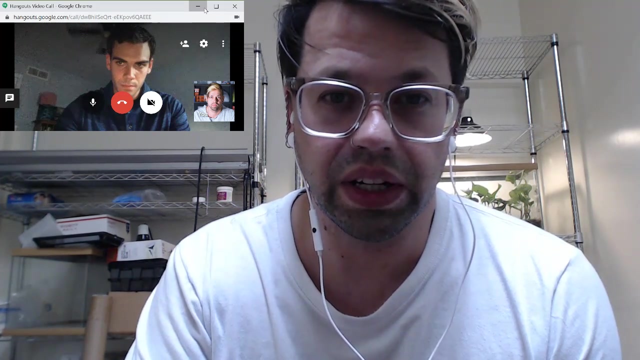 For Instance. If We Look At DNA, Let Me See If I Could Pull Up A Picture I Know Almost. So DNA Is Composed Of. 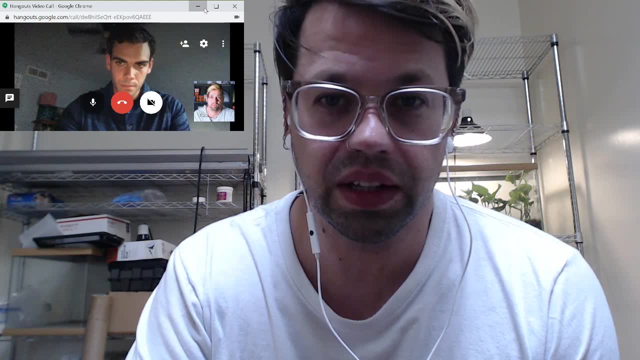 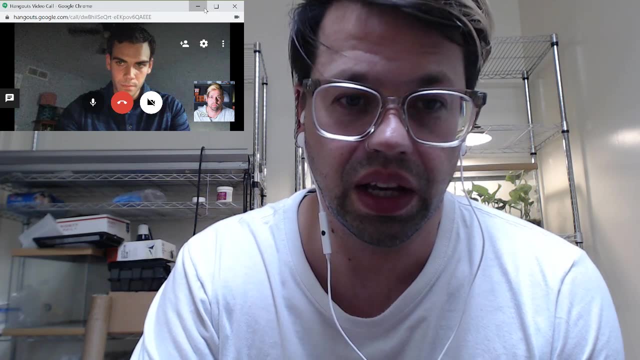 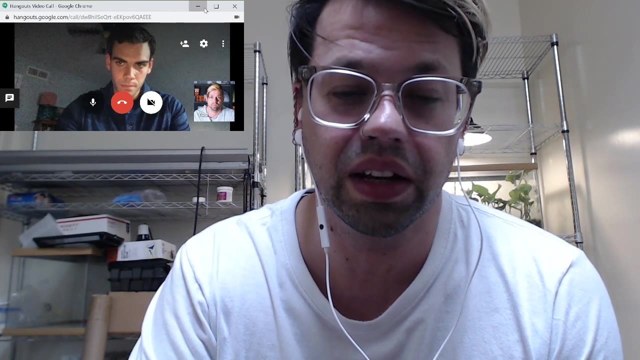 Two Strands Right, And These Two Strands Are. They Interact With Each Other, And An Interaction That Is Based On The Fact That Certain 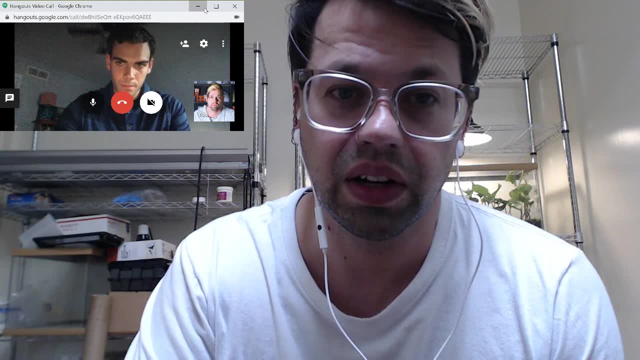 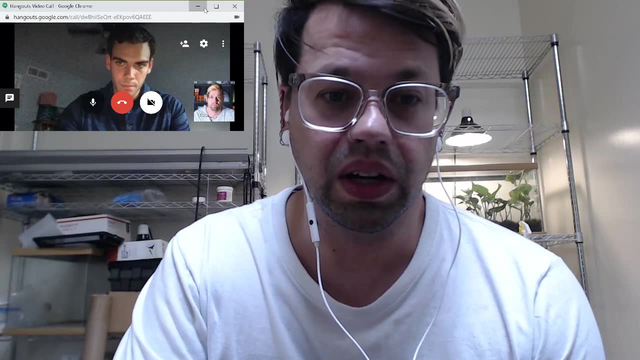 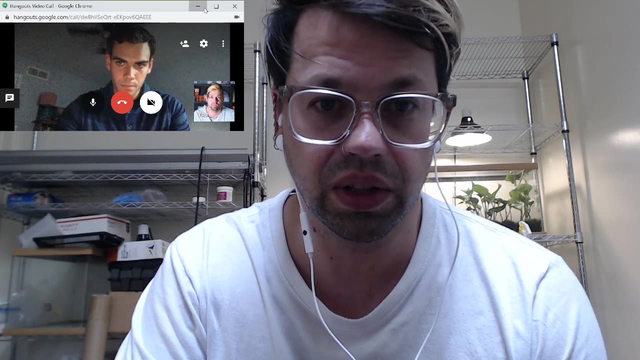 Molecules Have Different Charges, And Those Different Charges Allow The Molecules To Interact, Right. So Let's See Where Is I Thought I Had It. 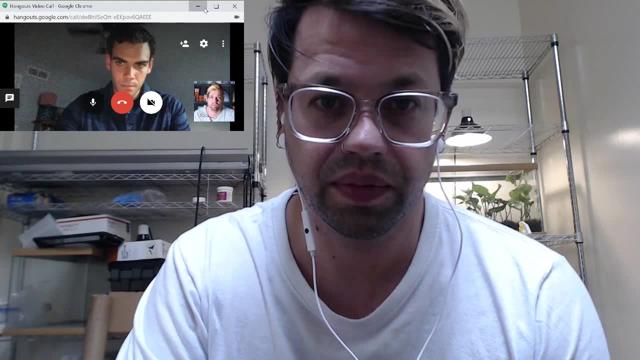 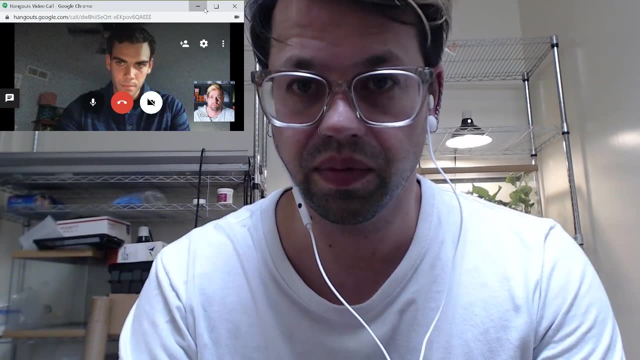 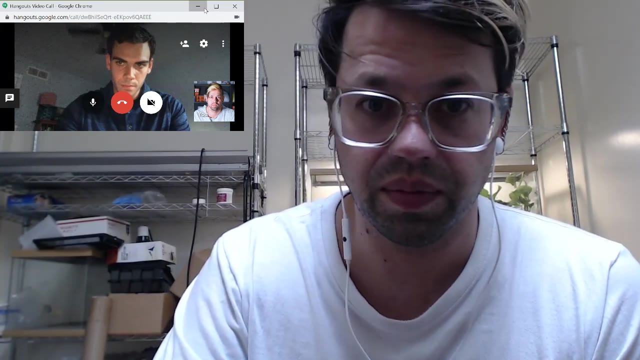 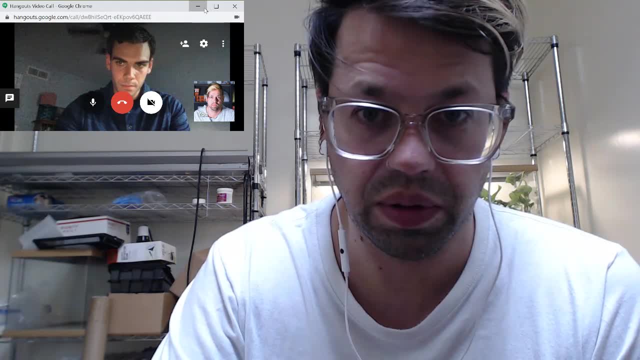 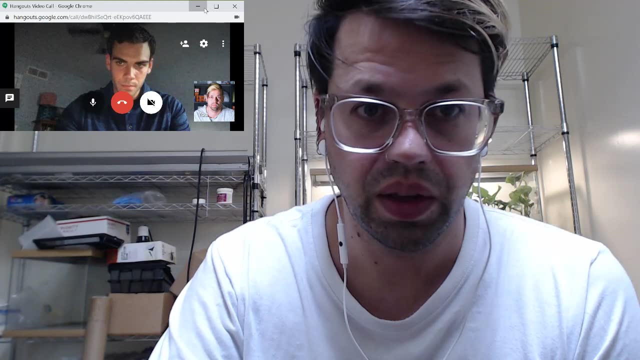 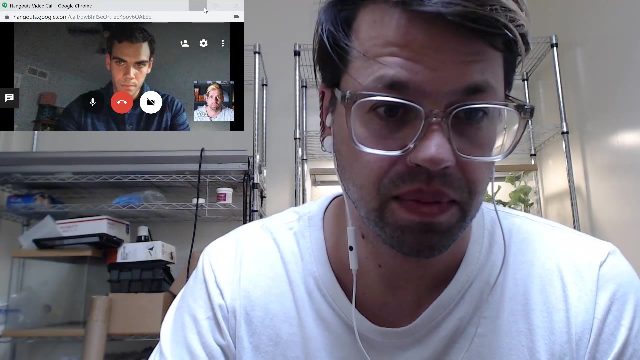 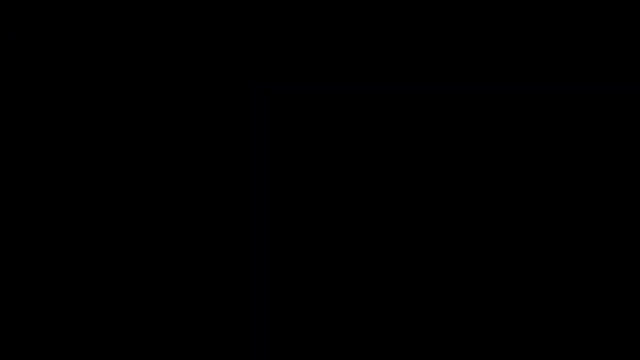 Is, Maybe I'll. Oh, Here We Go, All Right. All Right, Let Me Share This On The Video So You All Can See It. So 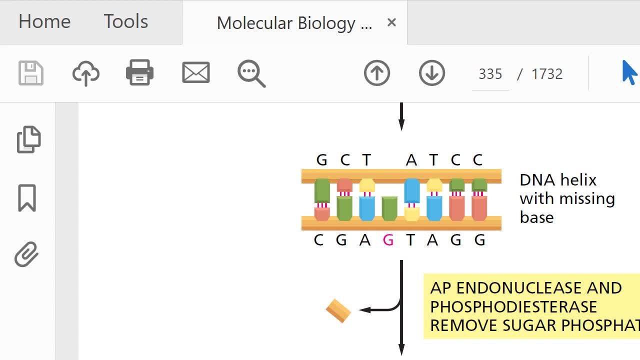 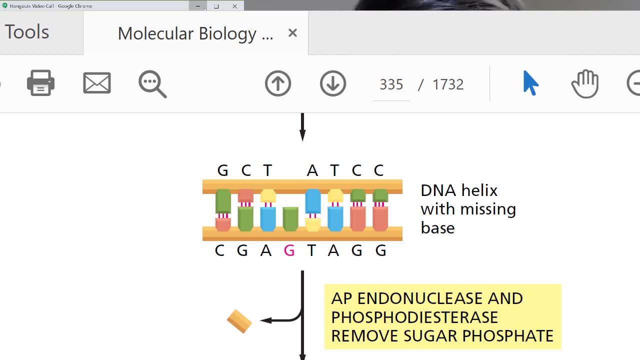 All Right, Here We Go. So Here's A Picture Of DNA Right Here, Right And You Have. DNA Has Two Different Strands, And 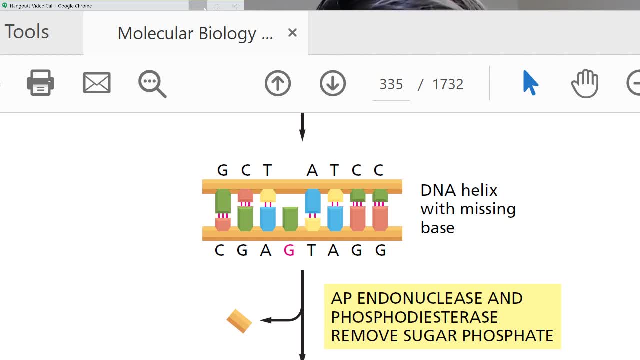 These Strands Of DNA. You Could See These Two, You Know, In The Early Hot Springs On Earth Or Wherever These Molecules Came. 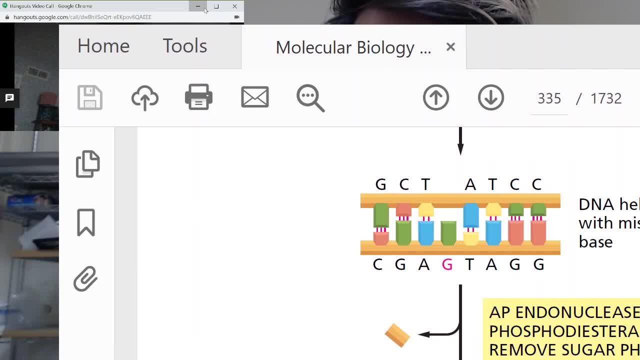 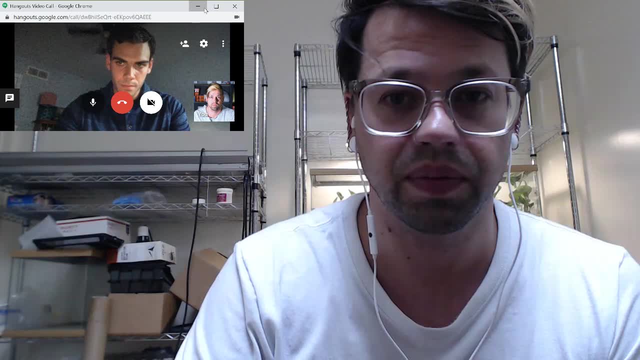 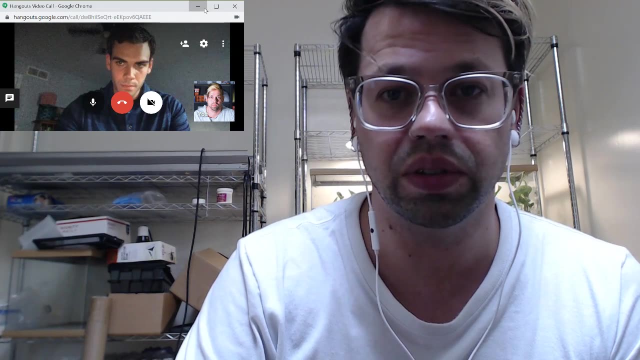 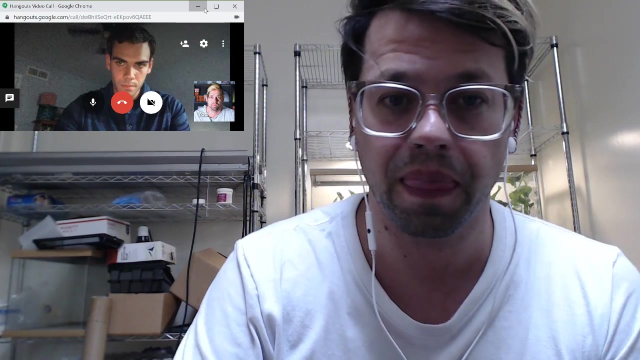 Together Because They Were Able To Interact Positive And Negative Charges And Things Like That And Bids, And How All Everything Works Is It Uses. 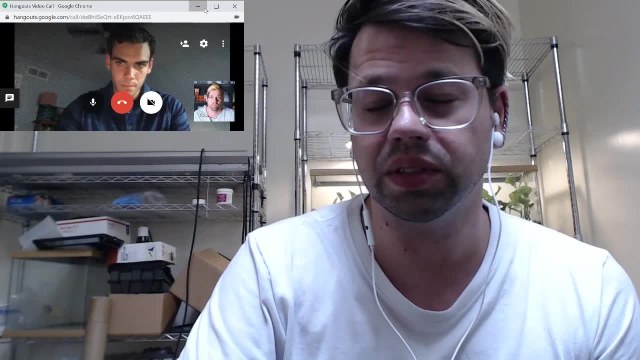 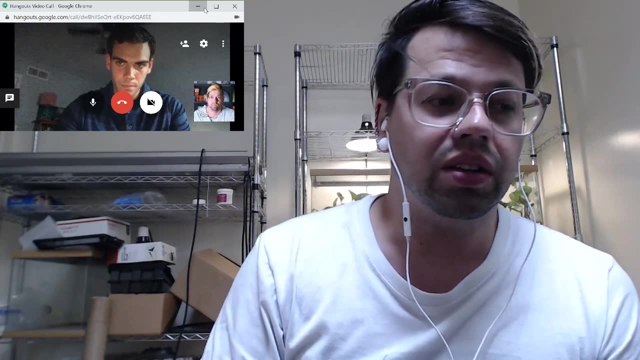 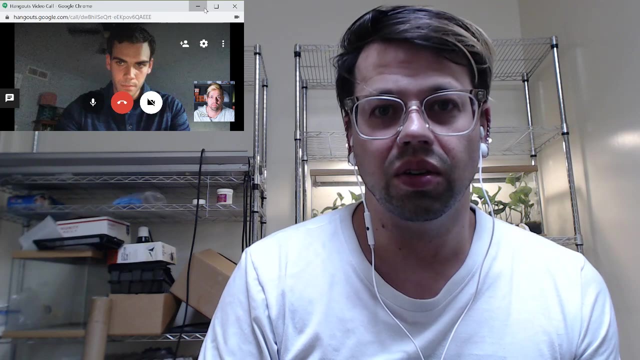 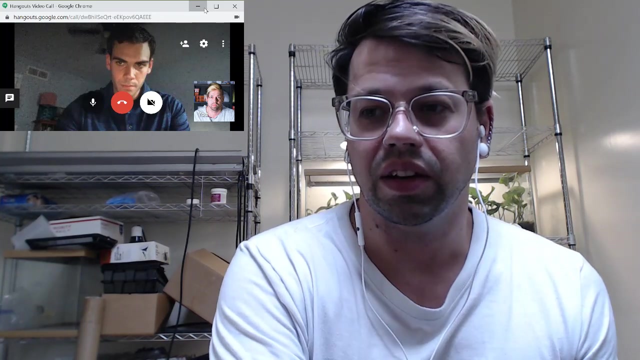 These Positive, Negative And Other Charges To Do Stuff Right. So Cells Specifically, Overall They Even Have A Voltage Right Now There Is A Difference In. 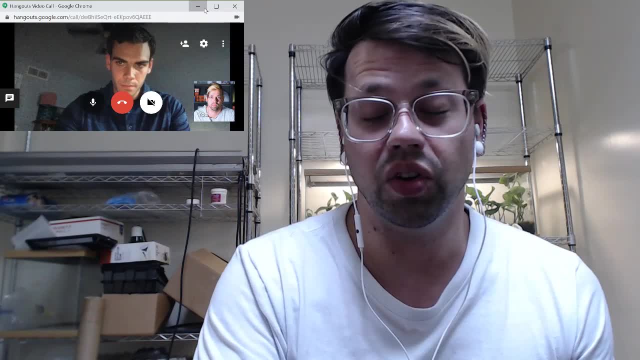 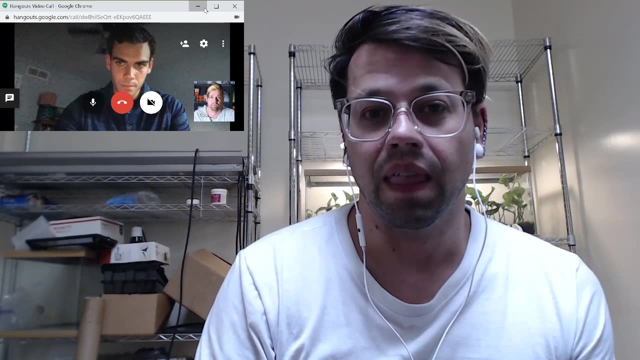 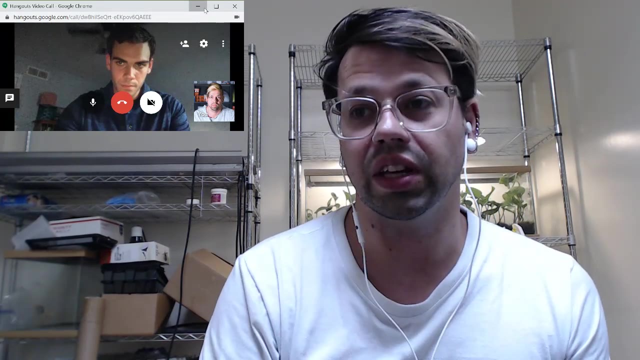 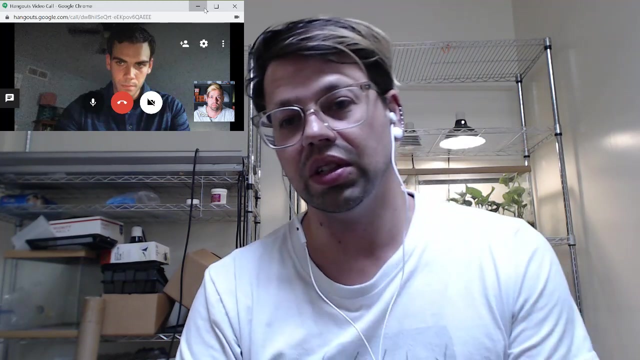 Voltage Potential Based On The Amount Of Different Ions That Are Inside Versus Outside The Cell Right, Because These Cells, They Also Use These Positive 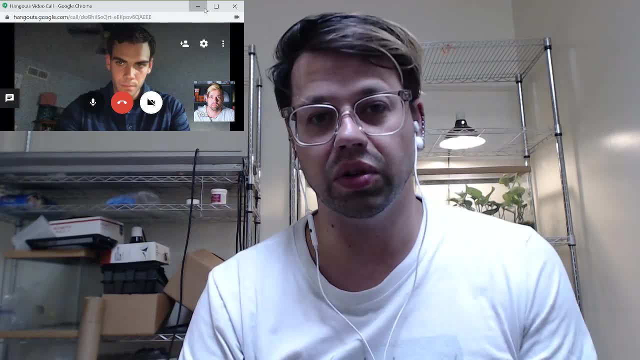 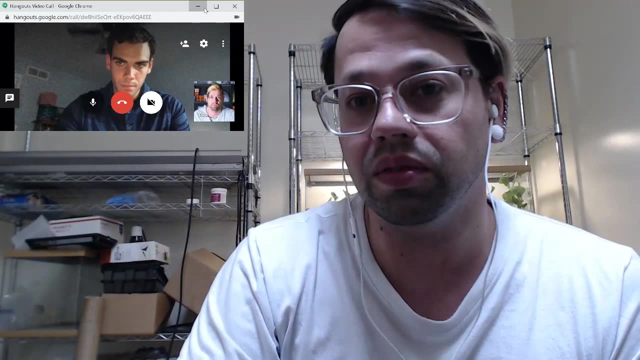 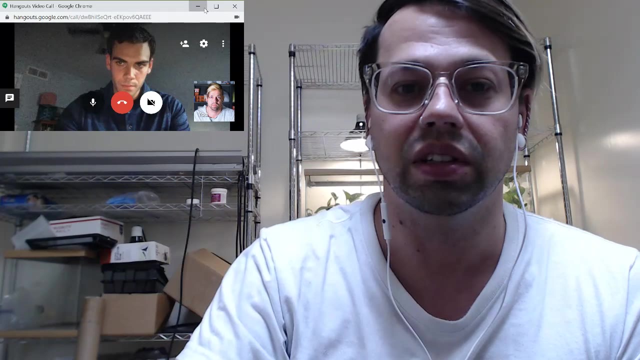 Charges That Help Our, Our Nerves And Neurons Communicate Through Our Whole Body. So, Like On The Most Primitive Level, We're All Just A. 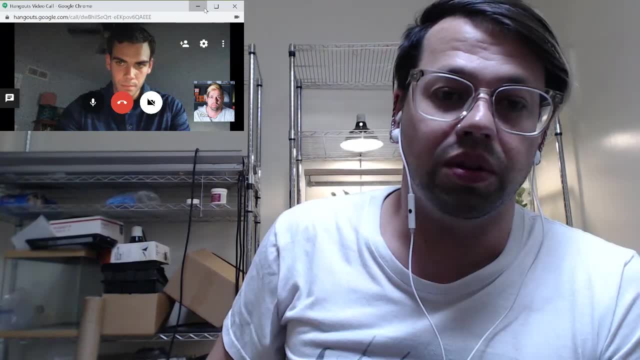 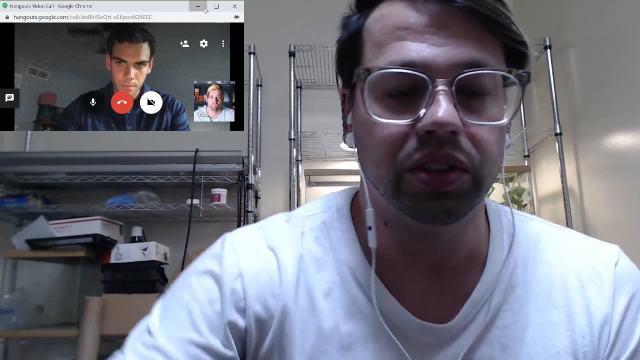 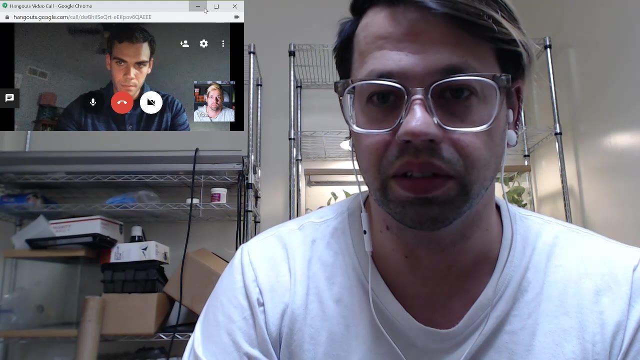 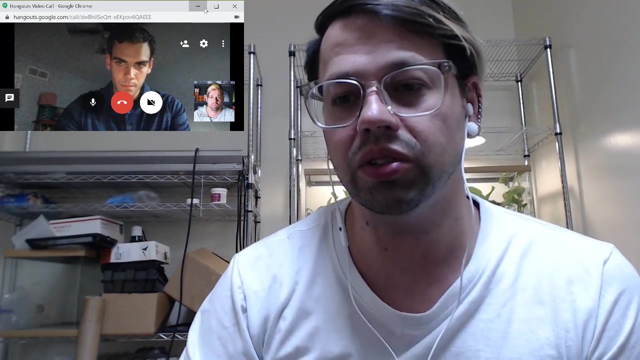 Bunch Of Neutral, Positive And Any Questions. Anybody Got Questions? Let Us Know. Me And Justin Are Here To Answer Your Questions. I Know It's. 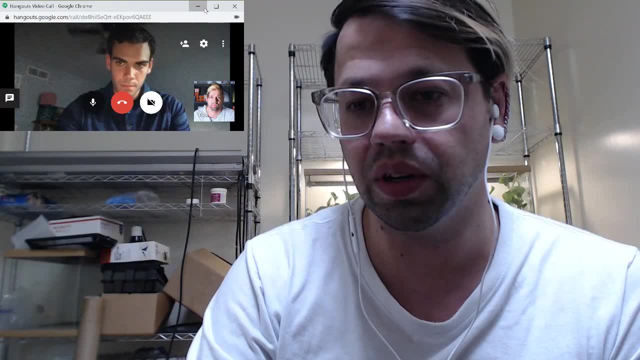 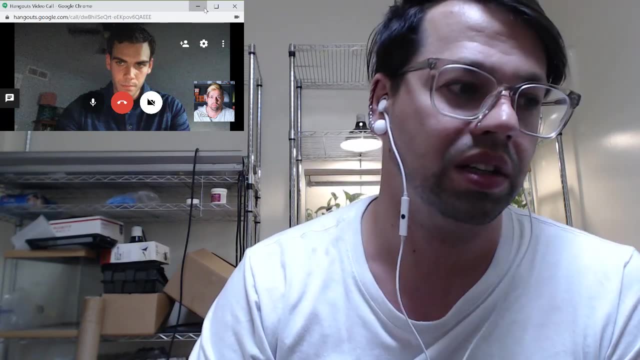 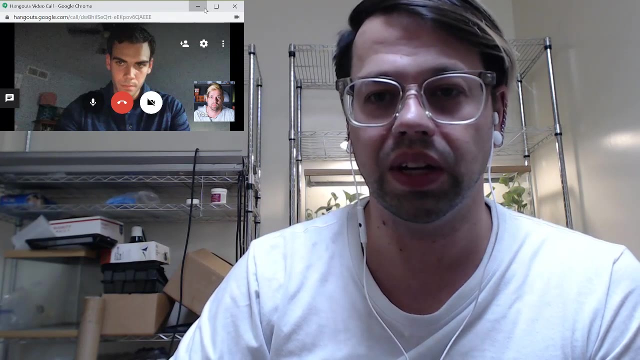 Crazy, Don't, Don't, Freak Out. You Know Like. I Know What's Going On. What's D N A, What's A Protein? Just Read Molecular. 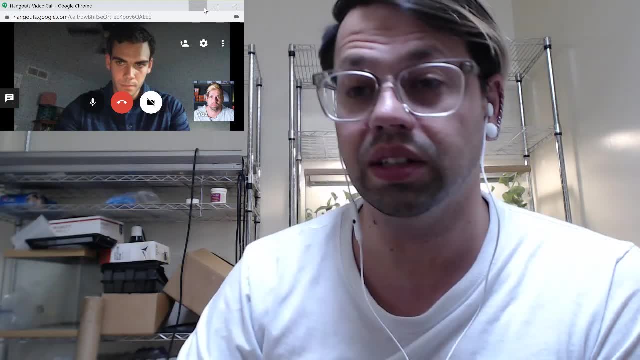 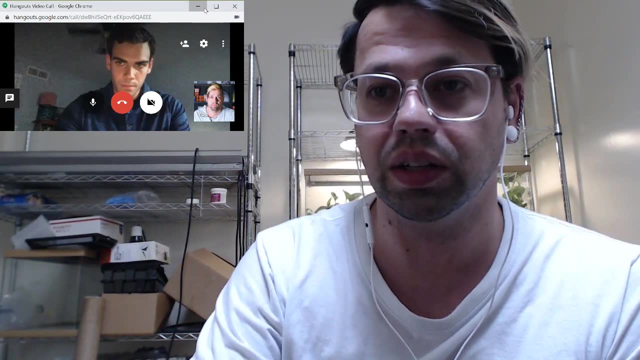 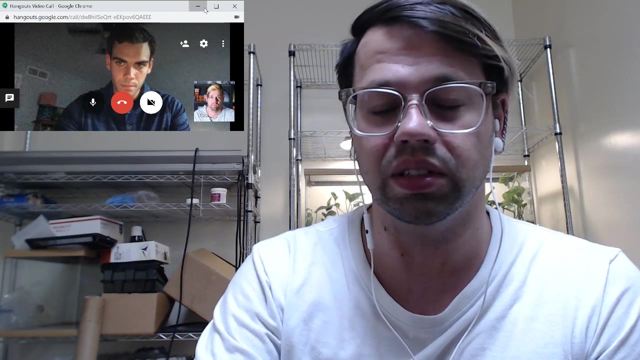 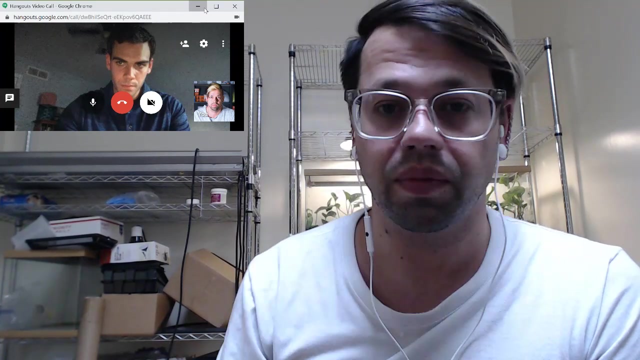 Biology, The Cell Find Time, Read, Some Of It, Start To Get, Take This Information. It's All These Different Terminologies And All These Different Things. 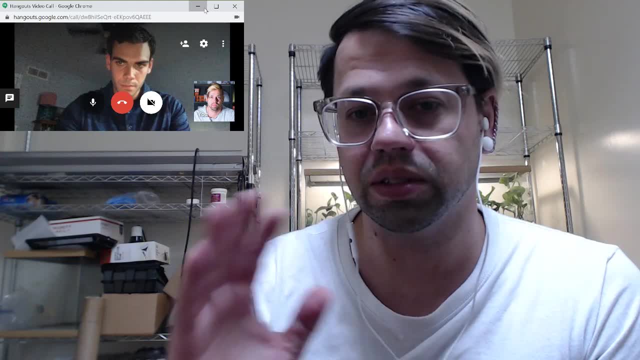 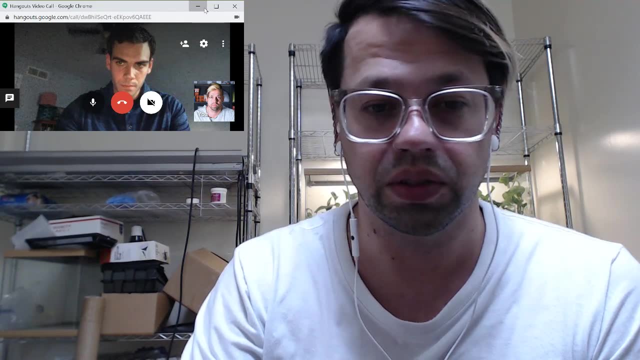 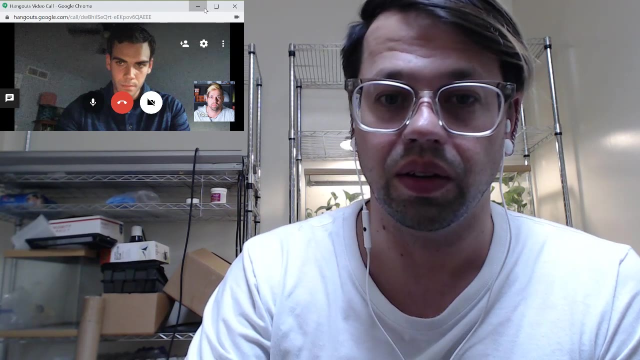 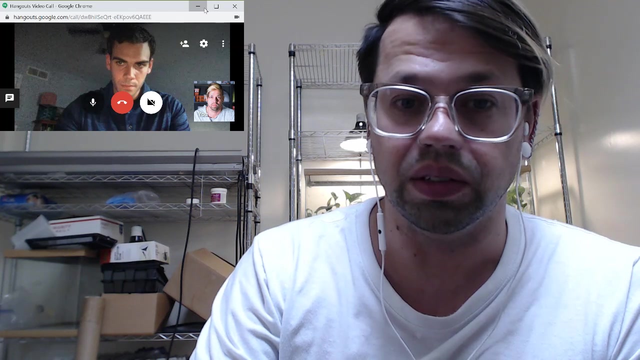 It's Just Like Learning A Whole New Language, So Don't Worry Too Much If You Don't Understand And Feel So. Cells, So The Two. 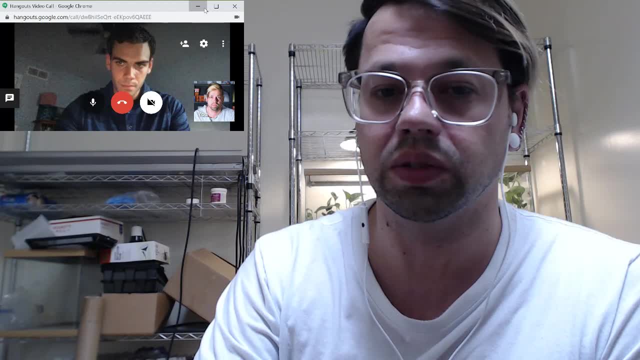 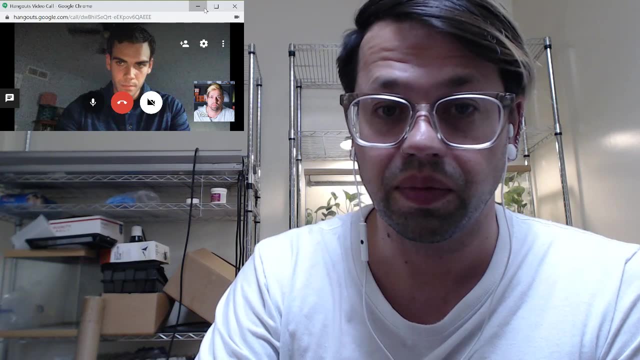 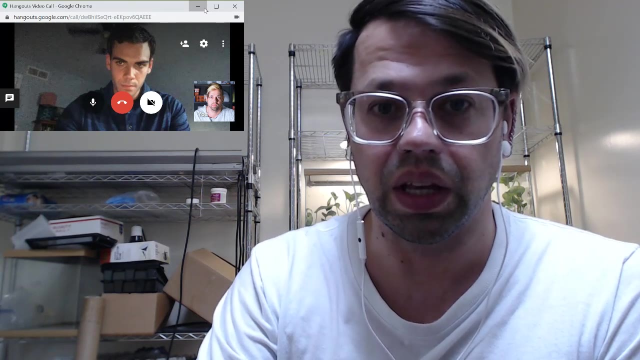 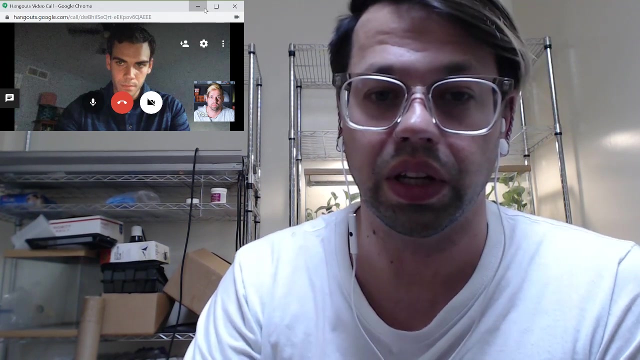 Experiments We're Going To Do This Week That Will Help Us Next Week When We Start To Get Into Actually Working With Cells In Your 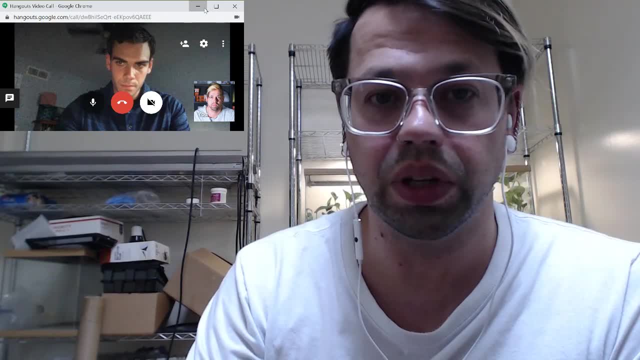 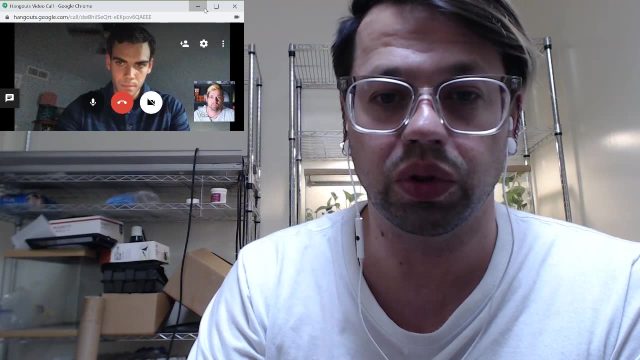 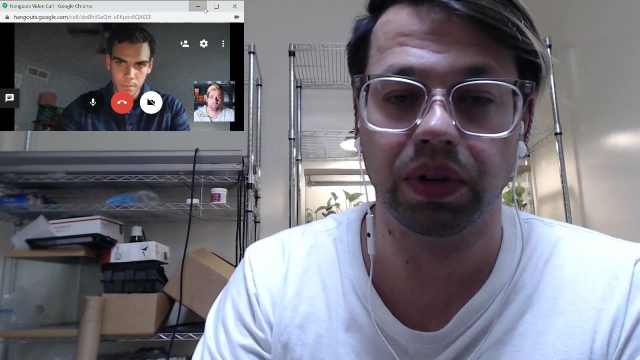 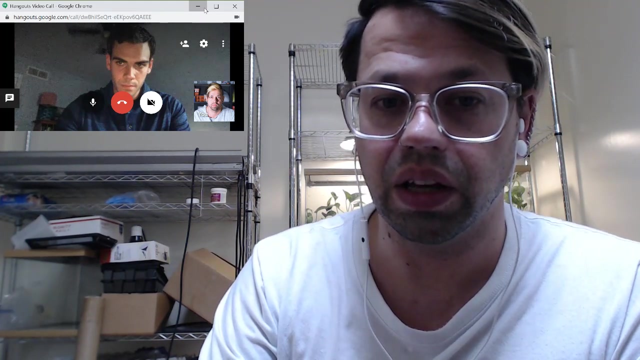 Molecular Biology Career. Now, If You Go To Week One, We Have The Experiments And We Should Have Tutorials With Pictures And Directions Mess Around. 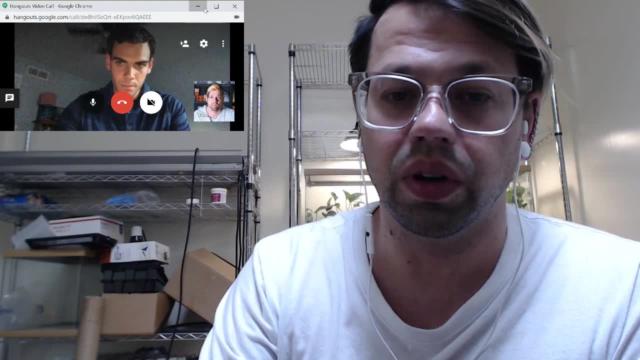 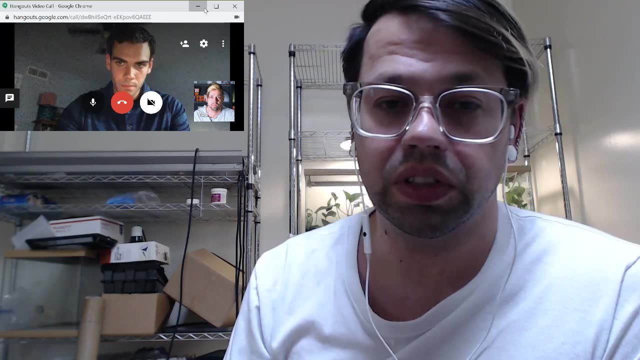 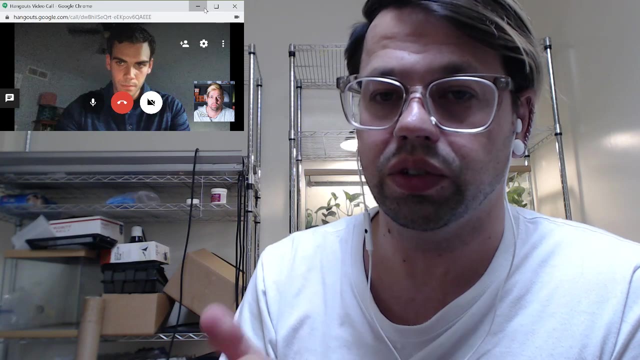 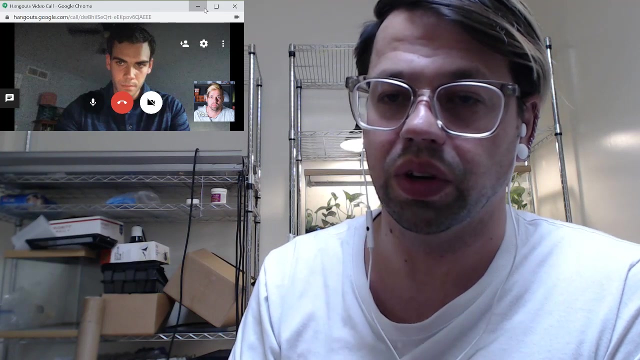 With Your And You Know. Understand That A Pipette Is, You Know, Semi Precision Scientific Instrument. So Be Gentle With It Like Try To Get. 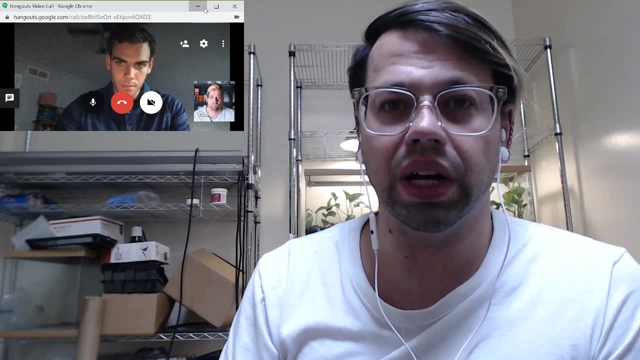 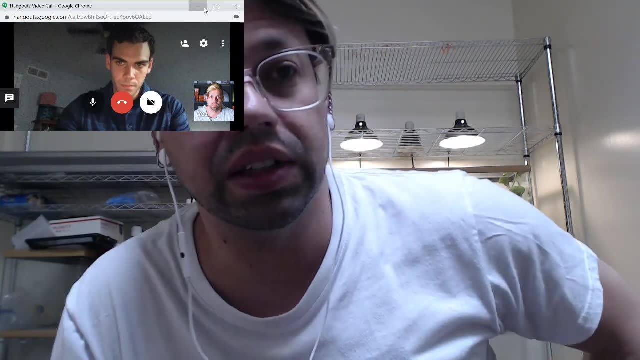 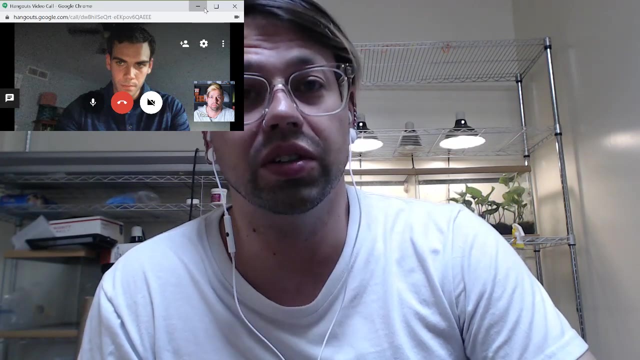 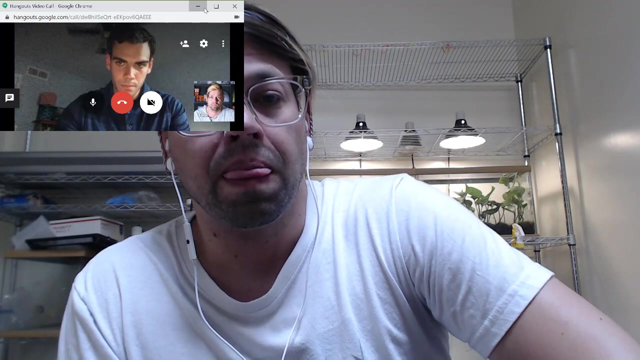 A Feeling For It. Don't Try To Learn. All These Things Are Not The Trials That You Can Have To Learn All About Your Life. 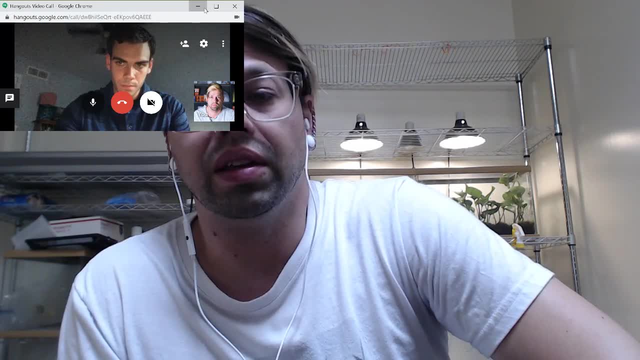 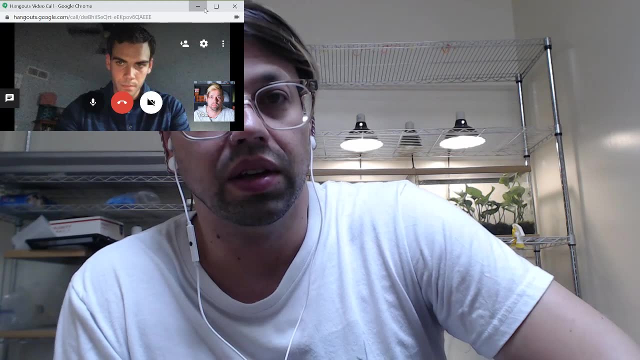 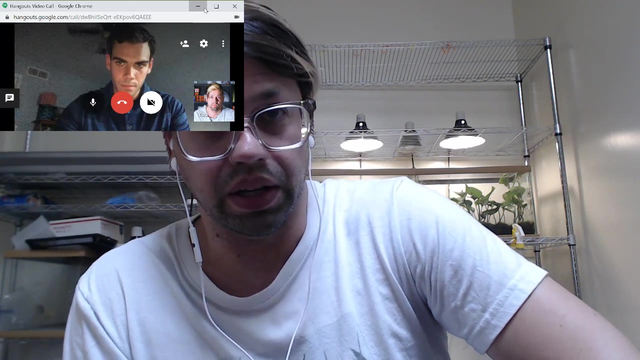 Well Know How To Learn How To Play The Guitar, And only way you're really going to learn how to play the guitar, or become good at playing the guitar, is by actually, you know, picking it up and playing it, And it's going to take a little bit. 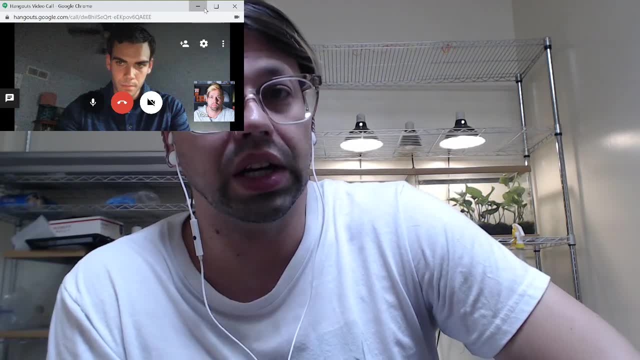 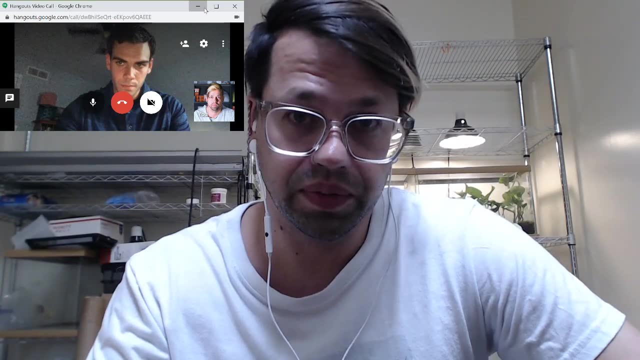 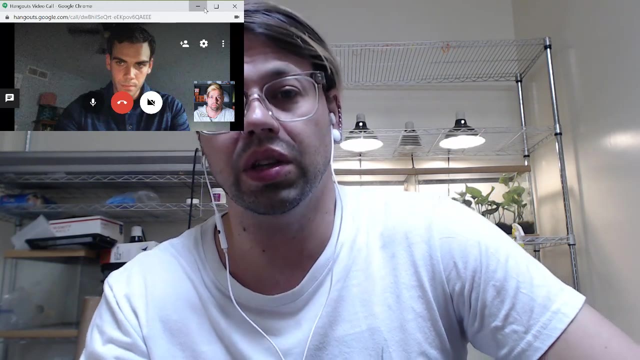 of time, But over time you're going to start to become good at it And you're going to have experience with it And you're going to be fine. So this week, first thing you're going to do is learn how to pipette, And the other thing you're going to do is learn how to use a scale. 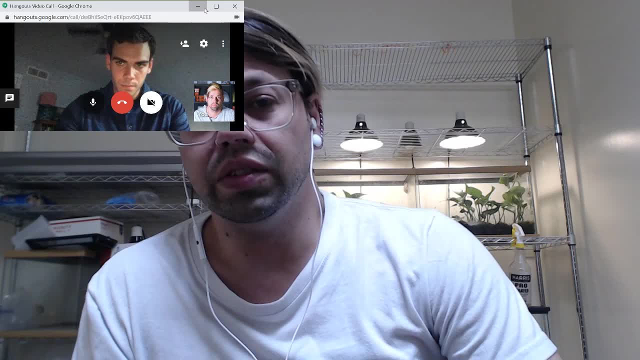 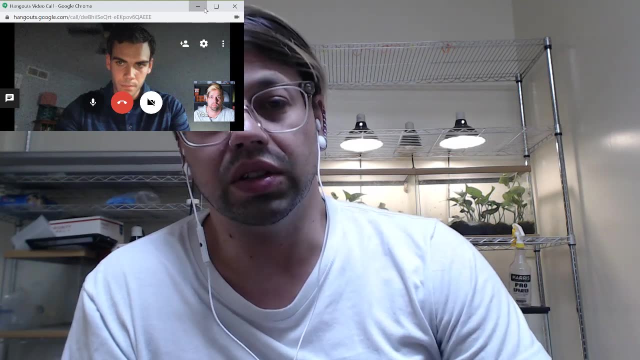 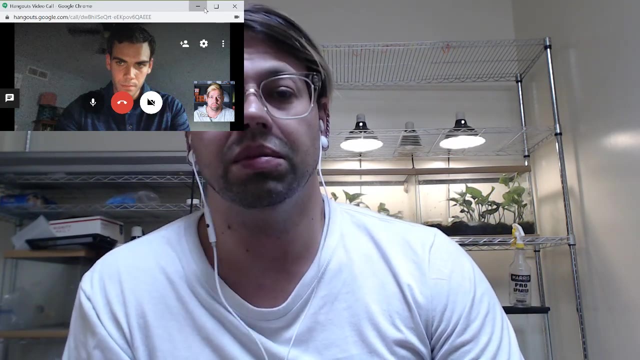 Scales are, you know, generally pretty easy, simple to get to get a hold of, get a grasp on, But still, it's just you know, helps you understand what you can do, avoid common mistakes and pitfalls that you might not have thought about. 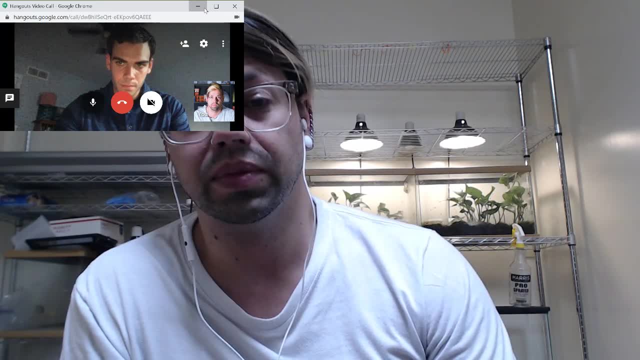 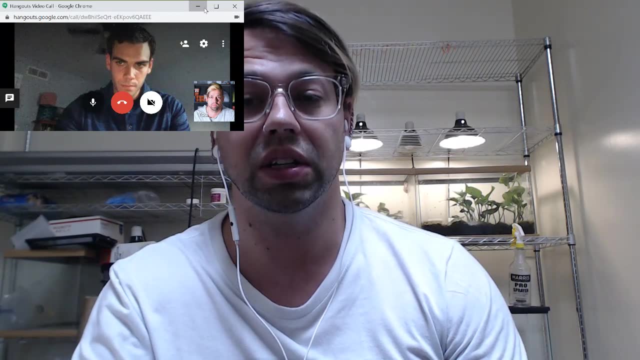 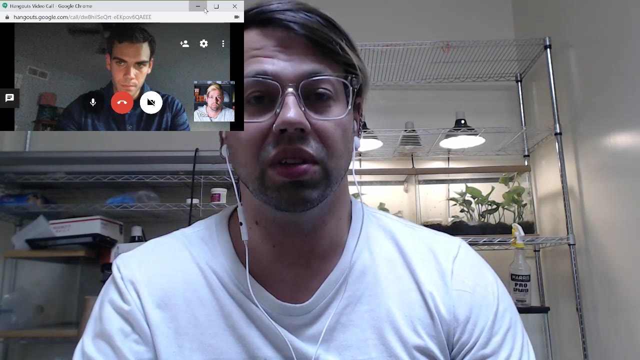 If you haven't really used a scale all the time, just so that you can do the future experiments, because in future experiments you're going to have to measure out stuff and mix stuff and things like that. It's something you'll always use for the rest of your life and the rest of your career. 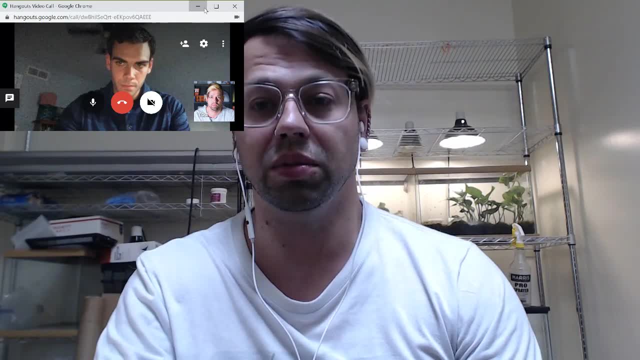 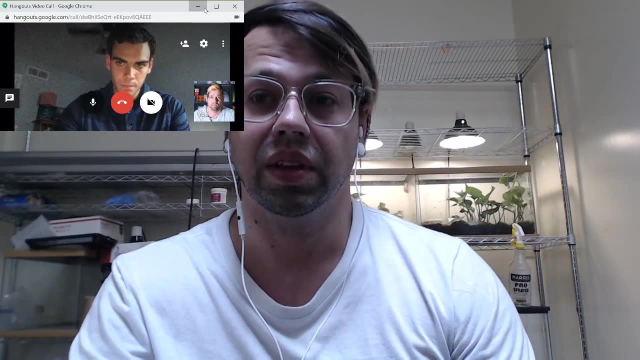 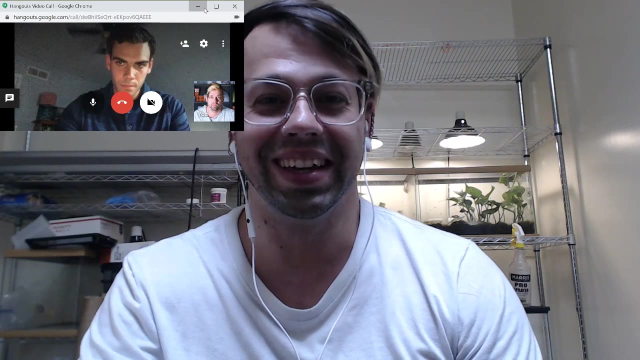 in molecular biology. You know I use a scale almost every day. I'm sure Justin does also. Yeah, Yeah, maybe we can hear you, Justin, I don't, I can hear you. I don't know if they can. 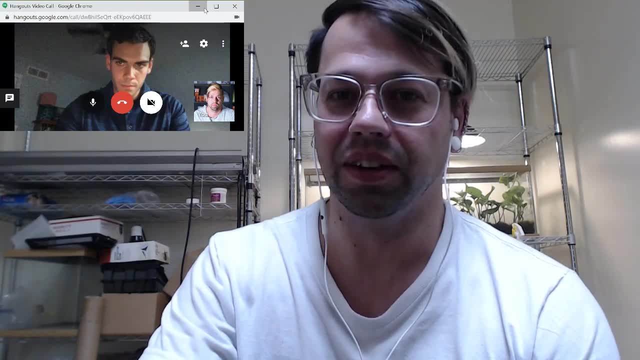 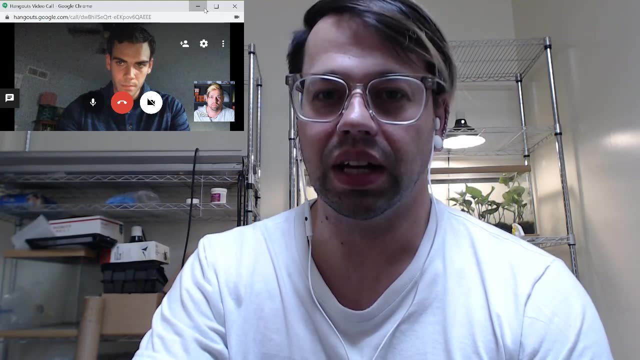 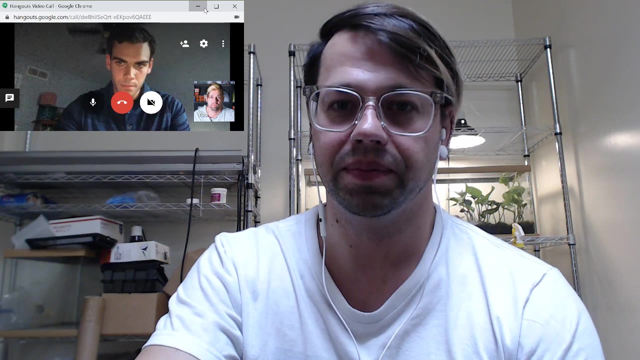 But we'll figure that out next time, Don't worry, We're going to make sure that I don't. yeah, I don't know if we'll have two instructors on every video, but we'll figure it out. It'll be all good. I just wanted to introduce everybody to Justin. I'm going to show you a little. 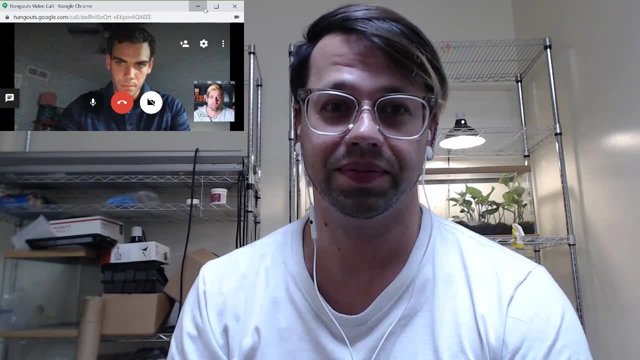 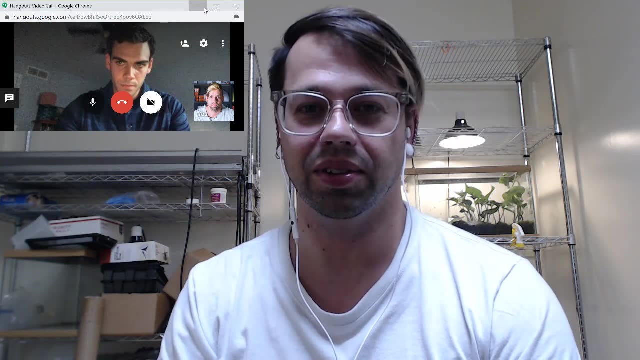 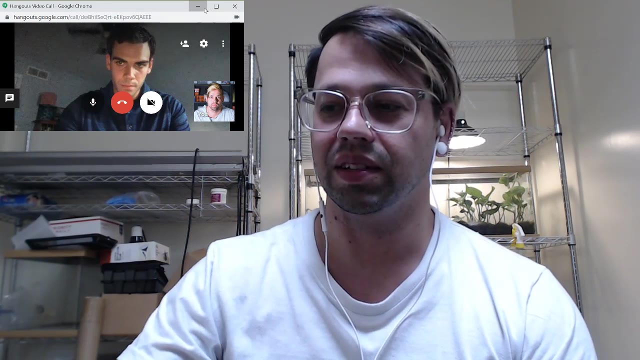 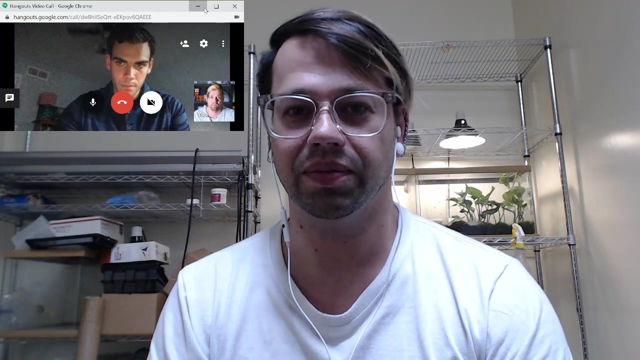 bit of Justin. I guess you can only see his picture kind of there, But I'm sure you could find him online somewhere on like Facebook or LinkedIn. Are you on some social media, Justin? Yeah, so he's on Twitter, Instagram and all the usuals. So find him there and connect with him.